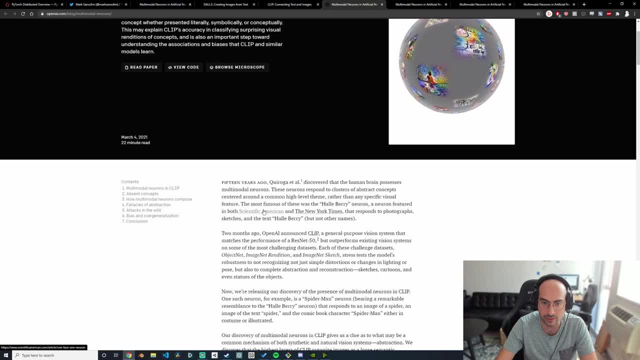 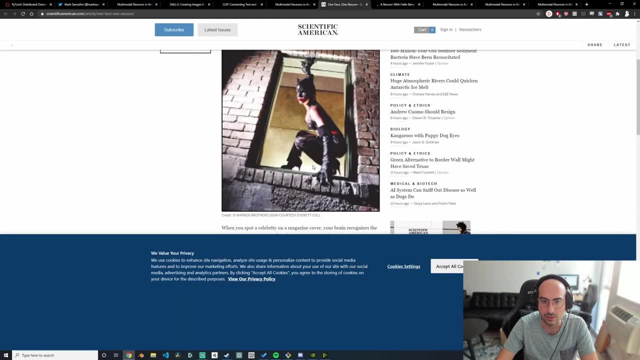 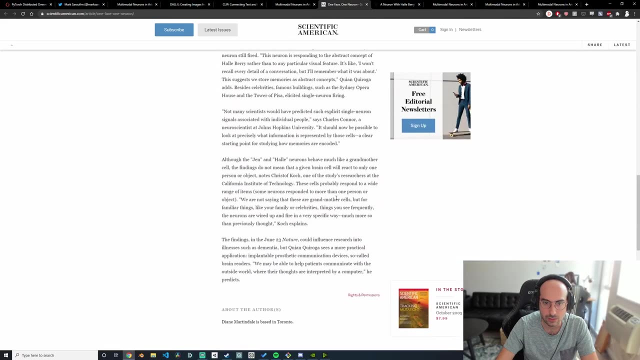 neuron featured in both Scientific and American, that responds to photographs, sketches and text. Halle Berry, but not other names. Okay, let's look at this. Oh, interesting. Okay, so this is not like, just like computationally, It's not a computational. 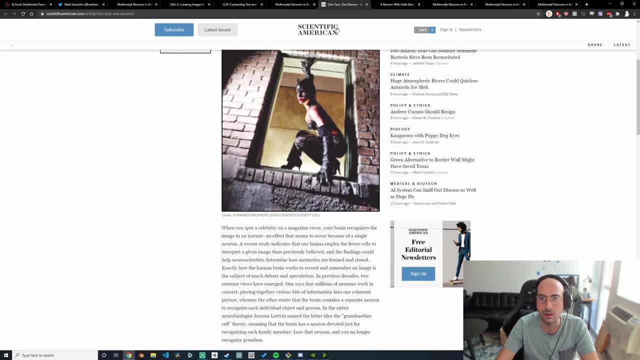 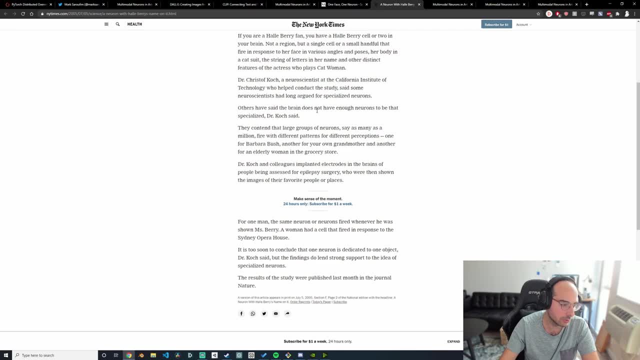 response. It's actually. it has a neuroscientific basis. So, yeah, someone's neuron only responded to Halle Berry. That's interesting And that's a higher level concept than you would expect. You would expect groups of neurons to encode concepts Instead. it seems that like it's not true. So 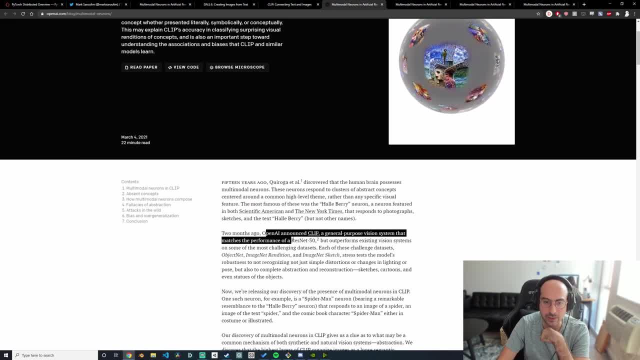 let's just keep going through this. So two months ago, OpenAI released a new version of Clip. that announced the Clip And so I also have a Clip right here. We'll go over it in a second. And Clip is a general purpose vision system that matches the performance of a ResNet-50,. 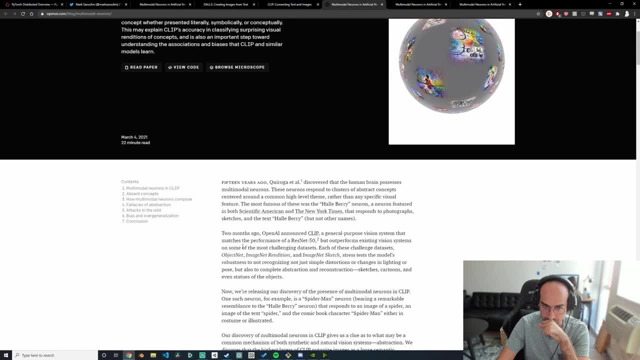 which is the most common image architecture, But it outperforms existing vision systems on some of the most challenging datasets. So each of these challenging datasets- ObjectNet, ImageNet Rendition, ImageNet Sketch, stress- test the model's robustness to not recognize, not just 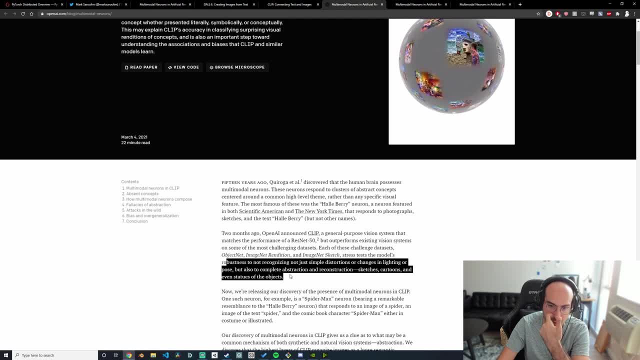 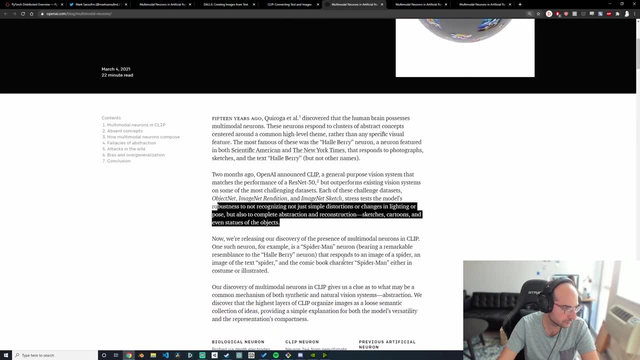 simple distortions or changes in the layout, but also the performance of the model's robustness. So it's just like a harder vision test than what we're traditionally used to. So our discovery of multimodal neurons in Clip gives us a clue as to why. 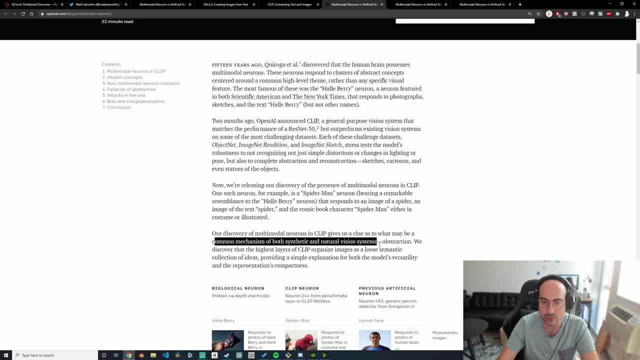 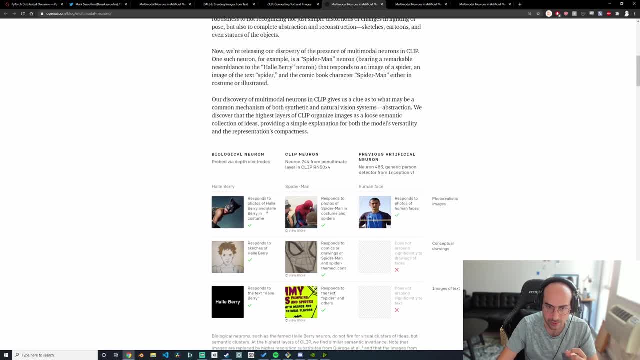 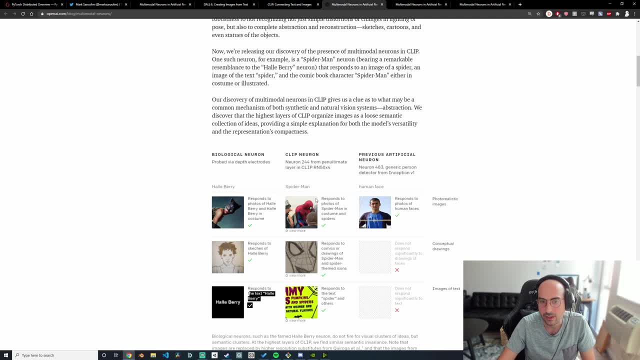 like that causes a similar response With the Clip neuron. they're saying: okay, well, we can also respond to a photo of Spider-Man, a sketch and the text. So these are all the same concept, uh, whereas here, for example, uh, you know you have a human face, but it does not respond to. 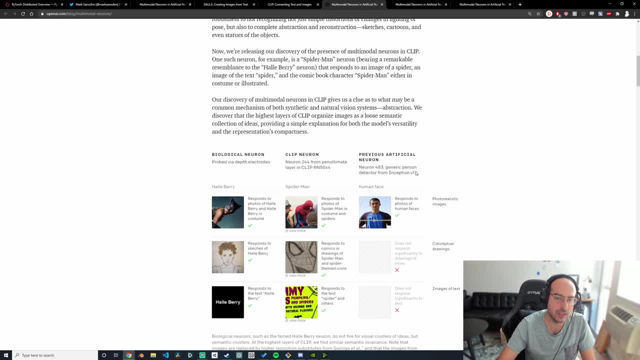 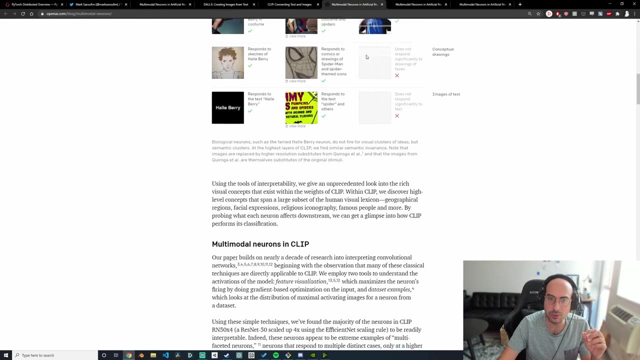 text or anything. so this is sort of the traditional inception net. inception net is really just uh like, just a deep vision architecture. it's nothing, uh like. the word inception comes from going deeper. it's not necessarily something related to anything fancier than that, so i think it should be helpful. 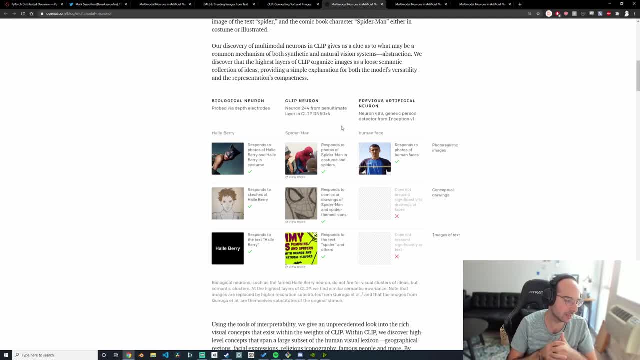 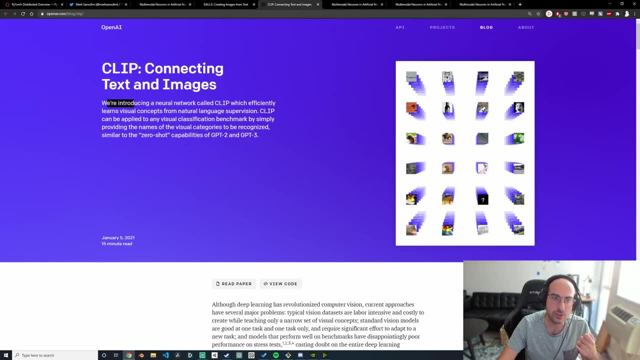 now, like now that we know why this work is impactful, because, like now, we have models that work over abstract concepts, i thought it'd be interesting to just go over clipped very quickly and then see what it's about. so clip efficiently learns visual concepts from that, from nlp and it. 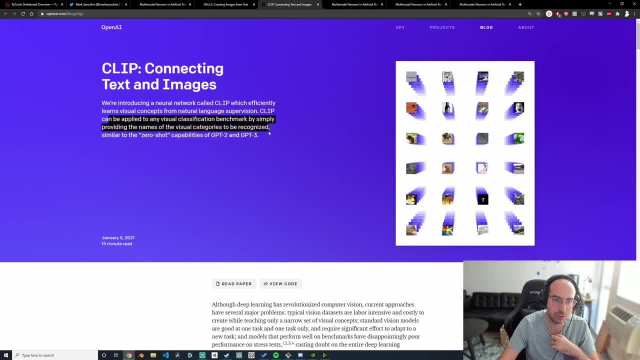 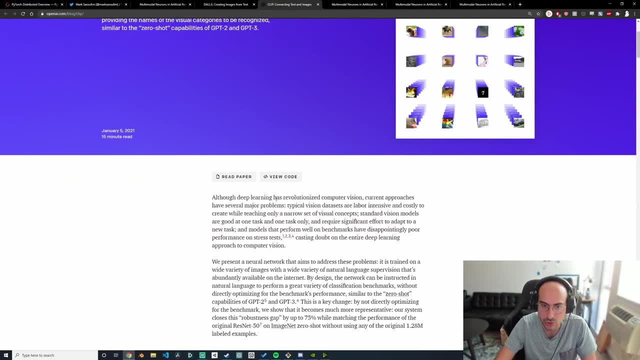 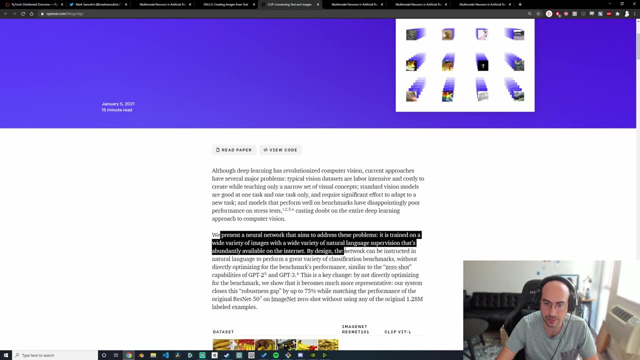 can be applied to any visual classification benchmark by providing the names of visual categories to be recognized. all right, so deep learning has recognized as revolutionized supervision: uh, labor, intensive, costly. okay, it is strained on a wide variety of images with a wide variety of natural language provision. that's abundantly. 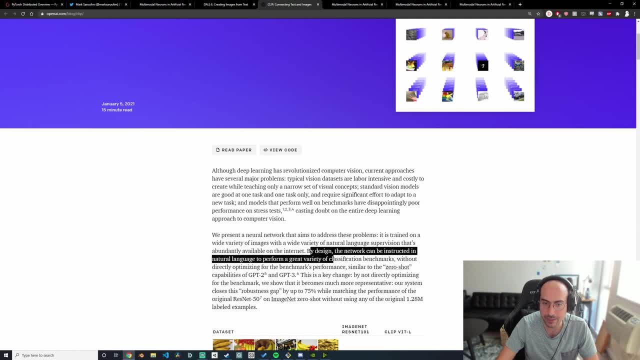 efficient and can be applied to any visual classification benchmark. by providing the names available on the internet and the network can be instructed in a natural language to perform a great variety of classification benchmarks without directly optimizing for the performance benchmarks. performance similar to the zero shot capabilities of gpt2 and gpt3. okay, interesting so. 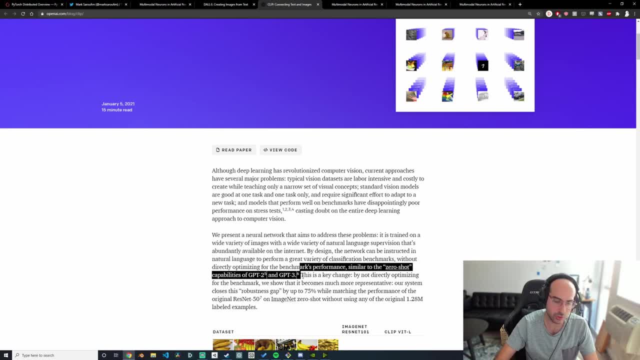 it seems like it's a natural extension of the zero shot classifications of gpt. i have a video about gpt. if that's interesting, uh, but that's interesting. so it's really applying the sort of similar idea to images. okay, without using any of the original live. wait, wait a minute. 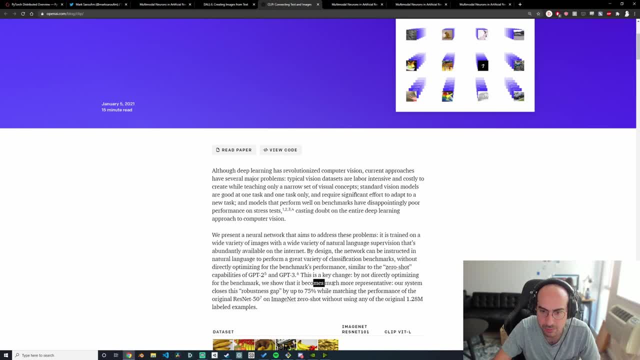 this. by- not by directly- optimizing for the benchmark, we show that it becomes much more representative. but this is not on board. okay, so supposed to work. okay, so this is why R transfer measurement system closes this robustness gap by up to 75%, while matching the performance of the original. 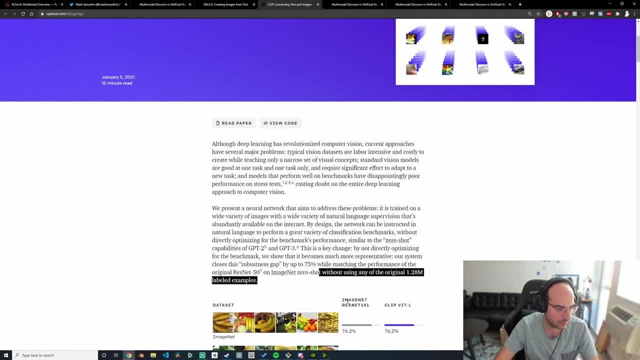 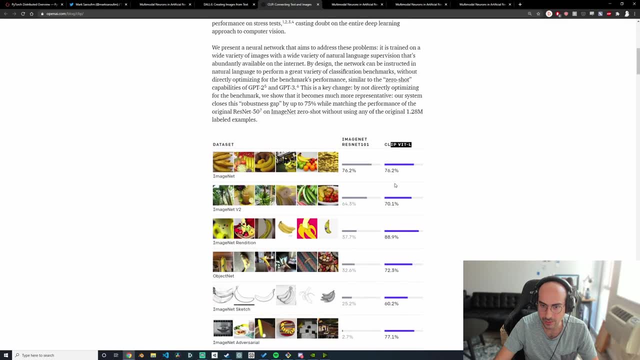 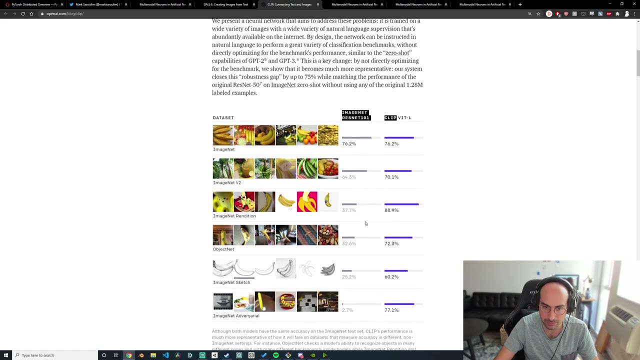 resnet without using any of the original labeled examples. okay, this is kind of crazy actually. okay, how does this work? So how does this work? um, it's like clip, uh, i think you know large or something. what's what does vit mean? well, we'll figure it out all right. so, first off, it seems like it beats resnet 101, which is pretty. 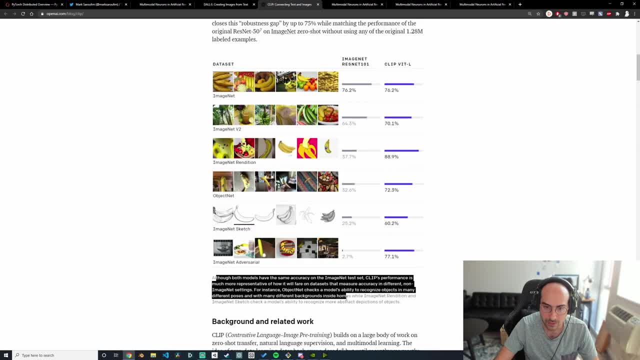 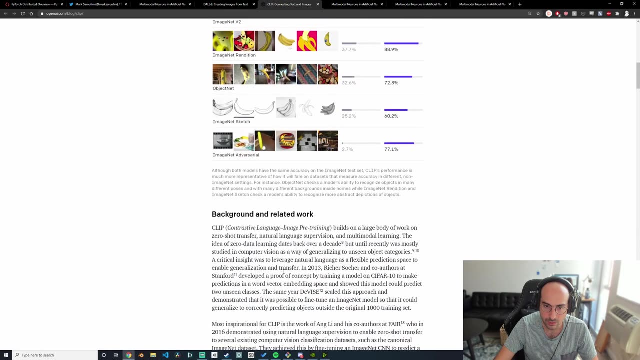 big in of itself: 101 layers. right object net checks a model's ability to recognize objects in many different poses and with many different backgrounds. okay, okay. so contrastive language image pre-training. oh, interesting so already the fact that this is very interesting in that i recently had a video about simclear, which is also a contrastive approach to distinguish images. 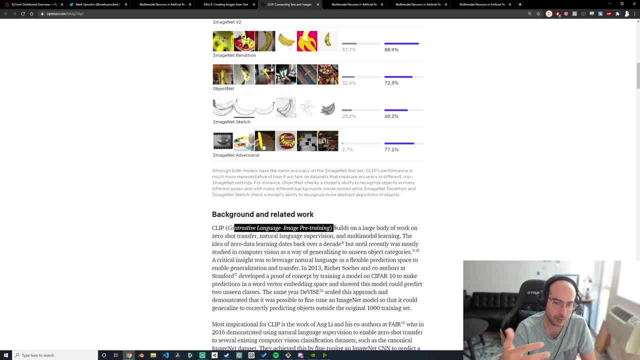 and it lets you build representations that are pretty good, because if you can distinguish stuff, that means you can class. you can classify that they're different. uh, so it's just like. so it's interesting that this contrastive idea is becoming so relevant and so contrastive language image. 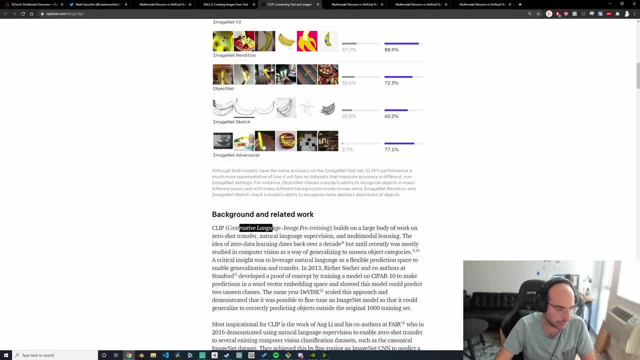 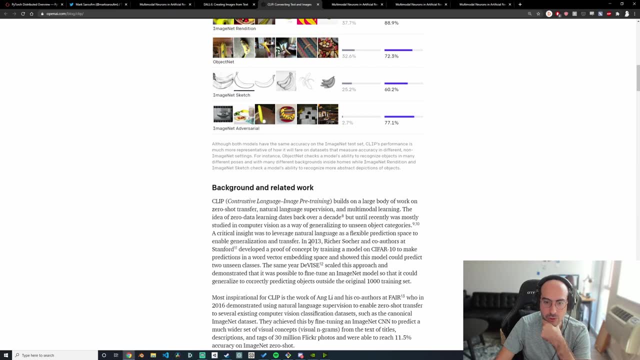 pre-training. okay, so we're gonna you. we do something with language, with this contrasting. okay, let's see. um, okay, richard socher and co-authors at stanford developed a proof of concept by training a model on cypher 10 to make predictions in a word: vector embedding. 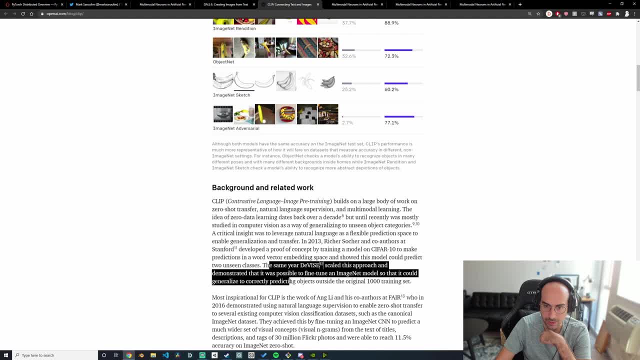 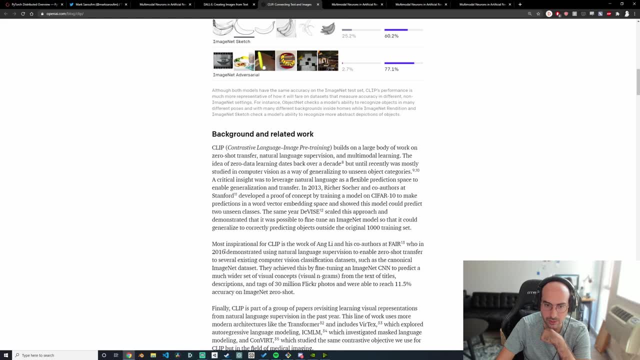 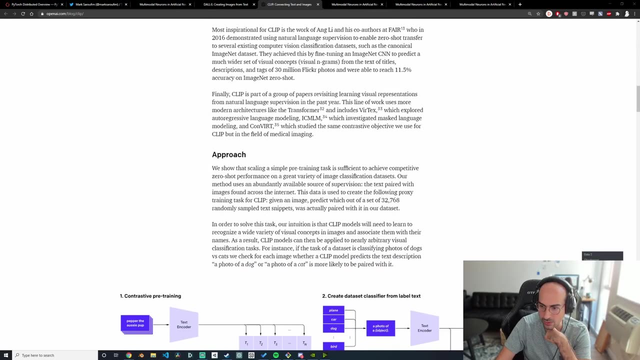 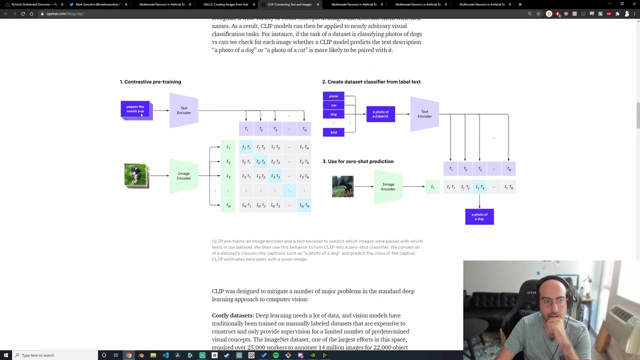 space and showed the small could predict two unseen classes the same year they scaled this approach. most inspirational is the work of ang lee and his co-authors at fair using nlp to enable zero shot transfer. okay, okay, so far, so good. okay, let's. let's look at this image quickly so we have a text encoder, uh, for a sentence, and then we 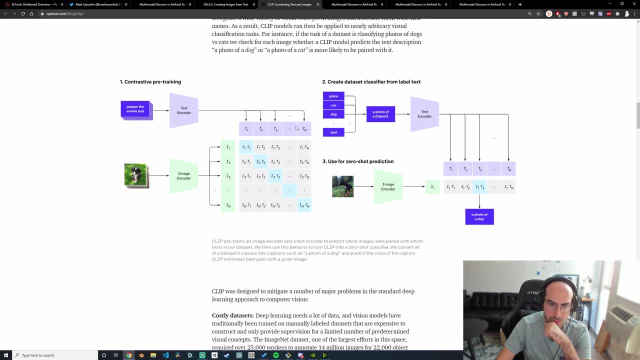 have an image encoder for the image, that's cool. so we get two vectors out of these and then from these vectors, looks like we place them, we put, looks like we create all pairwise, like all pair, all pair possible pairs, and put that, put it in a matrix. 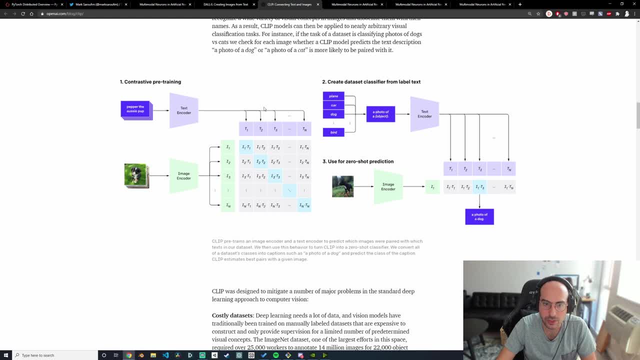 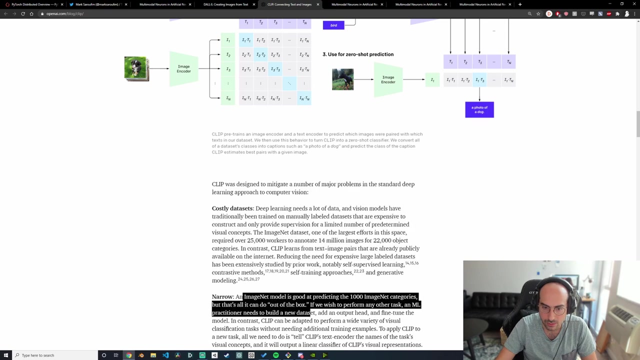 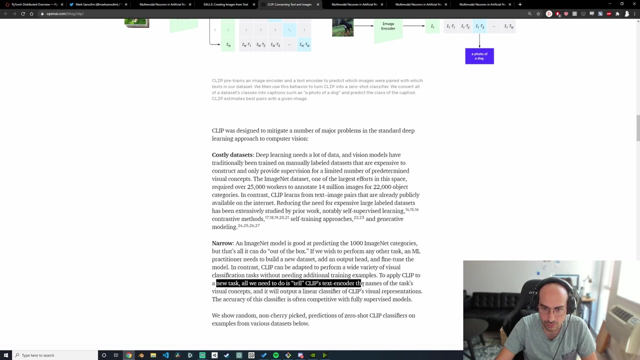 uh, okay, and then so this is the pre-training step. and then we create a data set classifier from label tags, so plain card, dog, bird, photo text encoder, an image encoder, and then i see. so so basically figure out like how to index into this representation. you all right. so so traditionally, this is interesting. they're saying like let's say, you want to get a pre. 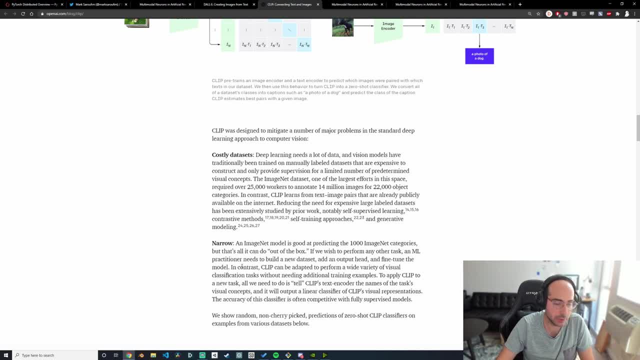 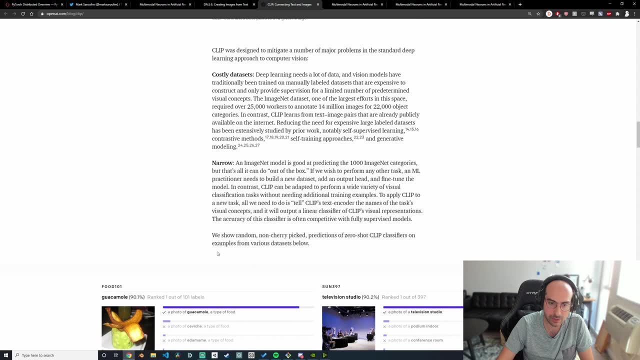 you have a pre-trained language model and you want it to work on a new class of images. well, either you train the thing from scratch on this larger data set, or you take the pre-trained model and fine-tune it on the new labels. so instead, here a photo of guacamole, a type of 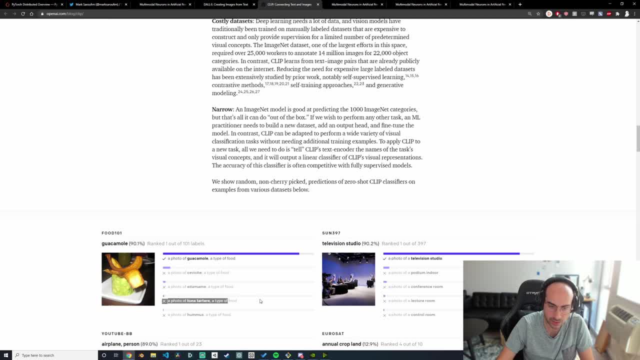 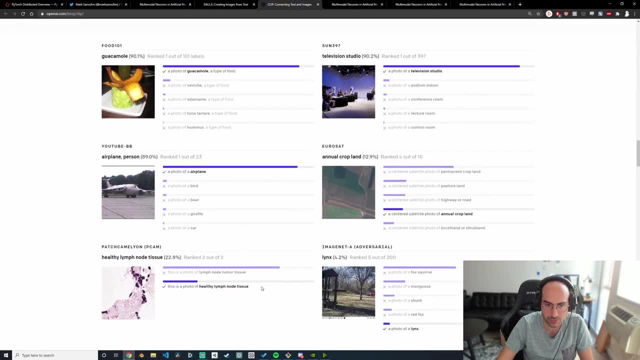 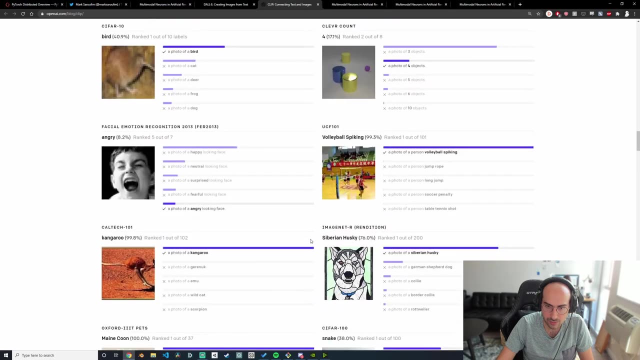 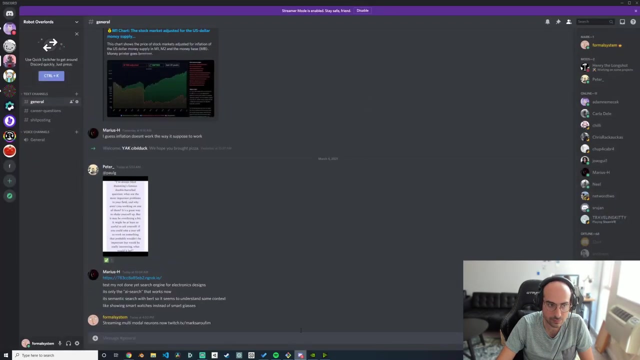 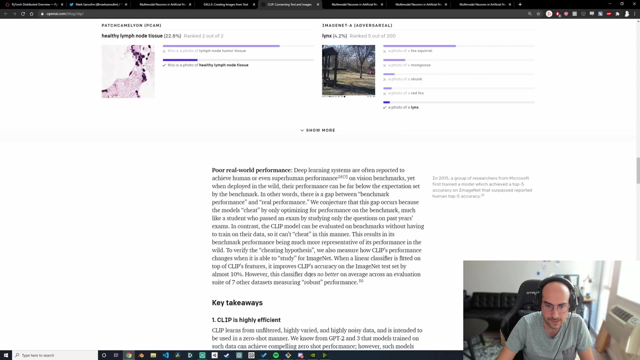 food. a photo of ceviche, a type of food, and it does kind of look like all of them, but television studio podium. okay, This is a photo of a healthy lymph node tissue. This is a very cool example. it's actually very pretty. All right, so let's look at the key takeaways. 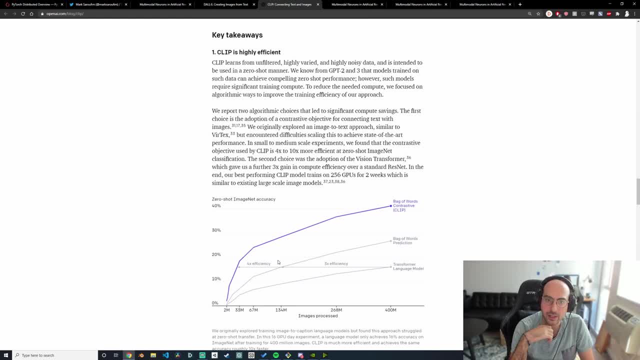 So Clip learns from unfiltered, highly varied and highly noisy data and is intended to be used in a zero-shot manner. So we know that GPT-213, trained on such data, can achieve compelling zero-shot performance, but they require significant training compute. 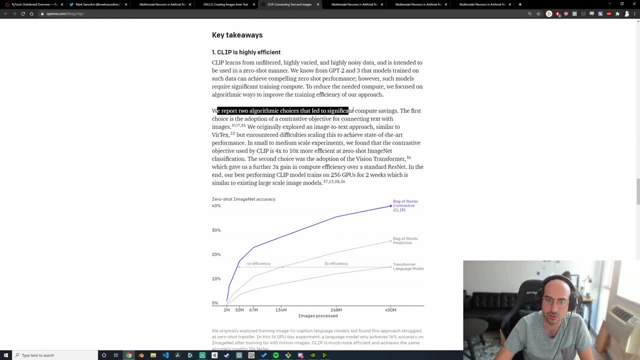 And so now they're saying: how can we make this more efficient? Is adoption of a contrastive objective for connecting text with images. We originally explored an image-to-text approach similar to Vertex, but encountered difficulty scaling this. So Clip learns from unfiltered, highly varied and highly noisy data and is intended to be used in a zero-shot manner. 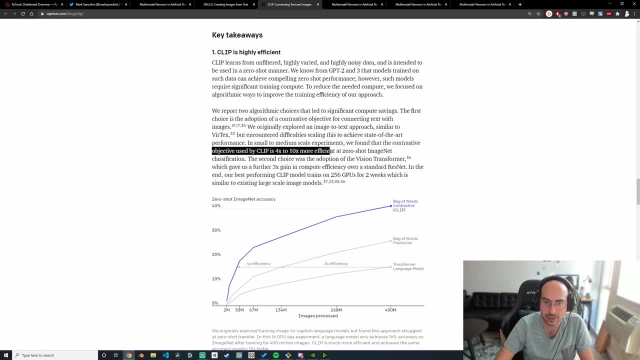 So Clip learns from unfiltered, highly varied and highly noisy data and is intended to be used in a zero-shot manner. The contrastive objective used in Clip is 4 to 10 times efficient Was adoption of a vision transformer, which gave us a further 3x gain in compute efficiency. 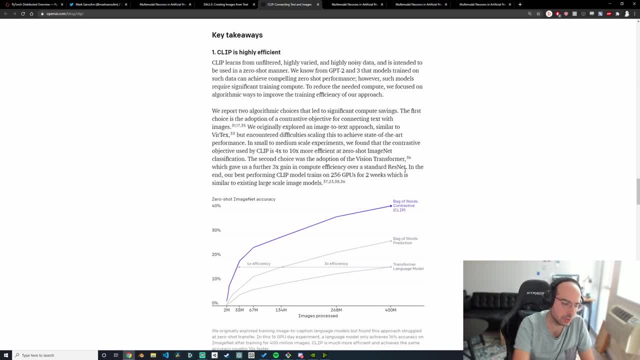 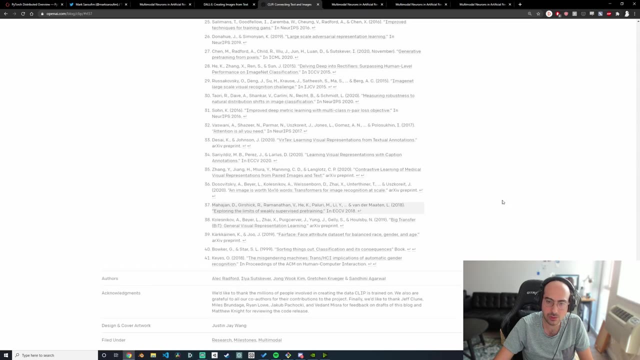 over a standard ResNet. That's nuts. I wasn't aware that vision transformers were computationally more efficient than ResNet. I'd have imagined that it would be a lot less efficient. Bag of words: contrastive Clip: OK, Our best performing Clip model trains on 256 GPUs for two weeks. 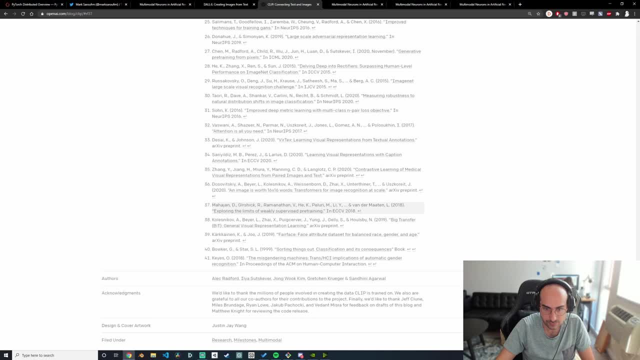 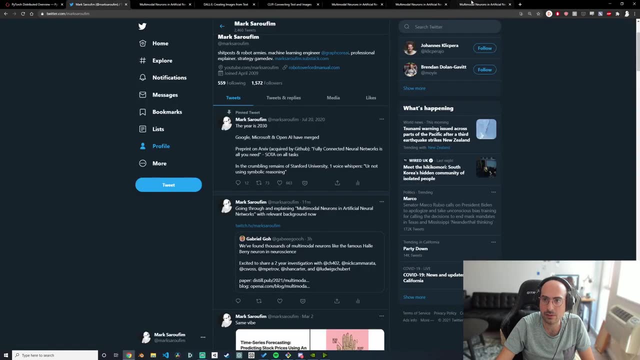 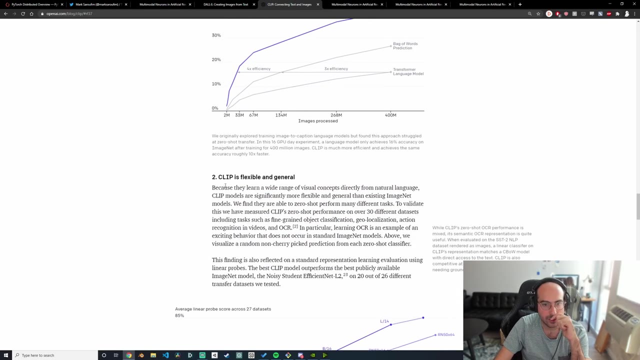 Oh, wow, OK, We're getting close to a million views, Which is similar to large-scale existing models. So it's flexible in general. So it learns a wide variety of visual concepts. So they measure Clip's zero-shot performance on over 30 datasets and learning OCR is an. 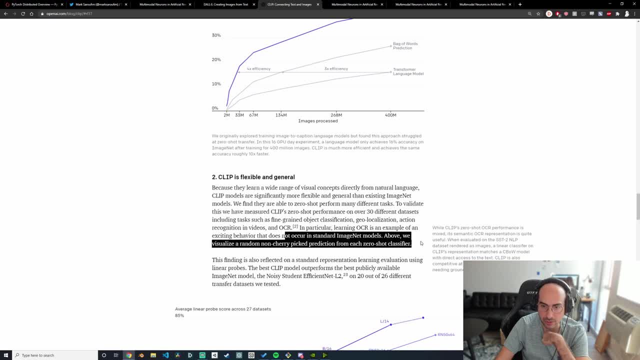 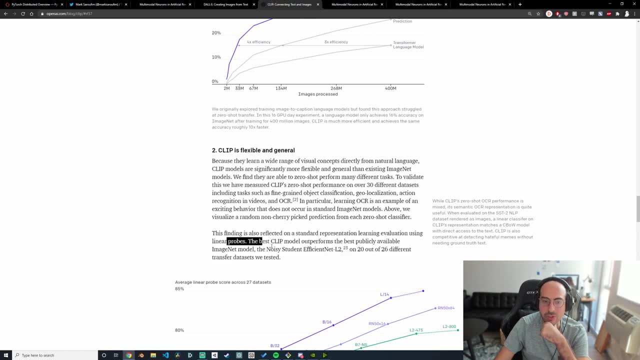 example of an exciting behavior that does not occur in standard ImageNet models. OK So, And this finding is also reflected in a standard representation- learning evaluation using linear probes: The best Clip model outperforms, the best publicly available ImageNet model? or the noisy student-efficient? 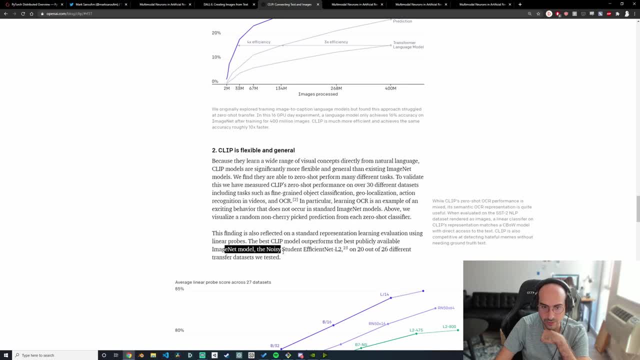 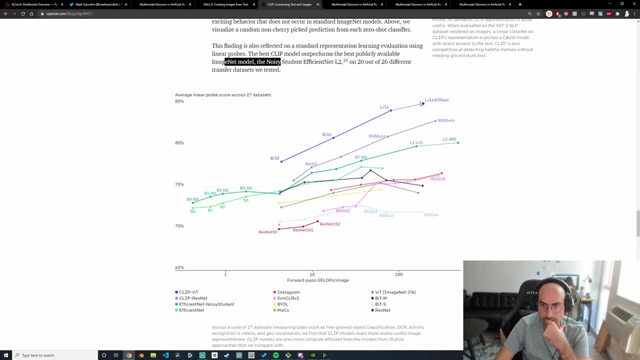 NET L2 on 20 out of 26 different transfer datasets that we tried. Let's look at this. I wasn't aware ResNet is just so poor, actually, relative to these other architectures. What is this RN? OK, So this is Clip. 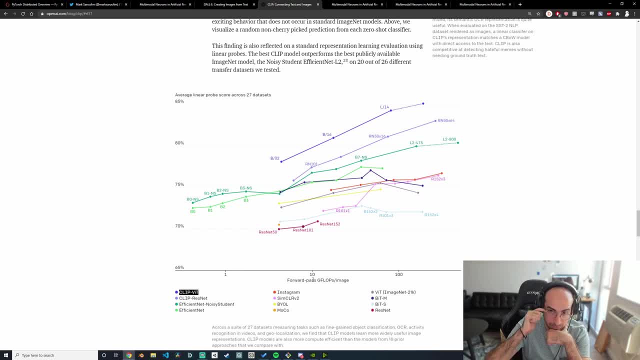 Seems to be FortPass gigaflops per image. OK, So OK, Yes, We need to compare this left to right, But essentially it looks like, at least comparing it to standard ResNet, there's about a 7% improvement. 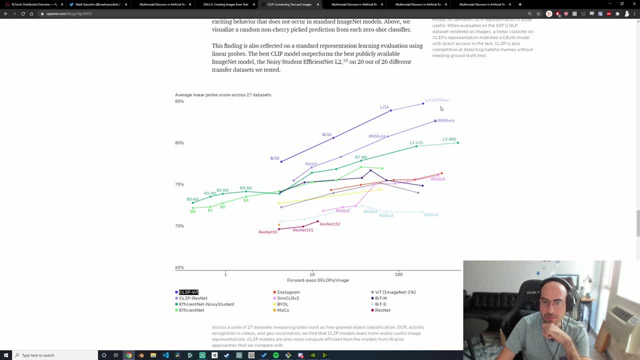 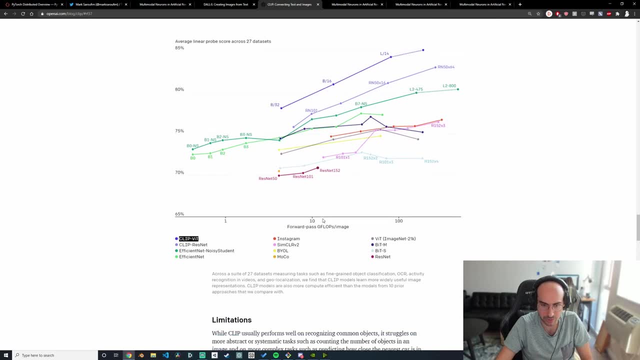 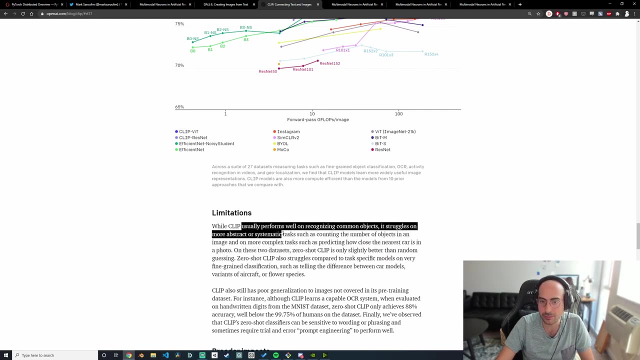 And then it scales better with the compute. It's like: well, with more flops like this grows exponentially, whereas here, you know, not so much. So it looks like Clip does well to count objects, but not so much at complex tasks like counting things. 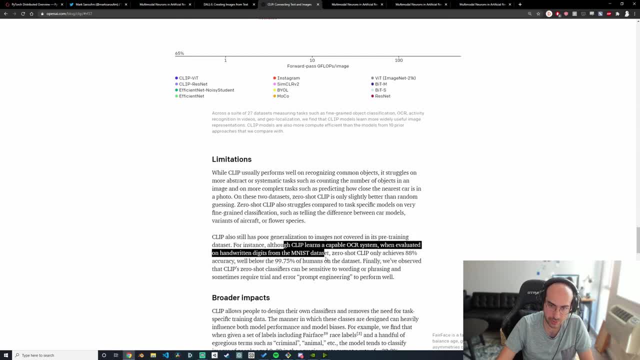 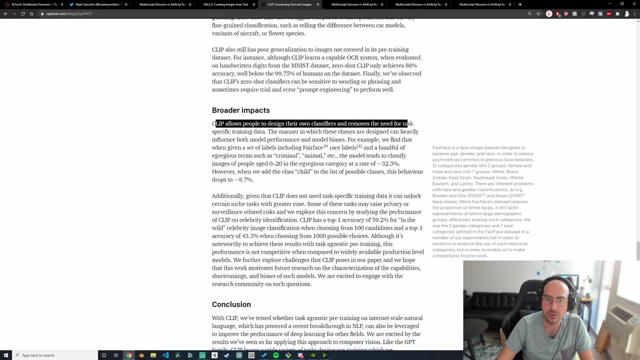 It also has poor generalizations to images not covered in its pre-training data sets. OK, So what's the broader impact? OK, Let's see, Let's see. OK, So what's the broader impact? So Clip allows people to design their own classifiers and removes the need for task-specific training data. 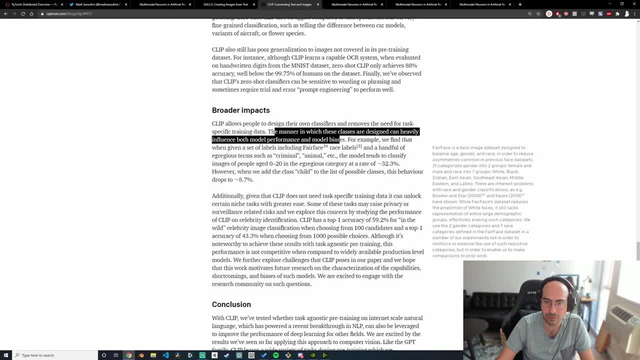 The manner in which these classes are designed can heavily influence both the model, performance and bias. So when given a set of labels, including fair face, race labels and a handful of egregious terms such as criminal and animal, this behavior drops OK. 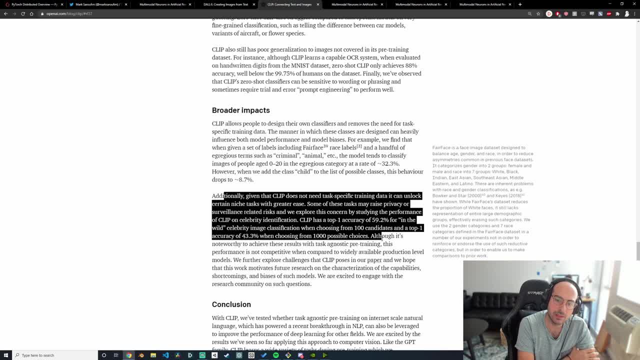 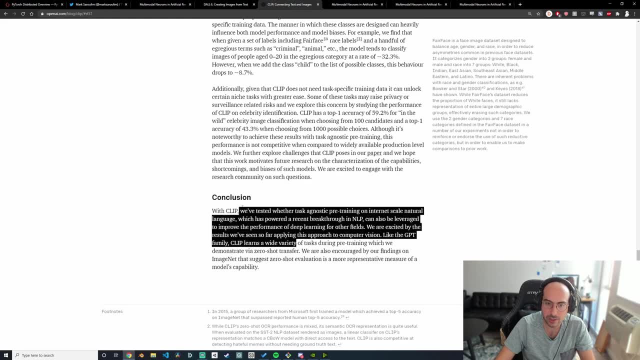 I mean, yeah, Like I can imagine that a lot of these biases are there. OK, It's just that the bias problems get like way more amplified. So let's see. We've tested whether a task-agnostic pre-training on internet scale has inspired a recent breakthrough in NLP. 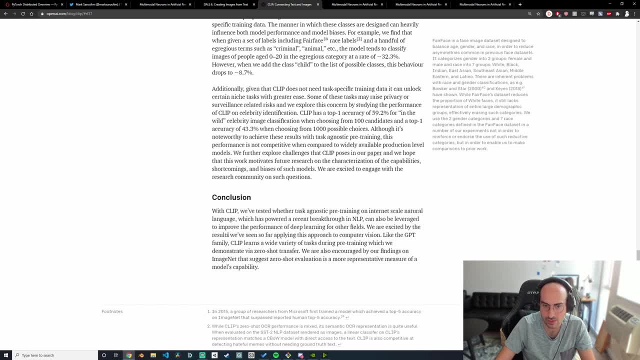 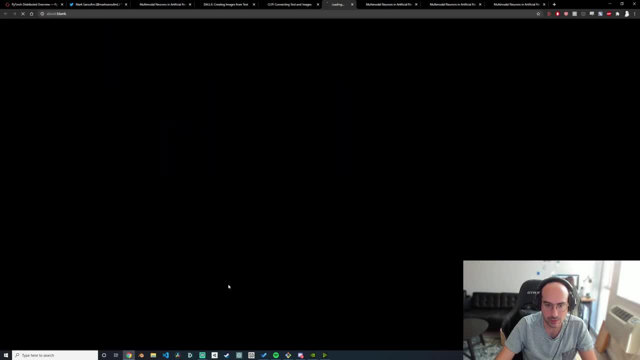 It can also be leveraged to improve the performance of deep learning for other fields And we're excited by the results. and Clip learns a wide variety of tasks. OK, This is good. Let's quickly go over the paper And is the – OK, 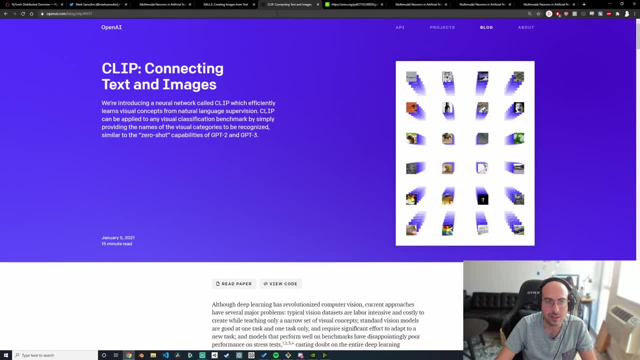 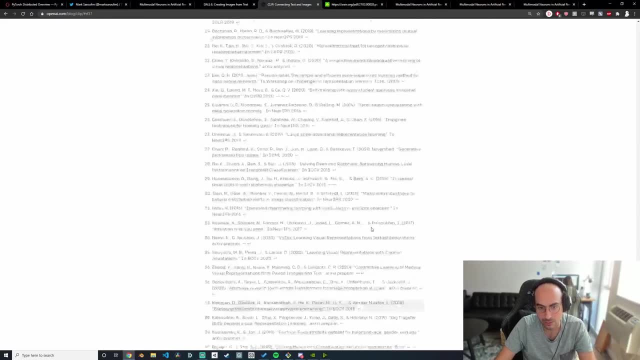 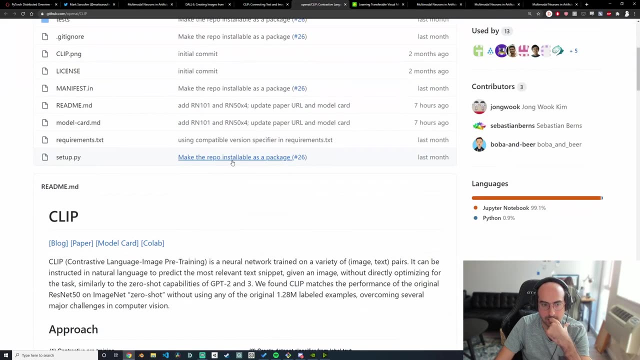 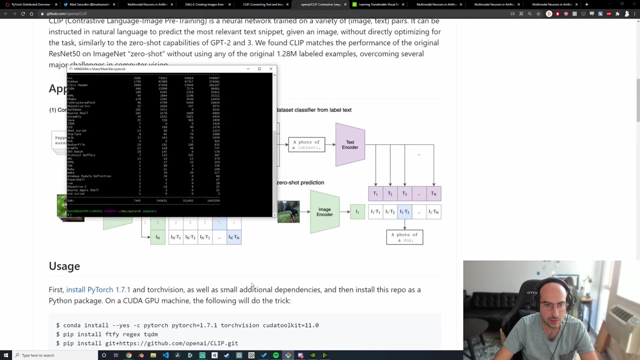 Of course, That's Alec Ratford, And let's also just quickly skim the code, OK. Okay, so let's get this thing here. Okay, so, it's gonna clip, and I'm just gonna just get some sense of how complicated this project is. Okay, so, it looks like the actual project, isn't that? 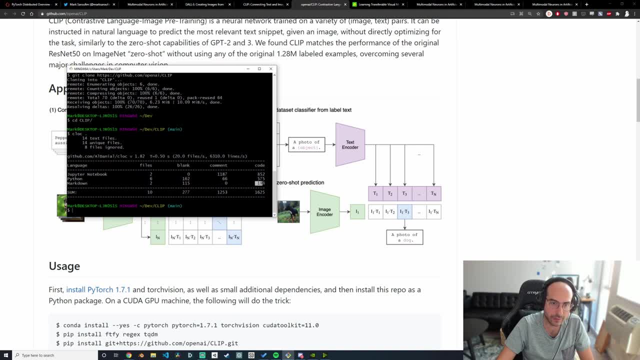 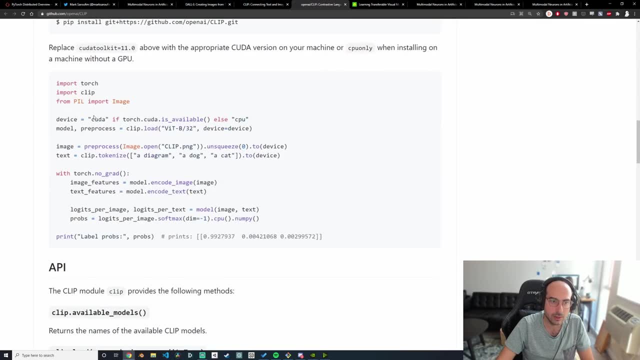 complicated. It's about like 600 lines of Python and then the Jupyter notebook looks longer than that. mostly markdown, So that's good. So it means like the idea is, at the end of the day, kind of simple, So okay. so how does this work? So we 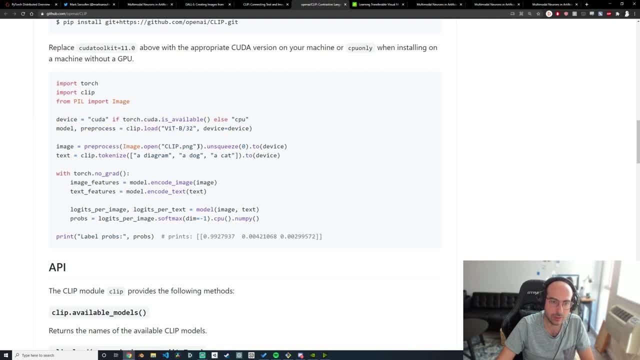 pre-process the data image, open clip NLP, unsqueeze it and send it to the device, because I guess it becomes an umpire array, And then tokenize the sentence and also send it to the device. So now we have this image and text. We encode the image, we encode the text and 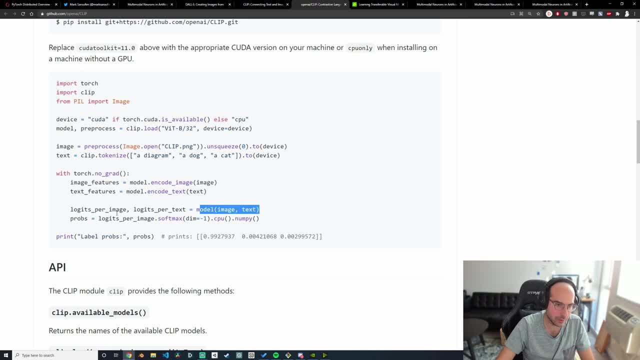 then we pass both to the model, And after that we do a soft Mac and we take the last, the most likely entry- No, not the most likely entry. We just like- oh sorry, we linearize it into a line, into a vector, send it back to the CPU. so we 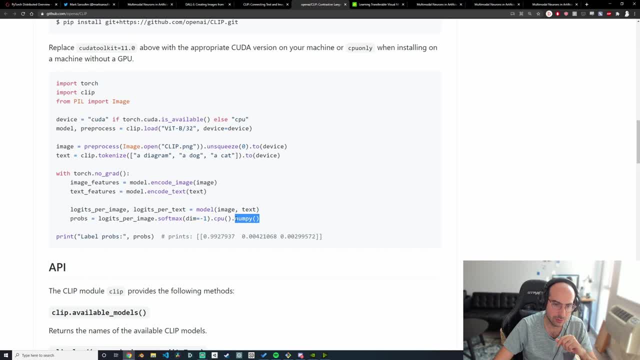 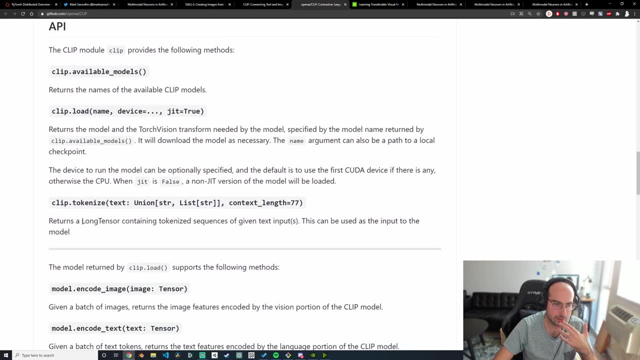 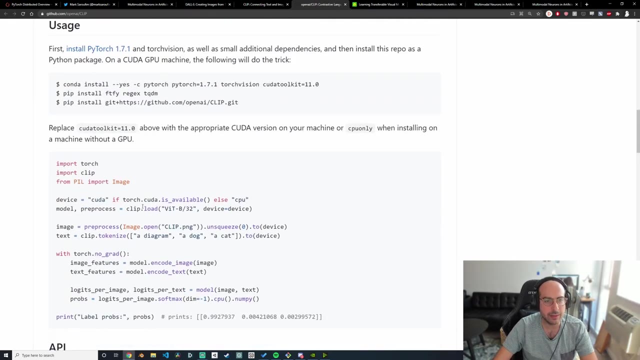 can read it and then back to NumPy. I don't think we need to do that, Or maybe you do, I don't know. Long tensor content of given. this can be used as input to the model. Okay. So one thing I'm not too clear on is: are there pre-trained weights here? So first off, 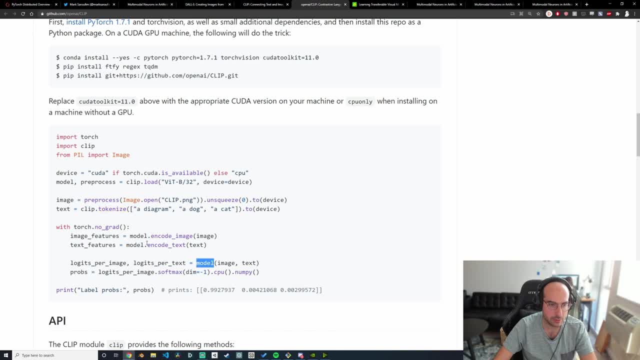 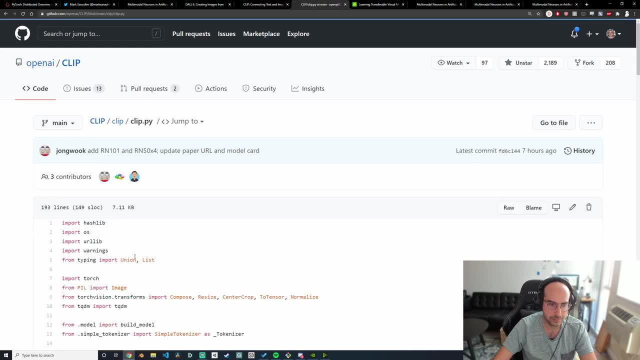 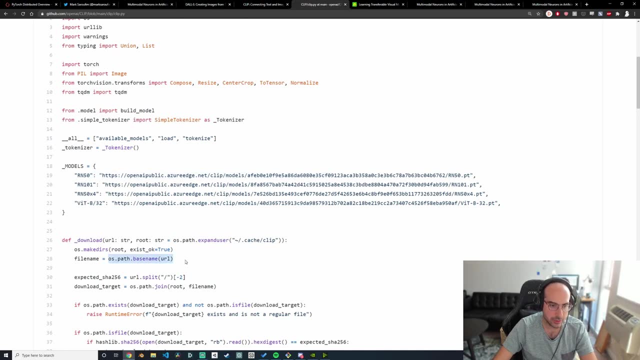 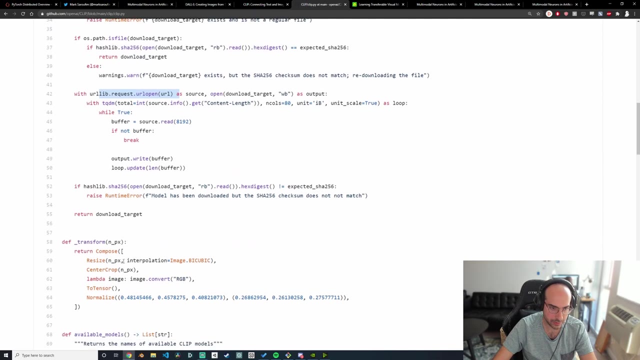 So clip, then clip, All right. So this is, I guess, where the model files are, And so when you're downloading it you just like call the URL. I'm assuming you use, like the request API to get everything. Okay, URL lib, It's the same idea. This is the image. 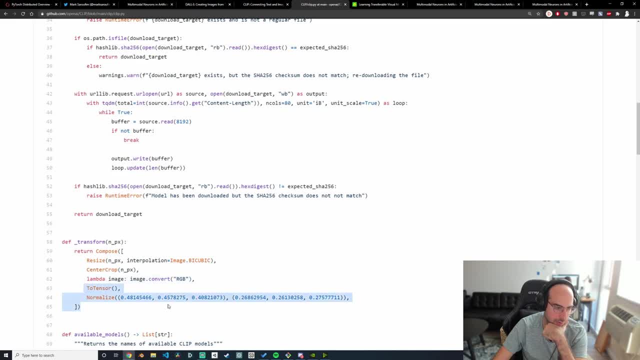 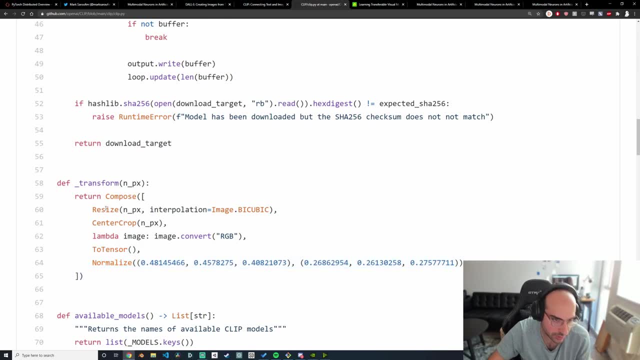 pre-processing stuff, like resizing the image center, cropping it. So this is like really nice. I really like these ideas And like PyTorch makes like a lot of these visions. So let's just go to this. It's very easy because you just compose the transforms that you want to do A lot. 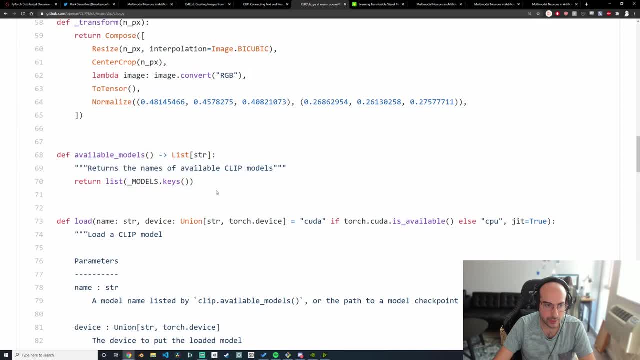 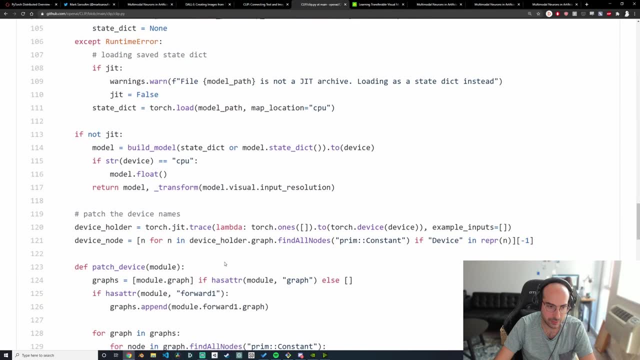 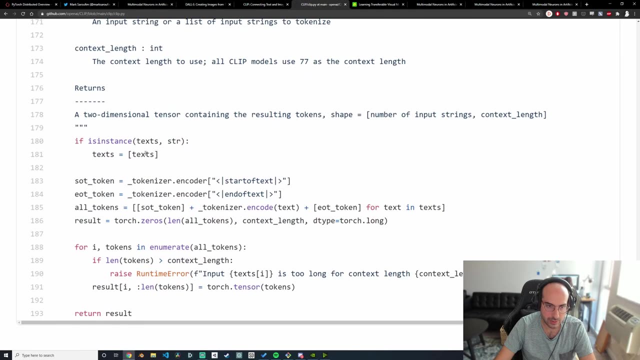 of these ideas I also cover in the SimClear tutorial. Okay, getting the list of models. This is loading the model. We download a model. You load it, just in time. What else do you do? Okay, so tokenizer, How does this work exactly? So? 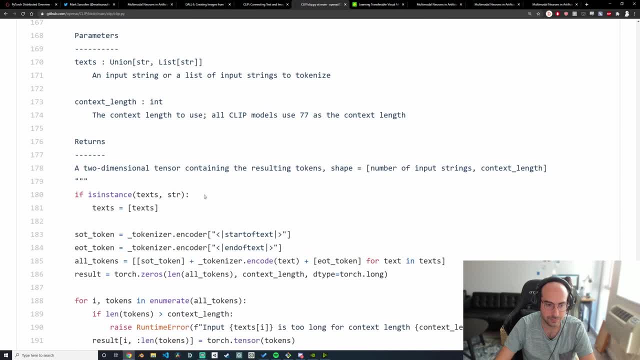 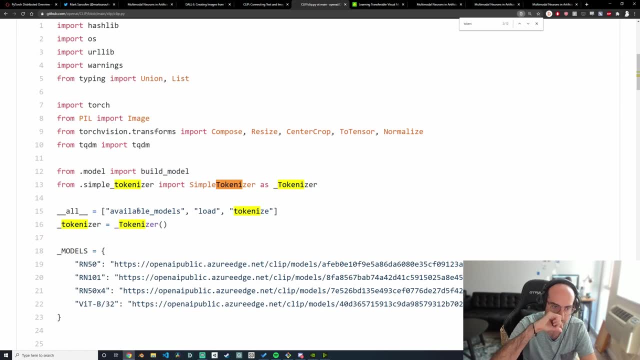 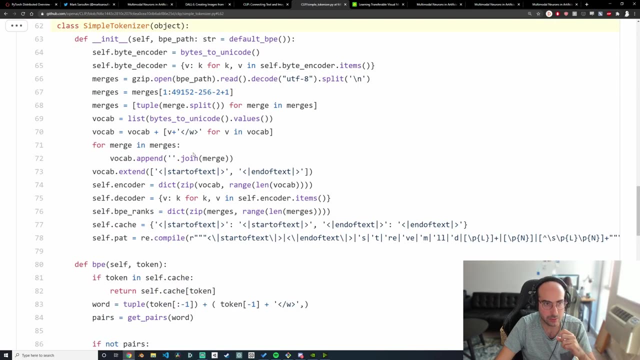 tokenizer encoder. This is passed in a tokenizer From simple tokenizer import. simple tokenizer to tokenizer. What's simple tokenizer? Okay, so it's also here. Let's just take a look. Oh, it's actually a byte: encoder and byte. 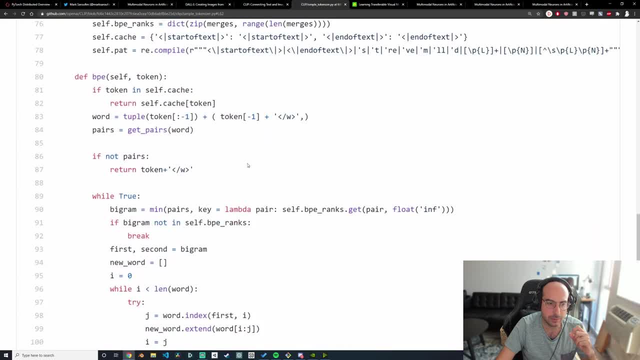 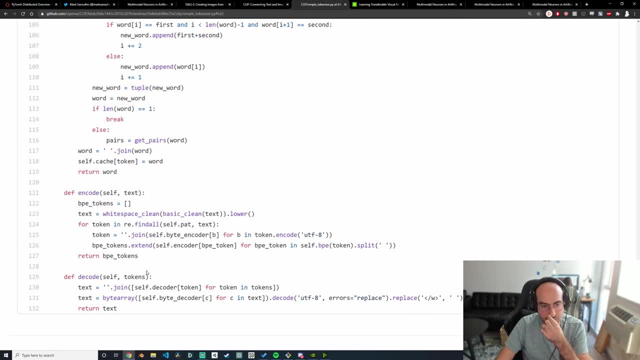 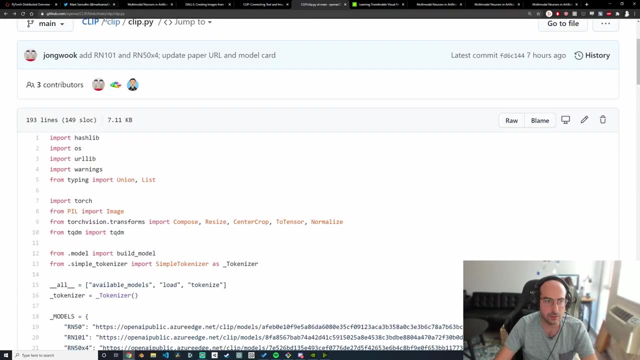 decoder. All right, so we have this vocab: BPE. Okay, this isn't like a Yeah, okay. So that's interesting, that they're actually Looks like yeah, they're turning it into byte tokens. So let's go to the model for. 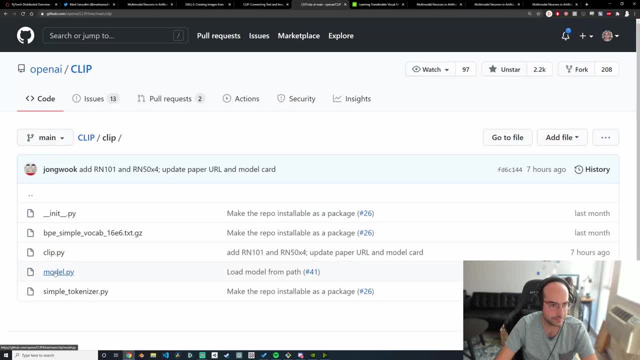 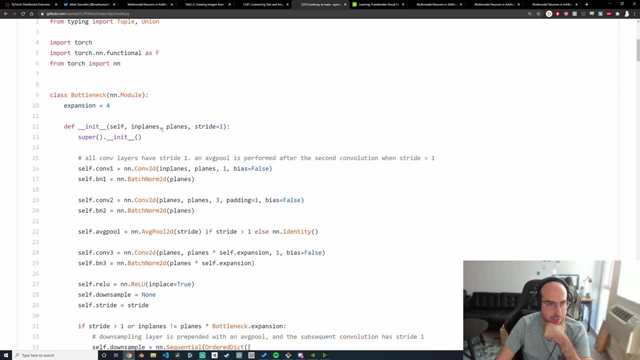 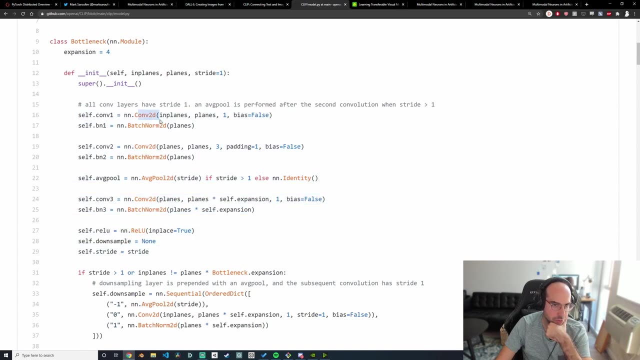 a second just to see how this all fits together. So okay, so they're calling this a bottleneck And this looks like a very traditional CNN architecture. So you typically notice there's a con, a batch norm, some relus Here there's. 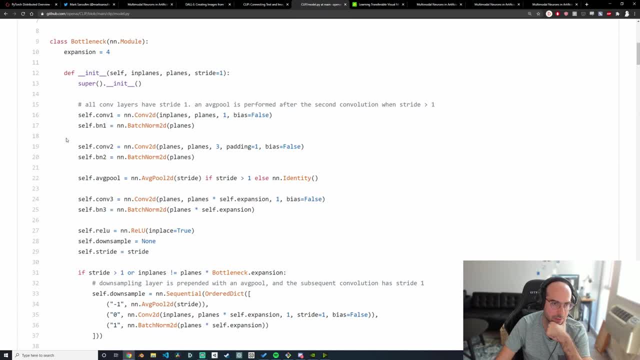 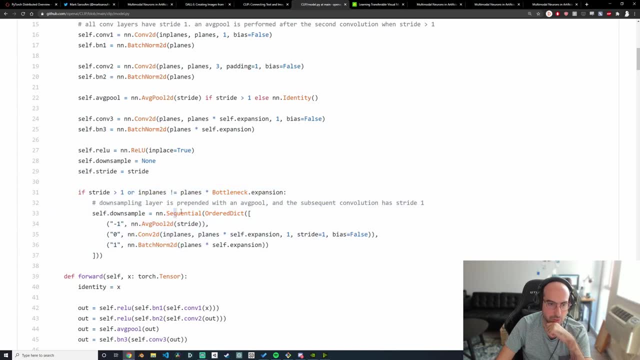 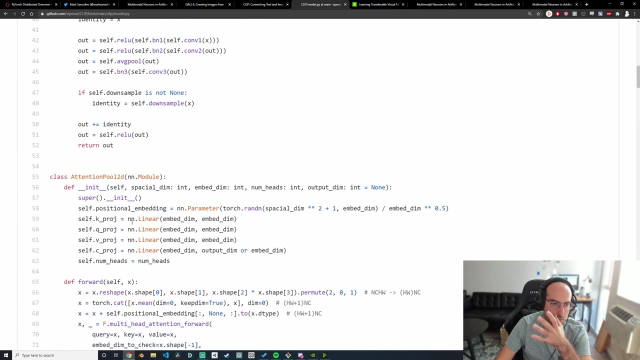 only a relu at the very end, which is interesting because typically I'm used to seeing the relu at the very end. And then what do they do? Okay, sequential order, dict Okay. and so I guess, like they do, like a bunch of them, This is the forward pass which makes sense. They have this module. 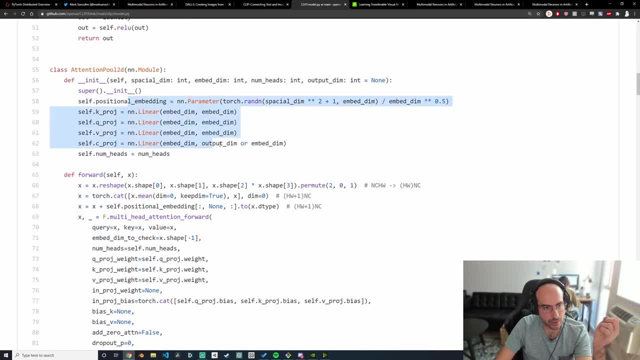 called an attention pool. Okay, so this is. you know, like you have the key, you have the projection and the value. So a lot of the similar ideas from regular transformers are here, So linear layers. you know transformers sound more complicated than they are The actual. 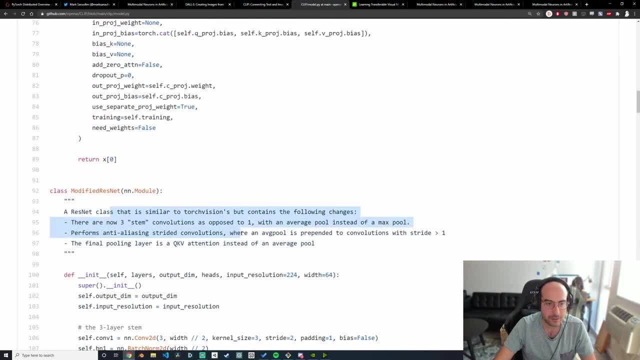 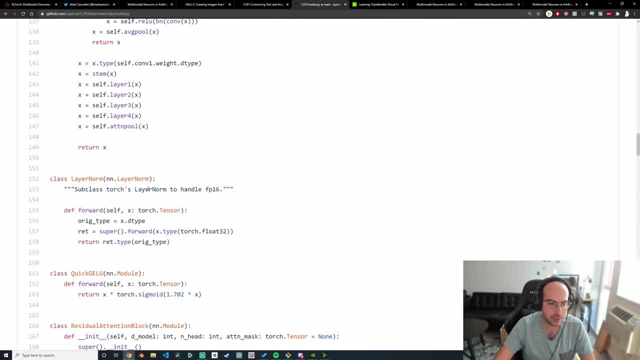 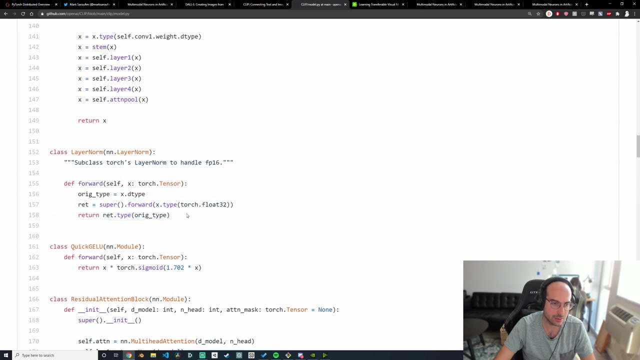 implementation is often surprisingly simple. So this is a different version of Resna. That's fine. I think that's probably for their benchmarks and the layer norm, so that it works for FP16.. Okay, But it doesn't look like it's using FP16.. 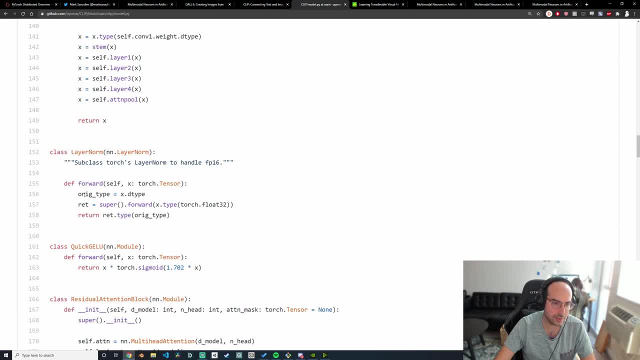 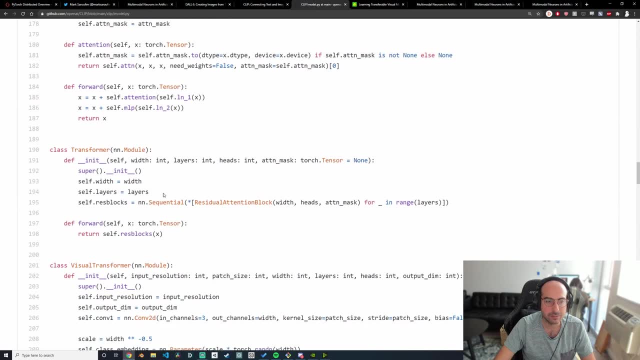 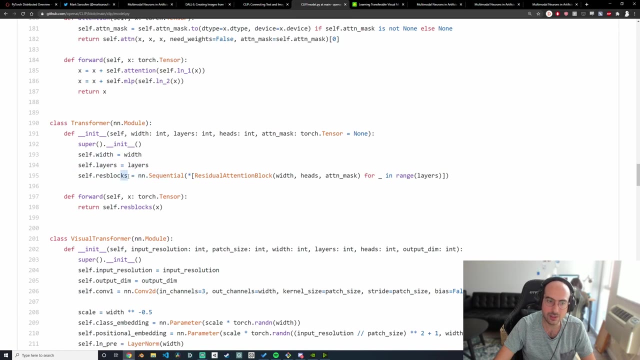 Orge type, XD type. Oh okay, never mind, It just uses the type of this. Okay, That's all fine and good. Okay, so then we have the actual transformer here, And this transformer has some residual blocks, which is just: you see this? So basically, you create a sequential layer, So this is: 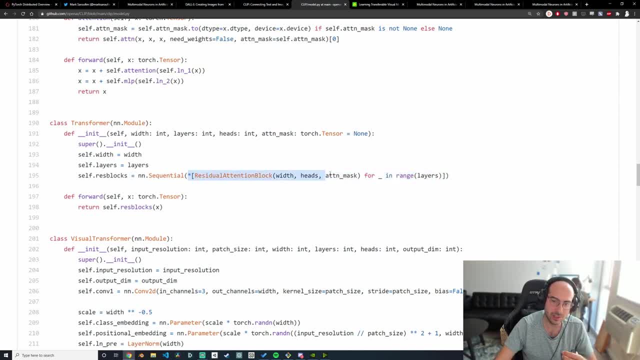 in fact. so you're going to create a list where you have as many of these blocks as you have number of layers, And each of these blocks has a width, a number of heads and an attention mask, And then you basically execute this whole thing sequentially. The 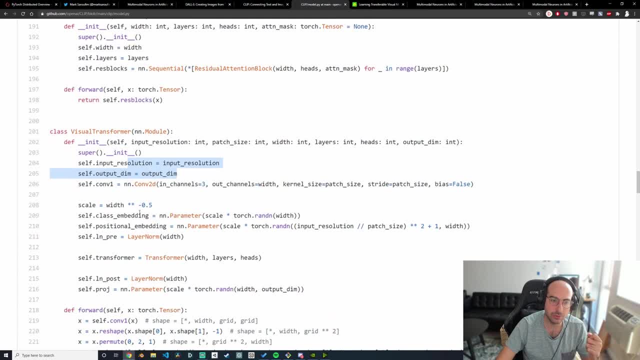 vision transformer. I haven't looked at implementations of vision transformers before, but it looks like we have a class embedding- positional embedding- because I think the way vision transformers work is, if you have like, let's say, an image, you would break it apart into. 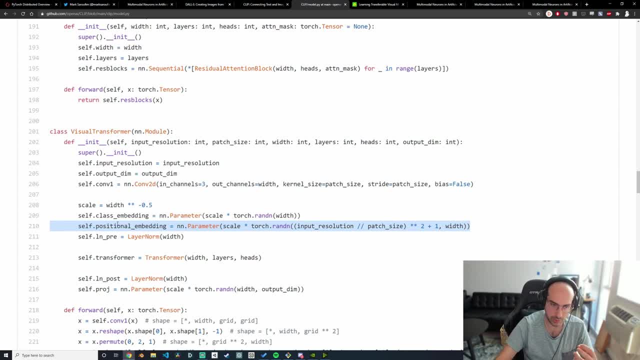 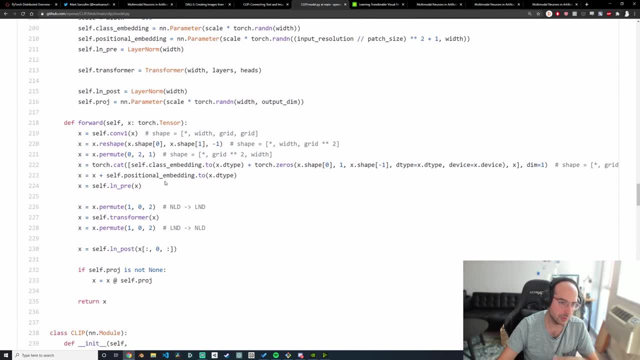 parts, and then you need to keep track of: well, which part are you at? So that's where the positional embedding comes in, Because if you don't have it, then you just don't know the order And it seems like the 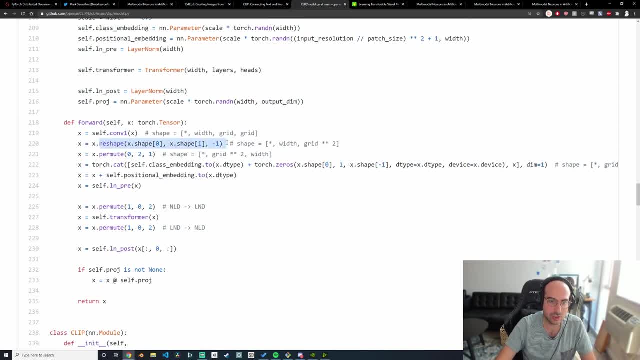 order would probably be helpful. Okay, so the forward pass is a convolutional layer. then they reshape it, then they permute it, They concatenate the class embeddings with this. I don't know what this is really about. So the plus here is also concatenating the 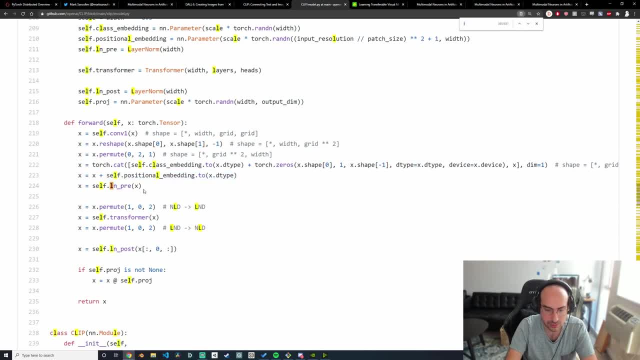 positional embedding. And then I don't know what ln pre is. What is this ln pre? Okay, so it's a layer normalization. Permute again nld lnd. Yeah, I actually like this convection. I wonder why these permutations. 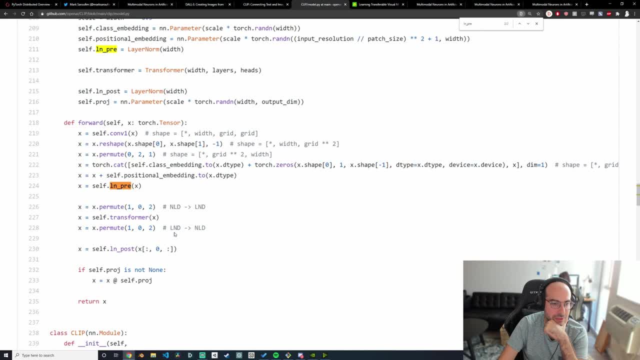 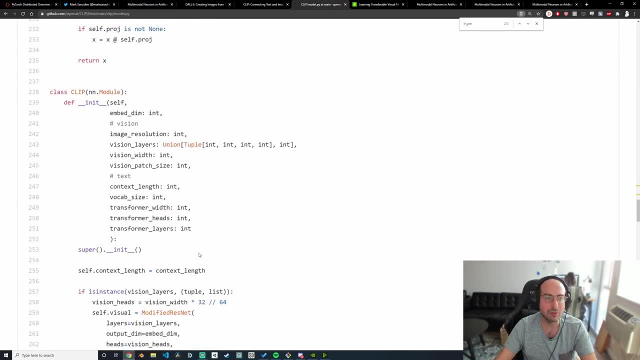 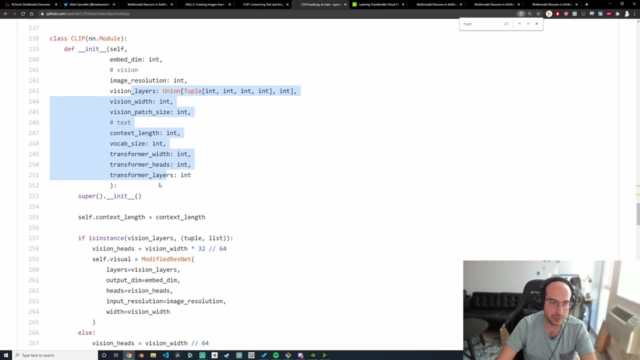 here are so important, Like I need to maybe read this original paper to figure this out. And then this is a matrix multiplication, where you're multiplying x by the projection itself. Okay, finally, we're at the clip module now. So in the clip module we have resolution. vision layer is a width transformer. has 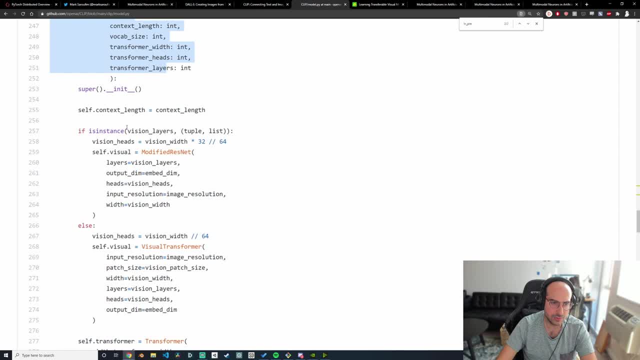 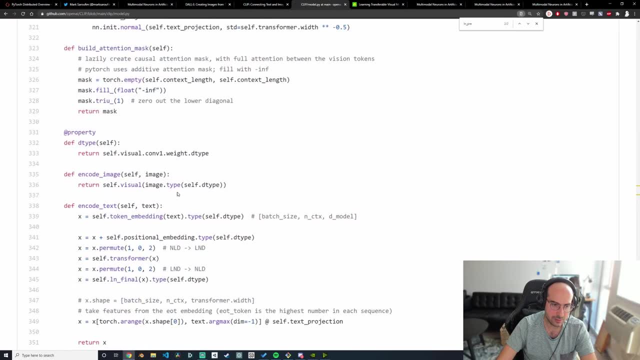 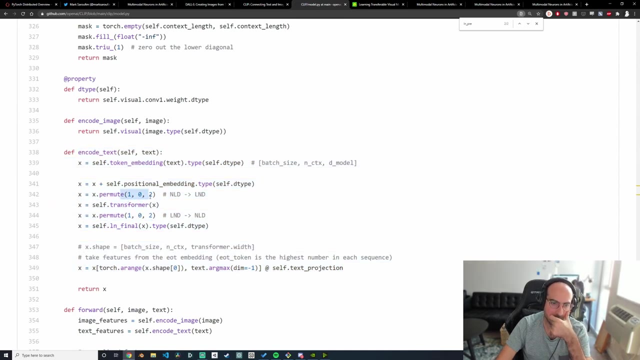 okay, If, as instance, vision layer is tupleless, like I don't know what this is about, Is there a forward pass? Okay, so this is the encode text part that we saw. It's interesting, like on these permutes, like I wonder why they're used so much. Yeah, this is a forward. 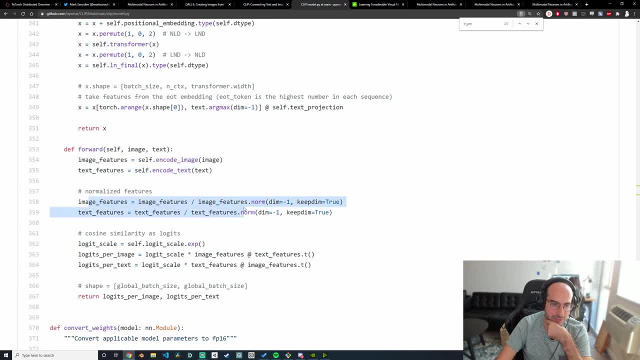 pass. So encode the image, encode the text, normalize the features, It's all fine. Take the cosine similarity as logits. So I think this is like cosine similarity, but I don't think this much of similarity is used a lot whenever you see anything contrastive. So 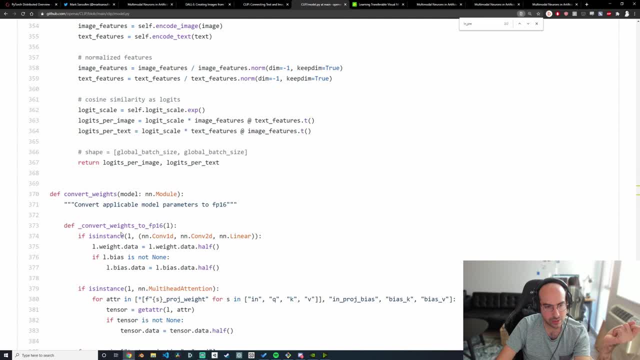 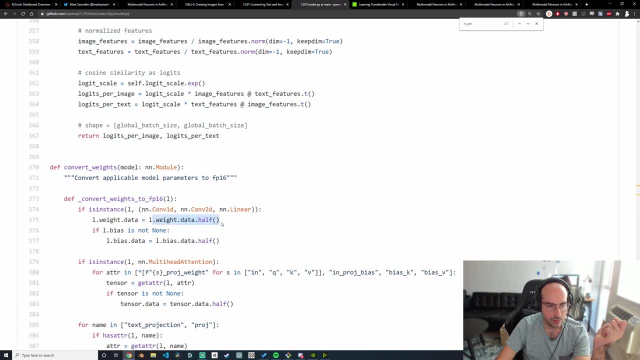 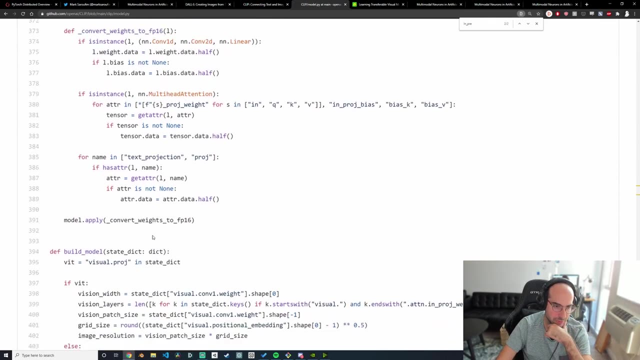 maybe this is where this is coming in. They do some weird stuff to convert everything to FP16.. I'm surprised this stuff doesn't just work out of the box with Pytorch. So yeah, so they take the data, have it, because before having it it's 32 bits And then 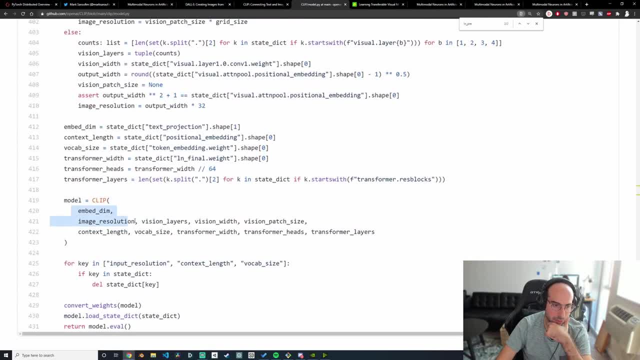 okay, though, this is the whole model, And then they convert the weights of the model. Interesting I see. So Państa Lin's, I have just a hard time saying these two groups thinking about what they're looking for: the die within some of. the global records for this market. I think it's pretty ridiculous because I saw already like on theся respect agency has the product habits on the blog, rationalizing a bunch string and then you can say, okay, do you think it's that ein Rails, strings or paneles? 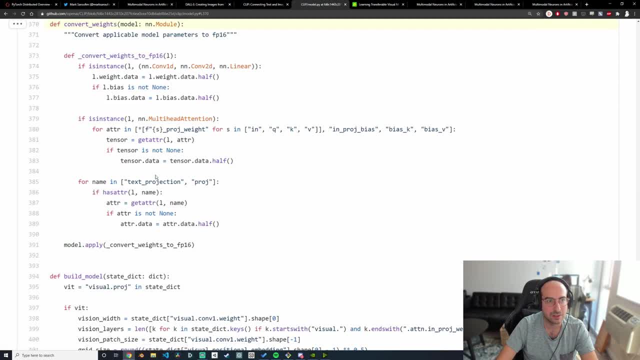 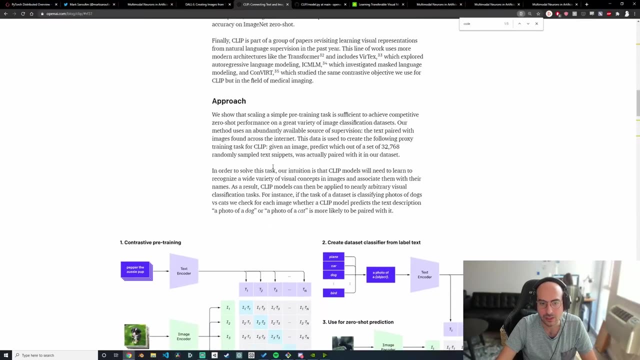 How does convert weights work? Okay, so just making sure that this conversion is happening. Okay, this is fine. So I think what I'll take away from this, let's just go back here. So we're gonna learn how to do a zero-shot classification. 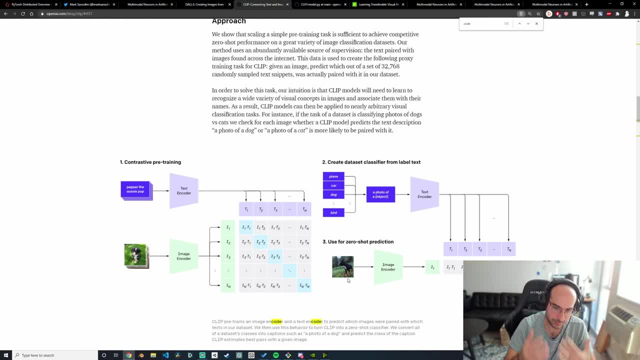 So we wanna classify for image classes that we've never seen, And the way we encode these image classes we've never seen is we have an image encoder that basically takes some text Like: basically you can use this, you can imagine, like maybe the ImageNet labels themselves. 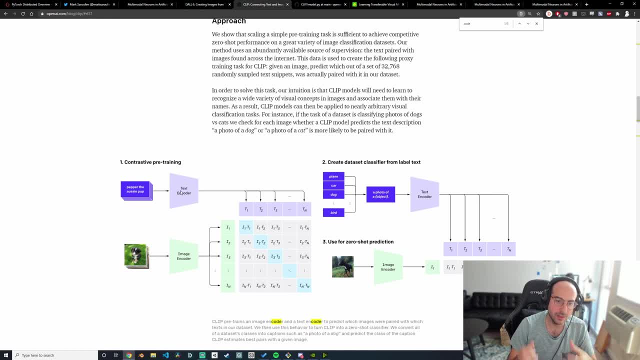 you encode them And then you take the image and you also encode it, And then you pass this to a vision transformer that needs to basically have some task that it needs to resolve. So this is the contrast of pre-training part. So this could literally be just predicting stuff. 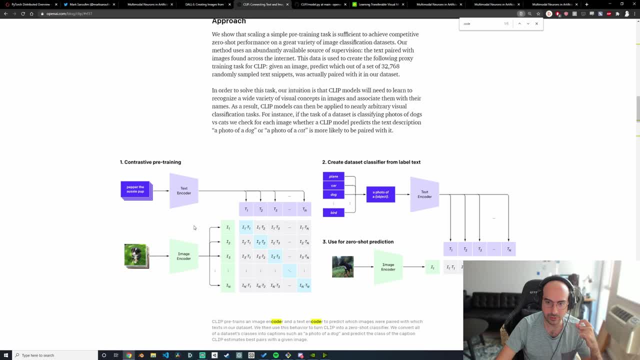 from ImageNet. And then the zero-shot part is: well, you have a new sentence that you create, You encode this new sentence and then you can say, well, like give me a photo of a dog. or like, let's say, given this dog, what's the text? 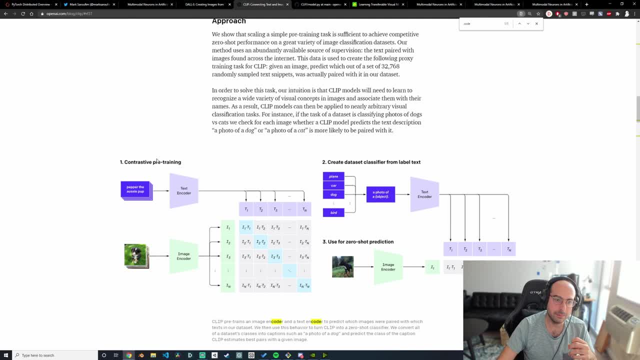 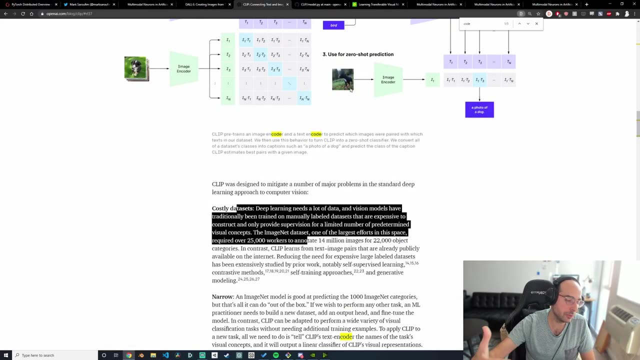 So this is where this becomes interesting. But this is like it's not exactly unsupervised in this case, like in the case of BERT, because you can use image pairs from existing labeled image data sets. But I guess the zero-shot part is for new things right. 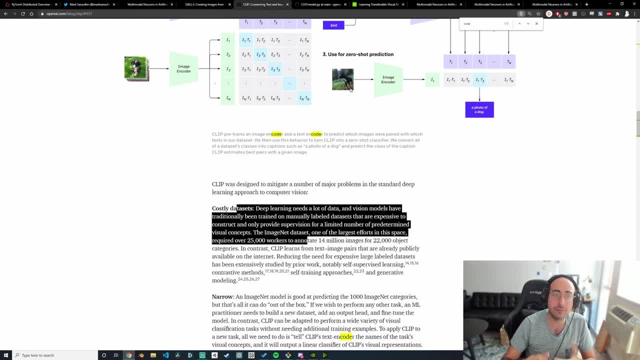 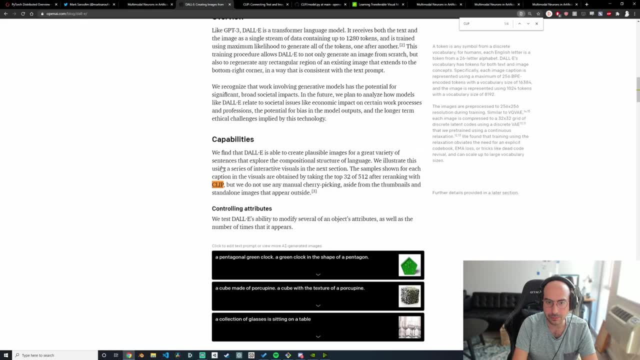 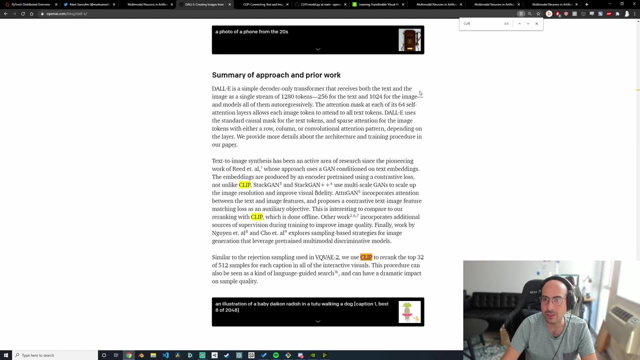 Like so for images, images that you haven't, for image classes that you haven't observed in your data set before. so i think the here they also mention uh clip in the dolly paper, right so is able to create plausible images. yeah, so, so clip is mentioned. what like four times here? 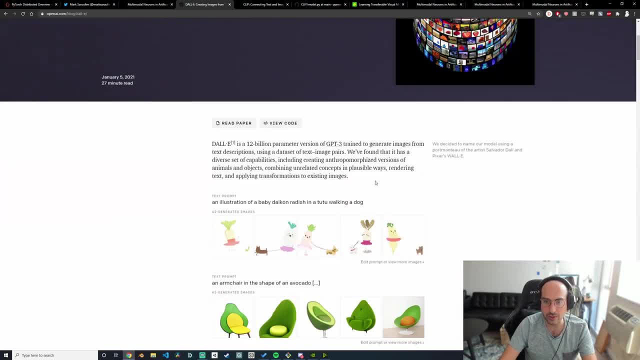 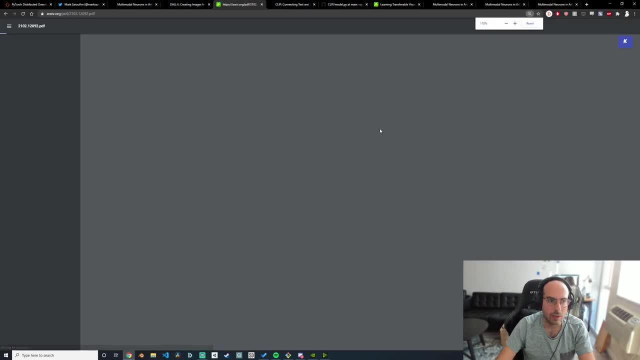 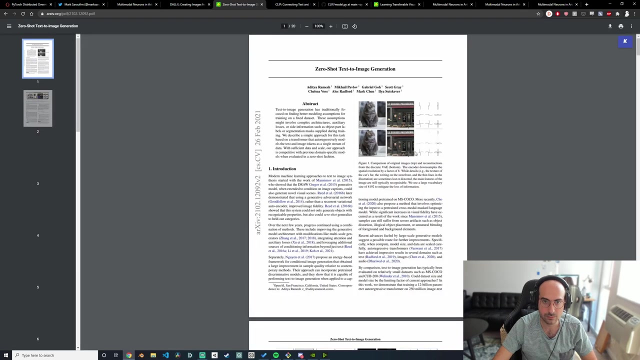 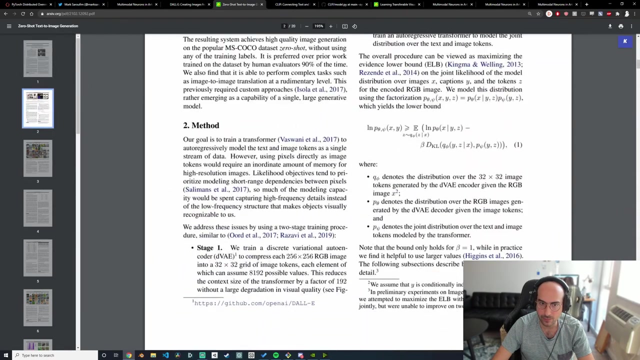 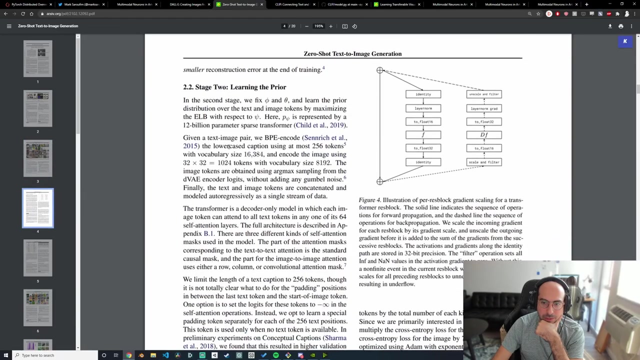 okay, but it's not actually using clip. so so with dolly, for example, you may have also recently seen this and it's usually, i believe, a similar idea. let's just, let's just go over the the paper again, okay. zero shot image generation: okay. so learn the visual cookbook, learn the prior. 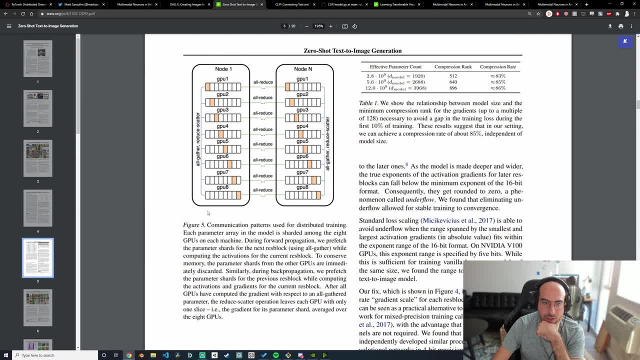 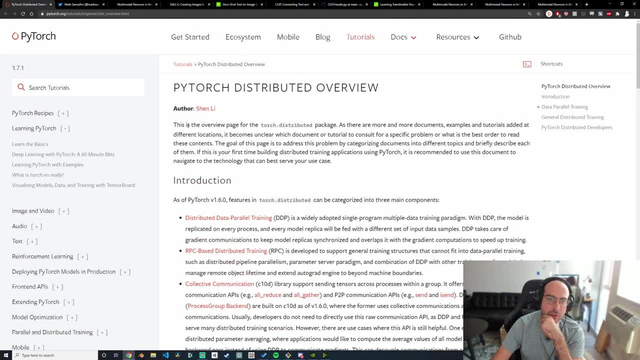 okay, so learn the visual cookbook, learn the prior. is there an architecture diagram for this thing? oh yeah, so on this whole point on distributed training, like the next video i've been very excited about doing is going over the like how distributed training actually works in pytorch. so i had a couple of videos on like model. 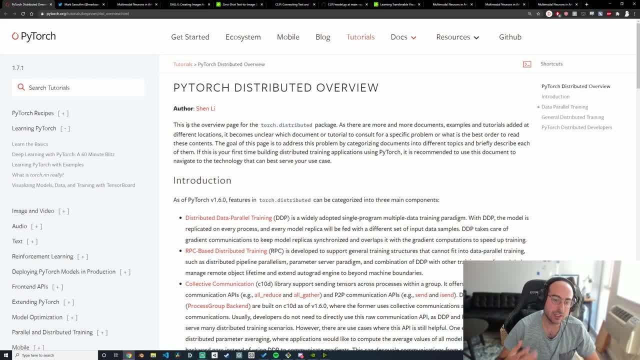 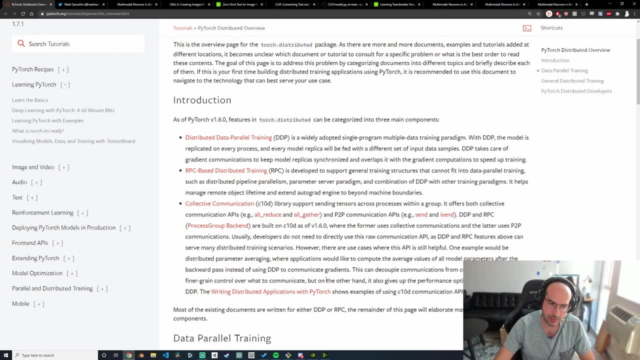 parallelism, data parallelism, pipeline parallelism, but i thought just like looking at some of the communication patterns, like, specifically, the all reduce and all gather libraries, would be really interesting. uh, so i should be doing that soon, probably. uh, this weekend most likely. so let me know if that's the case and i'll see you in the next video. 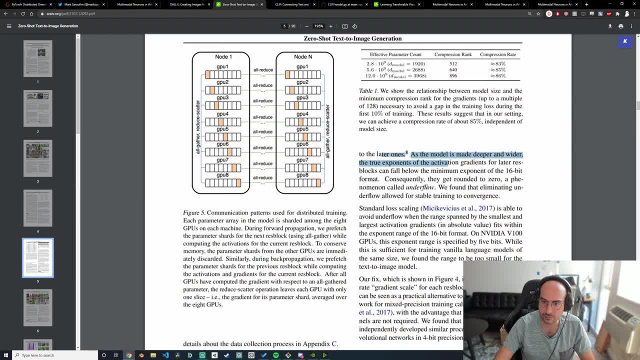 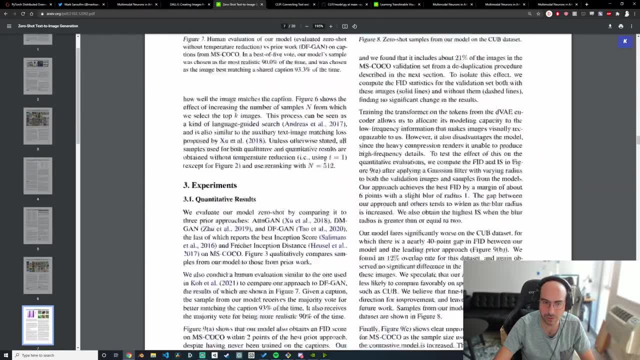 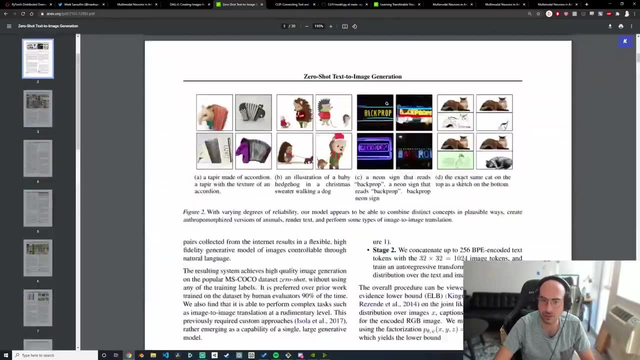 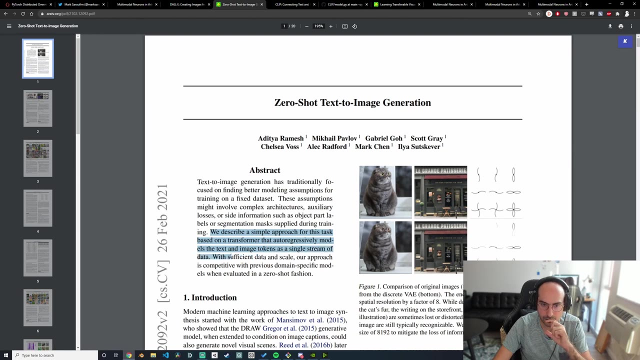 interesting. okay. mixed precision training- let's. yeah. so everyone's doing mixed precision training nowadays. it's very useful. you don't lose out all that much. i still want an architecture diagram. i don't see it that auto-regressively models the text and image tokens as a single stream of data. okay, sure, so i. think what they're doing is they're doing a lot of work on that. and they're doing a lot of work on that and they're doing a lot of work on the aesthetic orders that you're doing here. so you remember, you can mask uh text when you're doing stuff like for the. 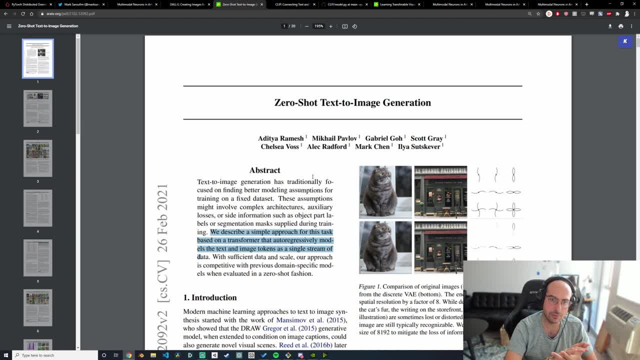 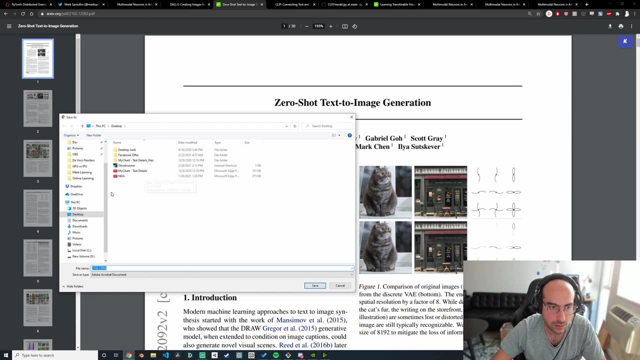 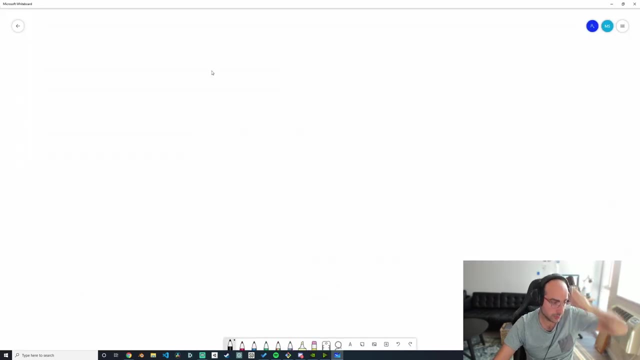 first問. yes, uh, I'll do it on Whiteboard, but it will be faster. so it's sort of a very similar idea like whereas. so it's sort of a very similar idea like: and stuff like seeingrato with already, uhOOOOO, start coding. 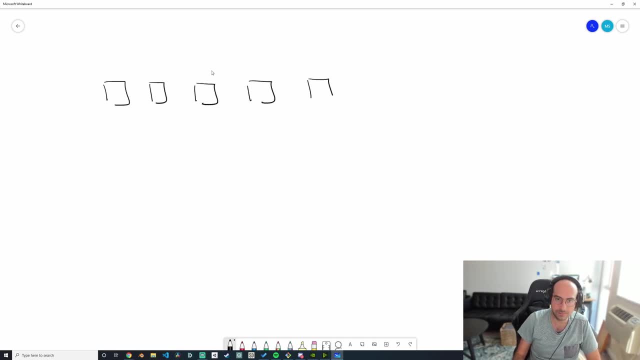 you're going to have like these. so this is your sentence, right, And each part of the sentence like this is a token, or, let's say, a word, And so what you do to learn in birth in an unsupervised way, is you essentially mask this. 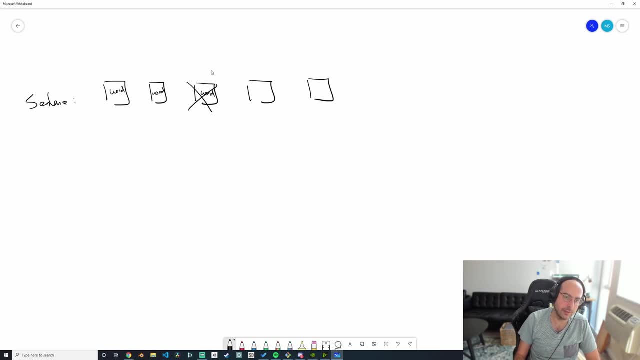 And then, basically, you pretend like you're not looking at it And then, given the surrounding context, like try to predict what this word is. Similarly, if you have an image, well, the image looks something like this. for example, let's say this image: 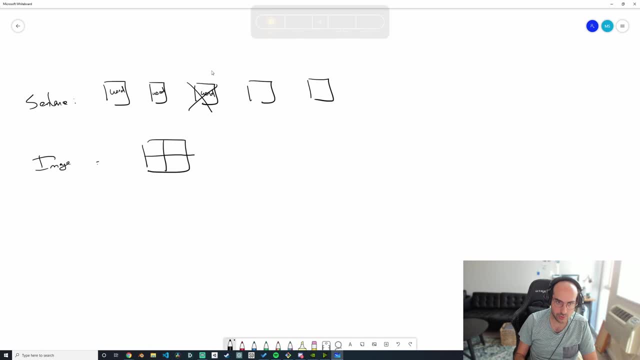 I mean, let's do a simple image for now. This is just like an image. So this is going to be a zero, zero. This is. this is one zero, This is a zero one, And then this is one one, right? So let's. 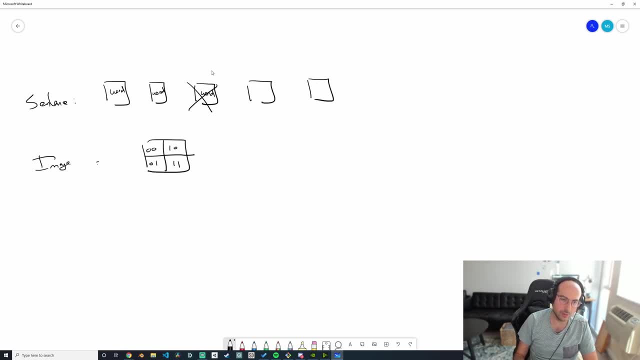 say: this is the. actually am I doing this? So I want row to be the first one. Yes, maybe I'll do this. One, zero, zero, one, and then one one, right. So what we're going to do is we're going to break apart this image into four sequences. 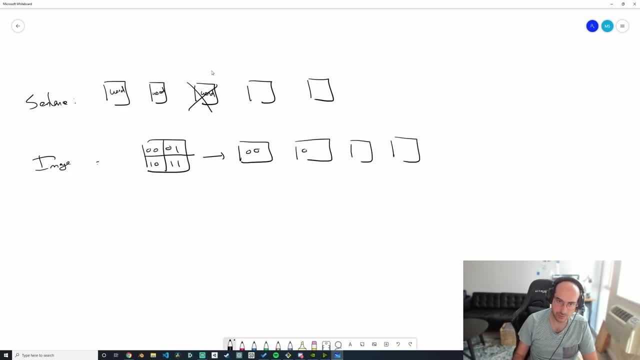 like this: So let's say zero, zero, zero, one, one, zero and one one. And we're going to do something very similar. We're going to pretend like we can't. take a look at this And given 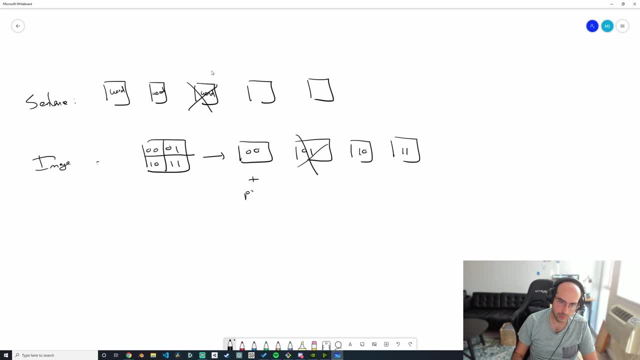 the surrounding context appended to the positional embedding for each one. we're going to predict what what this part is And this lets us build basically a, a, a vision, a transformer, in a completely unsupervised way. The interesting part of it and, I think, what they- 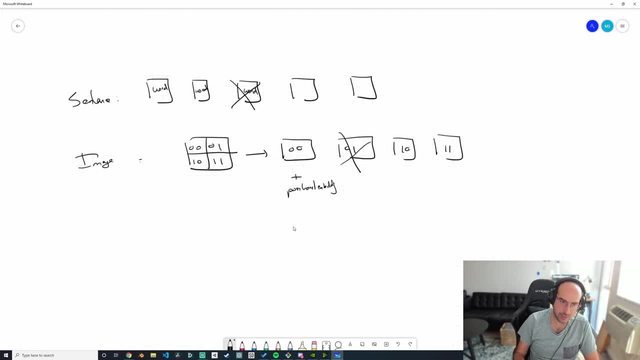 did in Dolly then is to say: well, I have image sentence pairs like right, So like image sentence pairs, and this could literally be like: like: basically, you know something, you can get this, like something like this from like ImageNet, And so what you do is you basically say: okay. 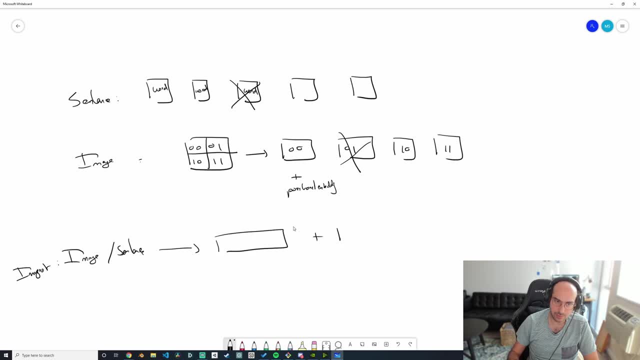 great, I'm going to append the sentence to the vision part. So this is the sentence, This is the image, And then do unsupervised pre-training on both. So it's a very powerful trick, but essentially this has been a recurring trend. 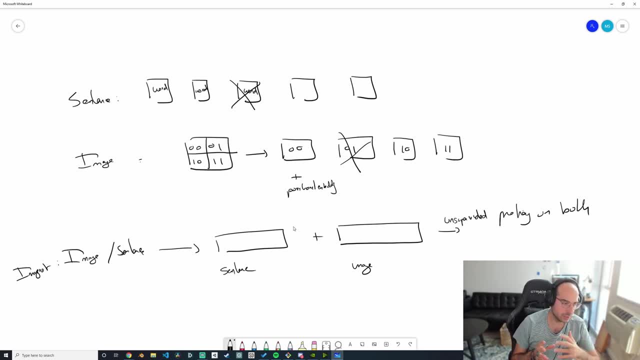 in machine learning, where anything that's supervised learning is easy. Anything that's not supervised learning is generally hard, And so a good way to make problems easy is to turn them into supervised learning problems. So this is exactly what this does. So again, so here for example, like this is, like, I believe, like sort of the main idea behind: 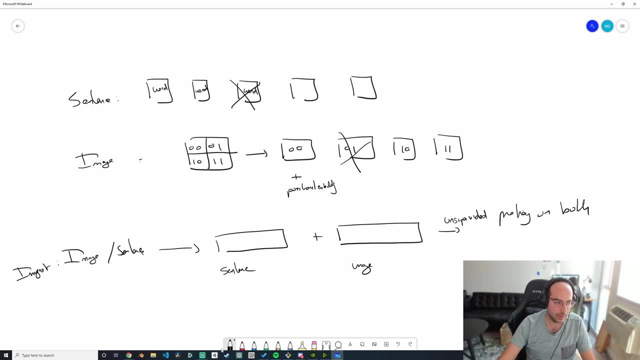 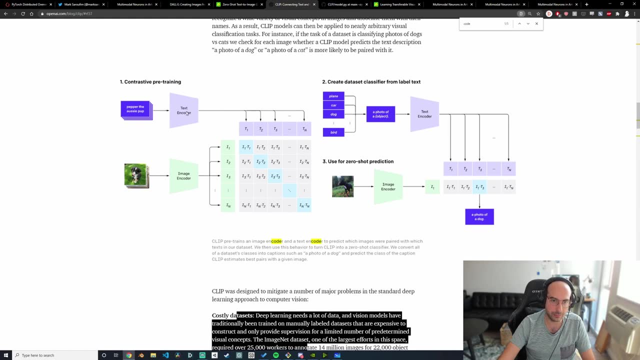 Dolly, I'm sure there's like a lot more tricks with the encoders and such, But if we were to look at a clip, for example, it's doing something very similar where it's coming up with a. it's not- it's not to say doing like this- unsupervised pre-training, but as you know, it is so it has. 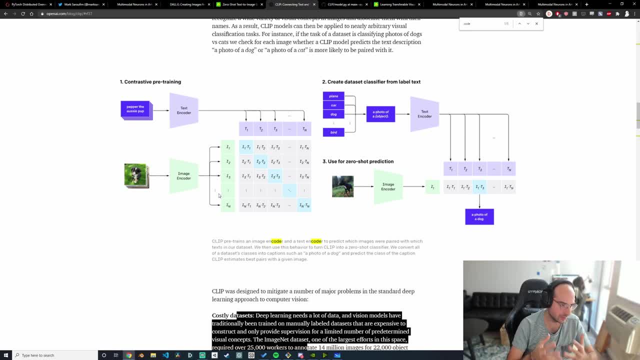 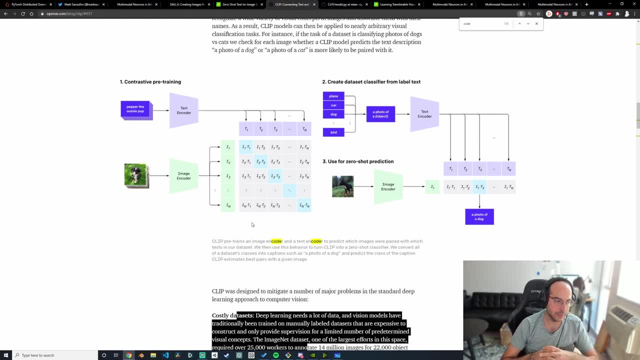 let's say, having two vectors, it turns it into this matrix And then you can basically train on this matrix on a class. So basically, given this matrix, add a linear layer at the very end of it, make some classification, and now you can pre-train this. And now this works for arbitrary images and 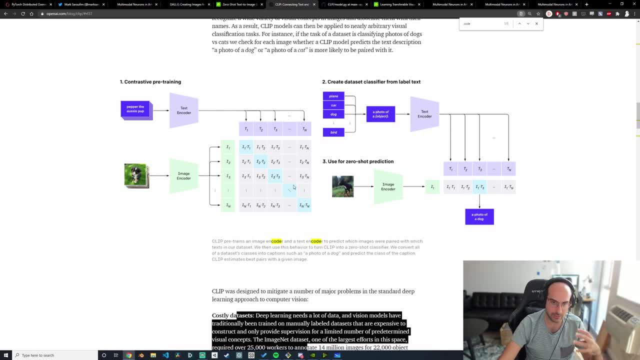 arbitrary classes as opposed to only working for a fixed number of classes. It was, like you know, absolutely very powerful And the nice thing about it is that, like well, when you're generating stuff, like you know, like like a linear layer is useful if you're doing a classification. 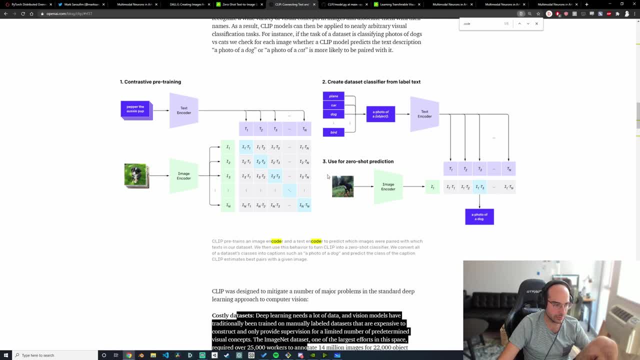 but if instead you make it like, let's say that you make it a linear layer and you make it a last part, here, for example, you can generate like sequences, you can generate images. So, again, depending on how you structure your output, you can either make this a generation, 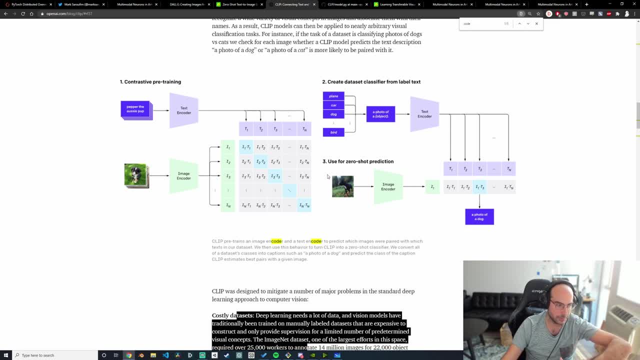 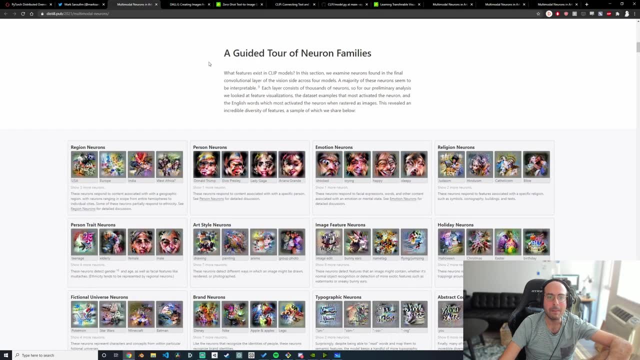 task, a regression task or a classification task? So it depends on what you're trying to do. So, okay, so all of this was was the background, And all of this was background to understand this new paper by about multimodal neurons, artificial neural networks, And I think what they're trying. 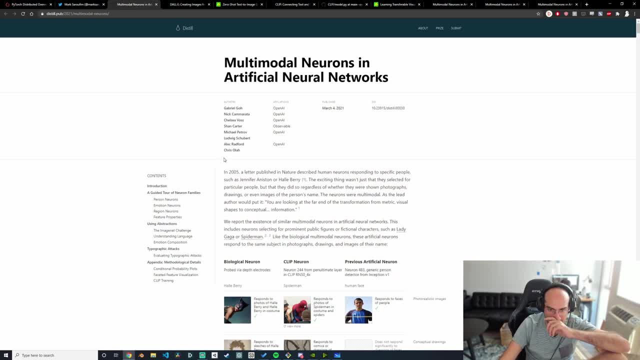 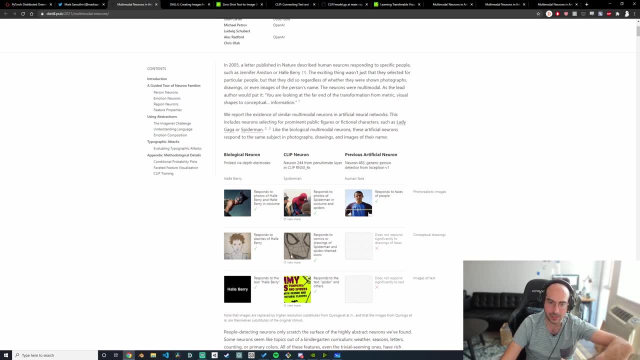 to do in this paper is try to get to the bottom of like: why does the clip work so well? So we already talked about like multimodal neurons and how you know we- we neurons recognize concepts and not just like specific pixels and shapes, And so they're saying like they find. 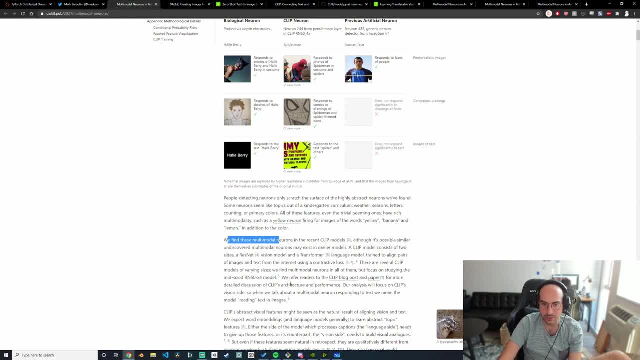 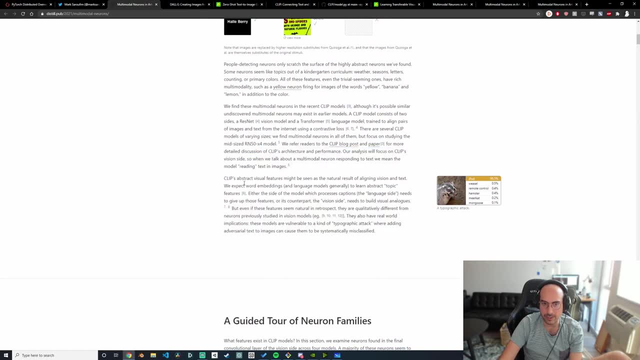 these multimodal neurons in in clip And so this is the okay. so they're saying we can refer you to the clip work if you're interested And clips. abstract visual features might be seen as a natural result of aligning vision and text And we expect world embeddings and language models generally to 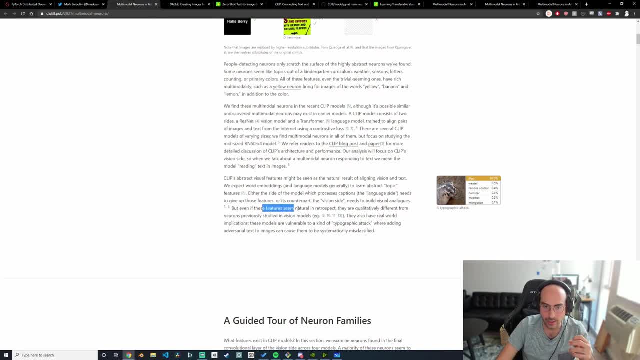 abstract topic features, And these features seem natural in retrospect. They're qualitatively different from neurons previously studied in vision models. They also have real world amplifications. These models are vulnerable to a kind of typographic attack, where adding adversarial text to images can cause them to be systematically misclassified. Okay, So let me just 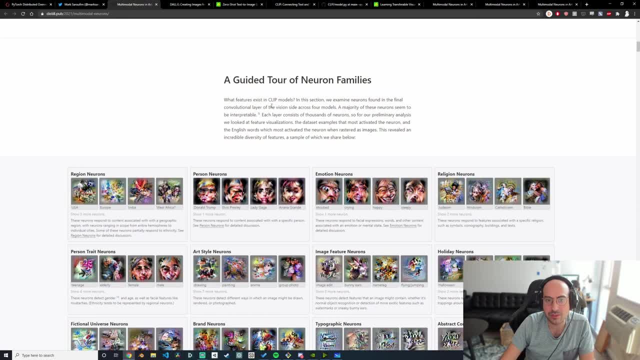 show you. let's see. We examined neurons found in the final convolution layer of the vision side across four models And a majority of these neurons seem to be interpretable, consist of thousands of neurons for our preliminary analysis. the English words which most activated neuron when rasterized images, And this revealed an incredible diversity. 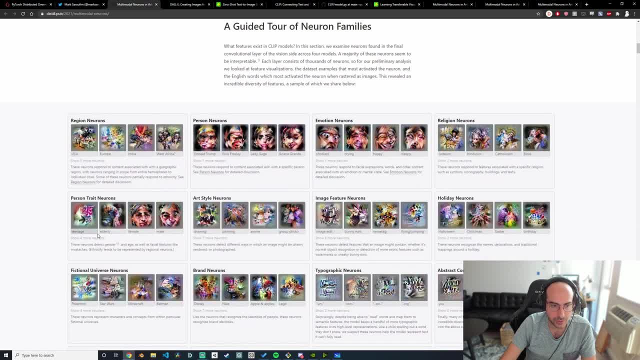 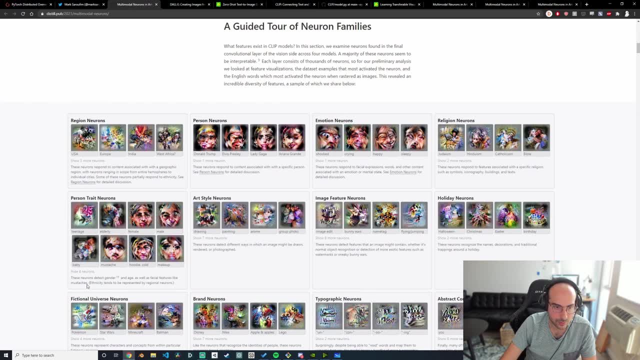 of features, a sample which we share below. So person trait neurons: Okay, So let's say, show four neurons, All right. So this is saying: okay, this is what, like an elderly neuron looks like a female neuron, a mustache neuron. I like it has mustaches on everything. 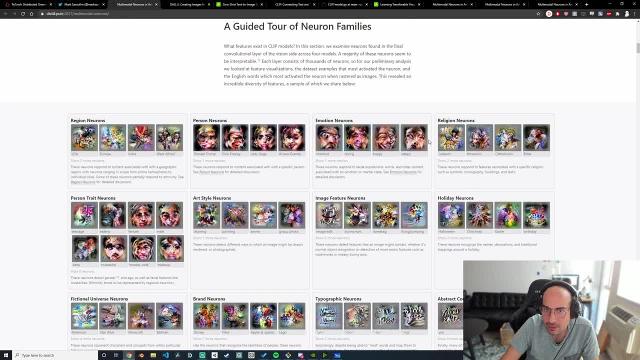 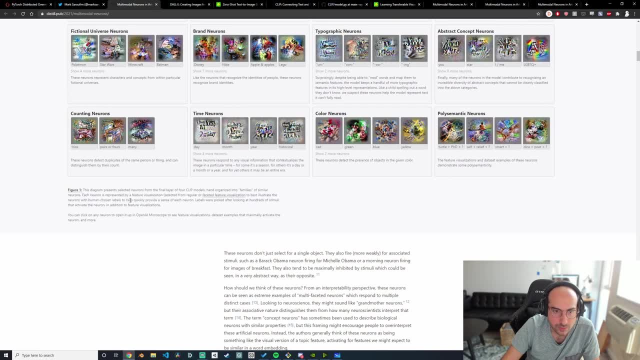 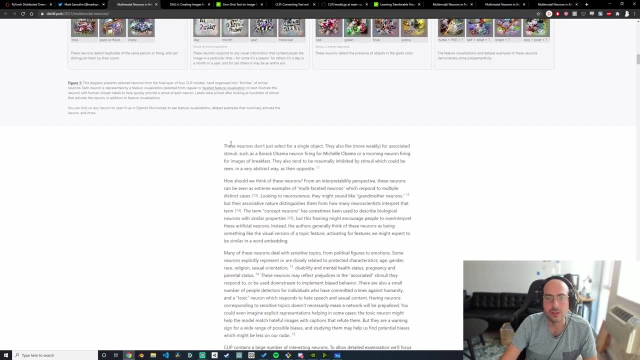 Bunny ears, happy, sleepy. Okay, Oh, interesting. So these neurons don't select for a single object. So, for example, if you look at, they also fire for weekly associated stimuli. So, for example, like this: Barack Obama is married to Michelle Obama. You expect these things to be, you know. 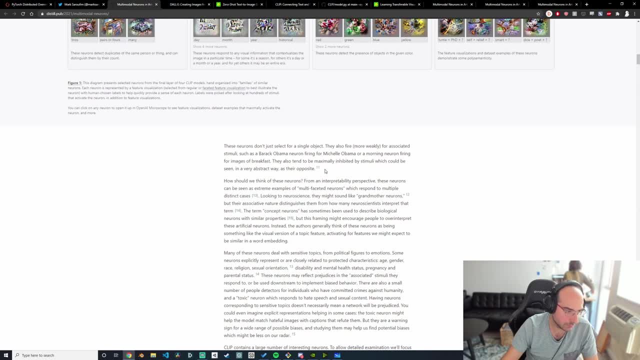 like Coke Co, stimulated Like the same same sorts of neurons should be involved in in recognizing these things. So they sound like her neuroscience, like all these grandmother neurons. What's a grandmother neuron? Okay, So it was just like neurons that respond to. 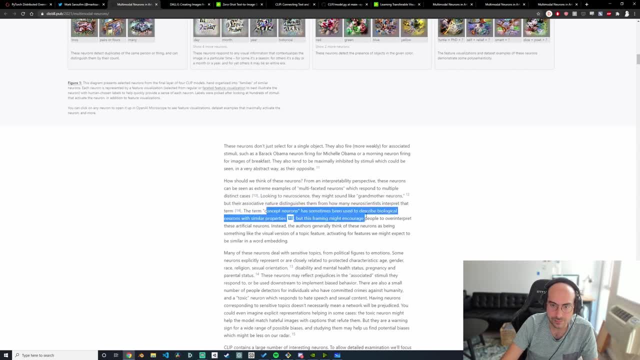 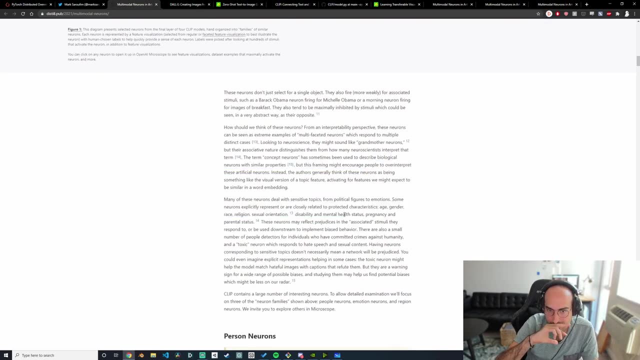 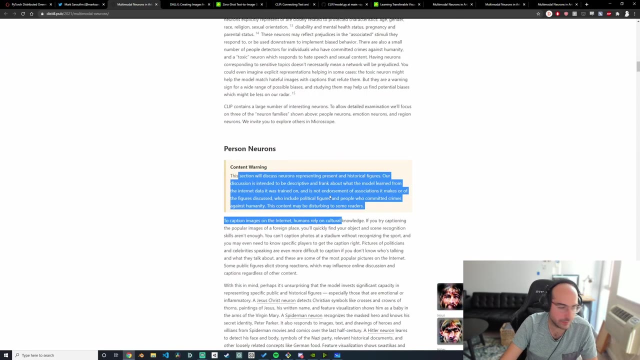 a specific stimulus. Okay, They also call them concept neurons. That's fine. I mean okay. so they're giving a content warning because i think a lot of the stuff may be biased like: let's see, so this is the what the hitler neuron. 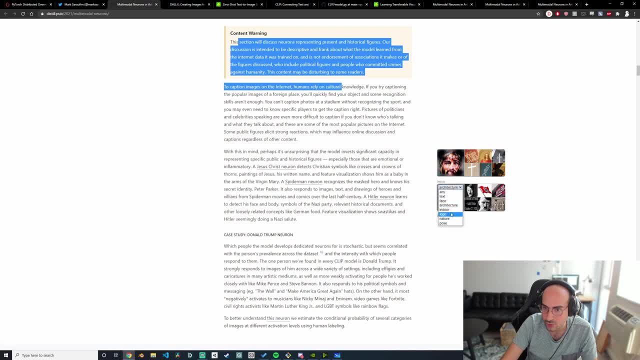 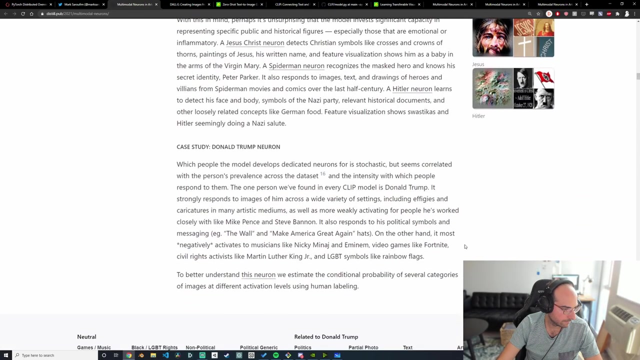 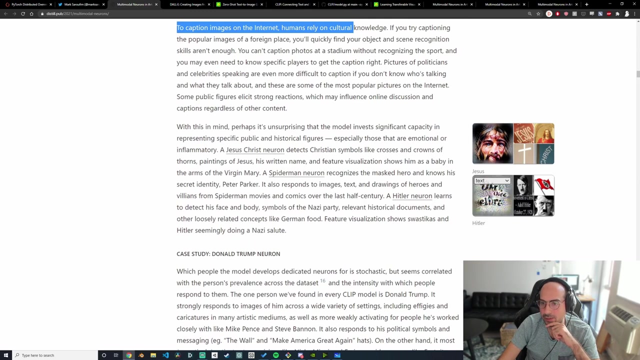 like german architecture with the logo. i know this logo is, oh, i see so so. so here, for example, i think what they're doing with this drop down here- let me zoom in a bit- so yes, so. so what they're doing with the neurons here is that they're showing you like the same. 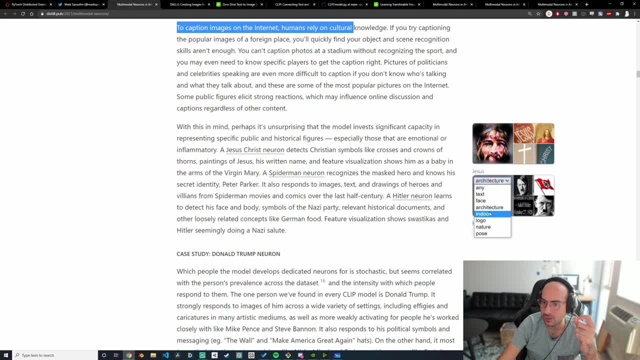 like, basically, if you change, like the, the nature of the thing, so that if it's indoor or if it's a logo or if it's a posture or whatever it's gonna, it's gonna show you the concepts it's related to. okay, so let's see. so they're saying we have a donald trump neuron. 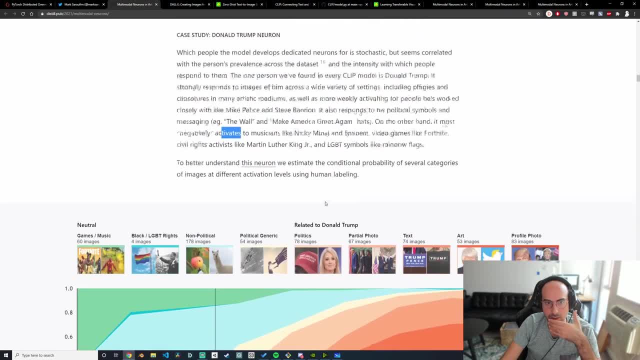 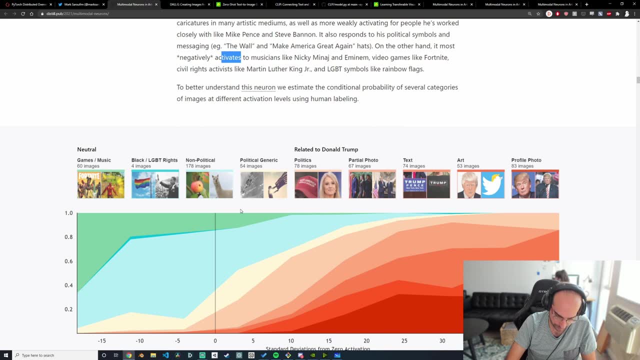 okay, what are they actually plotting here? i don't fully sorry, i think my pack is getting delivered okay. so, to better understand this neuron, we estimate the conditional probability of several categories of images at different activation levels using human labeling. conditional probability of several categories of images: oh so, games, given music, black given lgbt rights, non-political, generic. but what's the conditional? 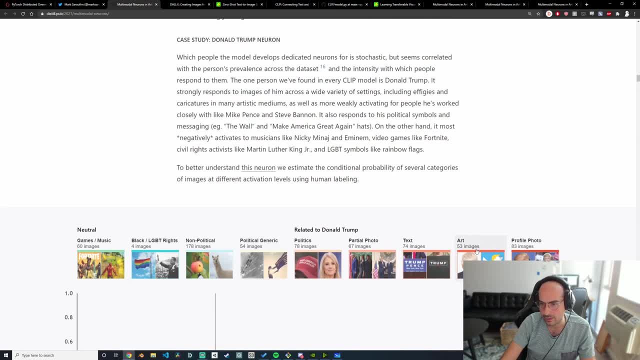 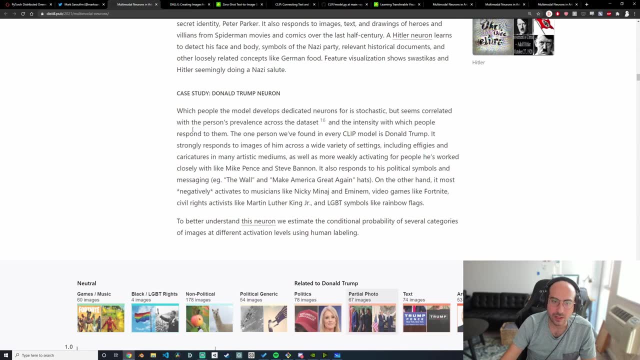 here. there's just one thing: is it trump, given twitter? it sounds so funny, okay, okay, let's just read this more carefully. so which people the model develops dedicated neurons for is stochastic, but seems correlated with the person's prevalence across the data set and the intensity with which people respond to them. the one person we found in every clip model. 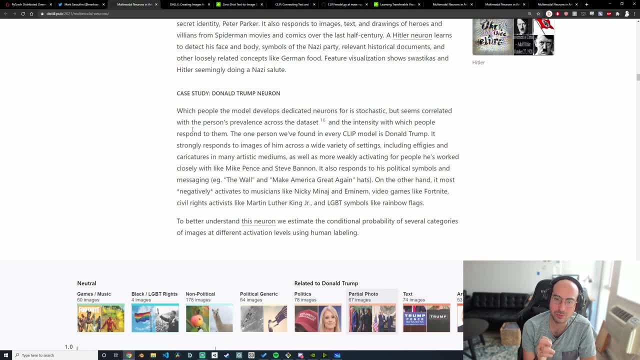 is donald trump. it strongly responds to images of him across a wide variety of settings, including effigies and caricatures in many artistic mediums, as well as more weakly activating- activating for people he's worked closely with, like mike vance and steve bannon. 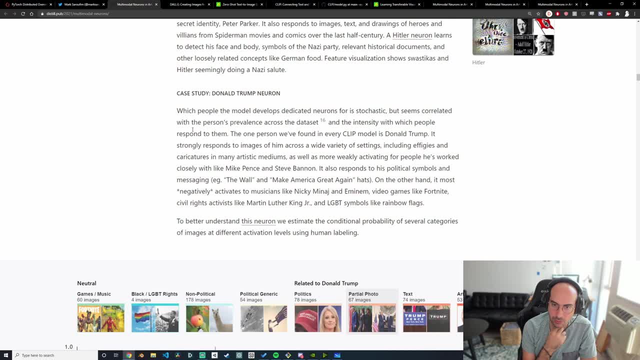 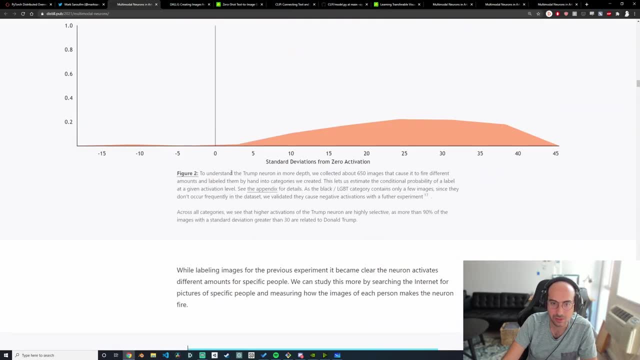 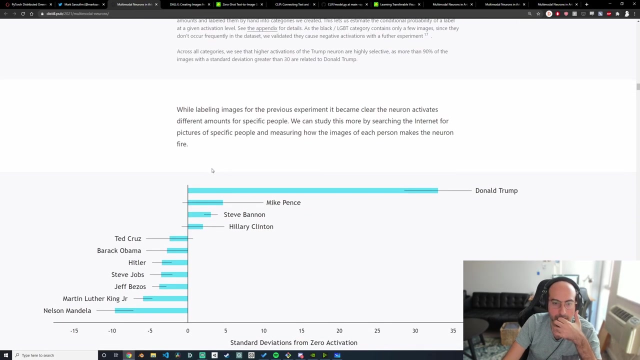 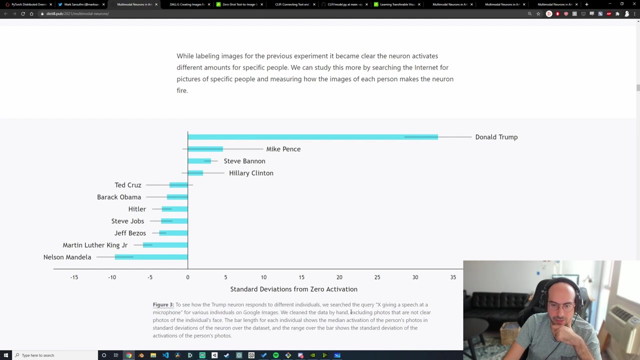 it also responds to his political symbols and messaging, like the wall make america great and, on the other hand, it most negatively activates the musicians like nikki minaj and eminem. okay, if we search the query x given x giving a speech at the microphone for various individuals on google, 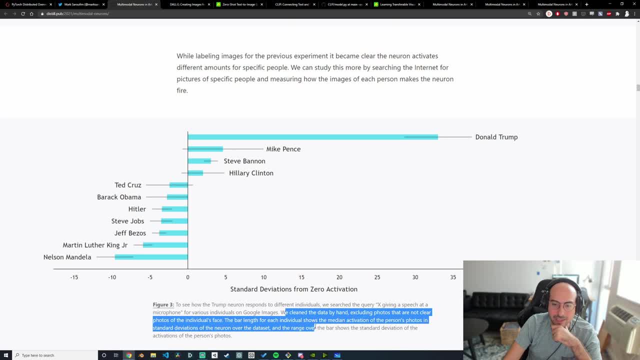 images, the median activation of the person's photo and the standard deviation of the neurons over the data set. oh, interesting, i see what they're doing. so if you know that certain neurons activate certain concepts, uh, now you can basically count for how many such images in the data set. 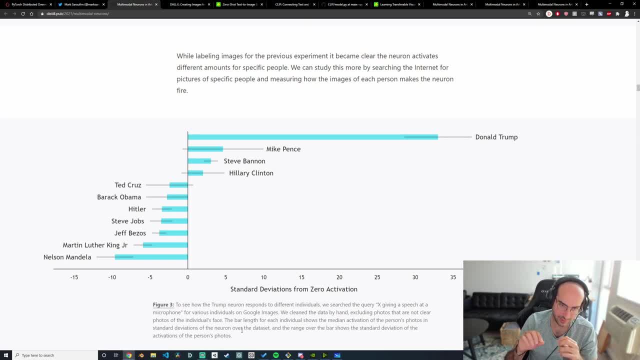 does this line of text uh activate for? and this gives you like an idea. it's interesting. it's sort of like image search, almost like it's built in um, this is a very interesting trick actually and i like it because, like traditionally, like when you're searching the stuff like you could like. 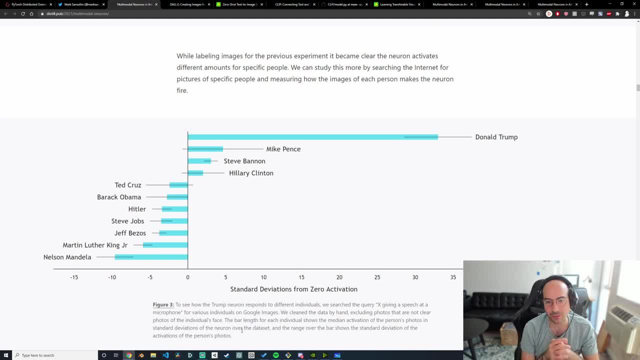 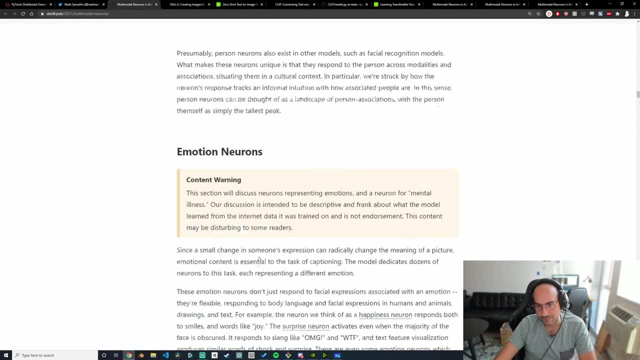 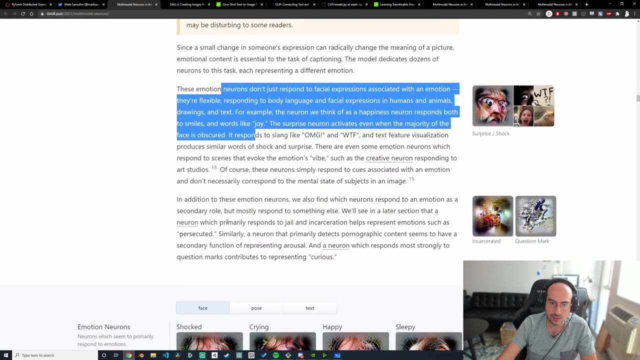 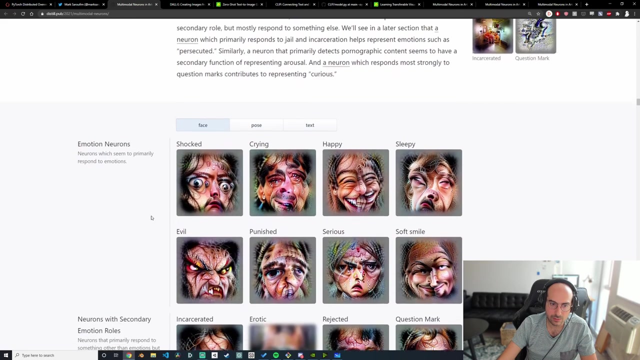 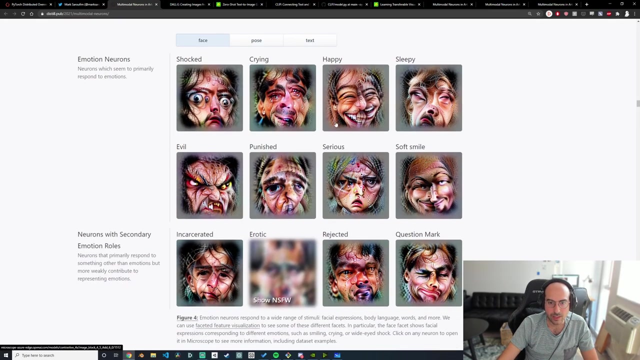 label the best examples or the worst examples, but this sort of gives a more systematic way of dealing with these things, where you have like a natural language api to think through these problems. okay, so we have emotion neurons. okay, evil punish. i wonder if it's me just like over analyzing here, but it does feel like the images have like 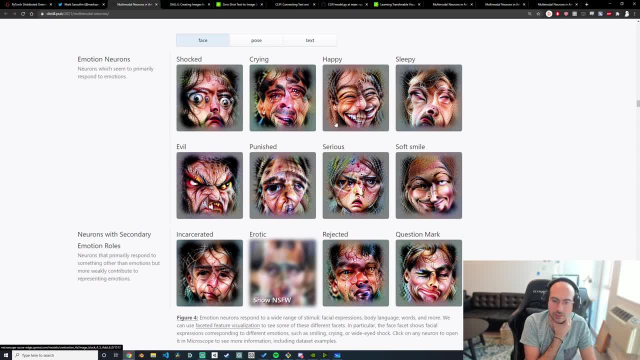 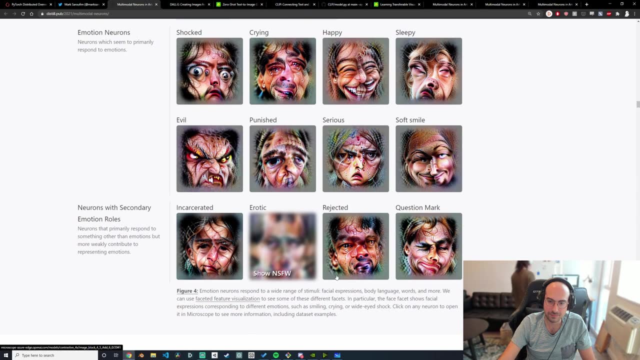 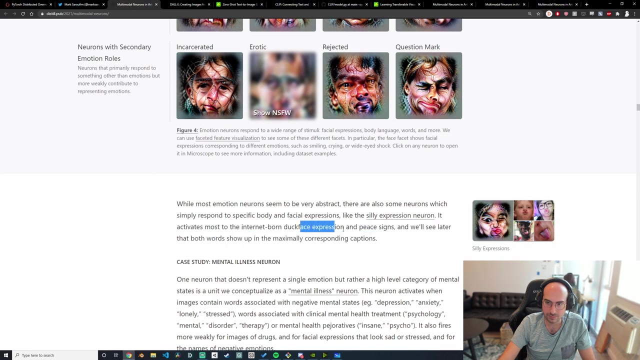 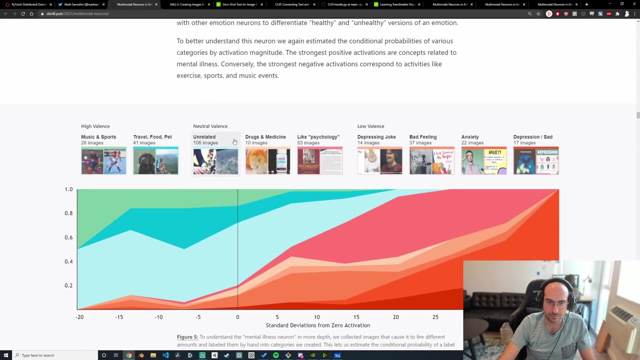 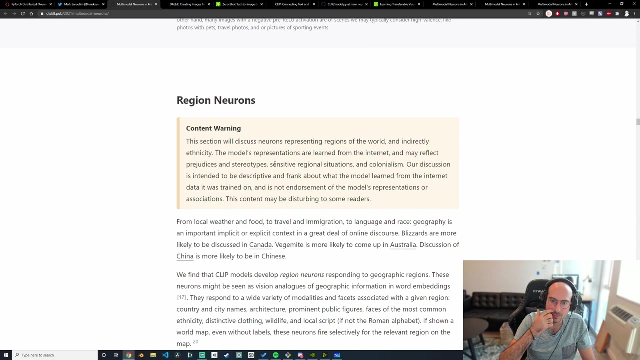 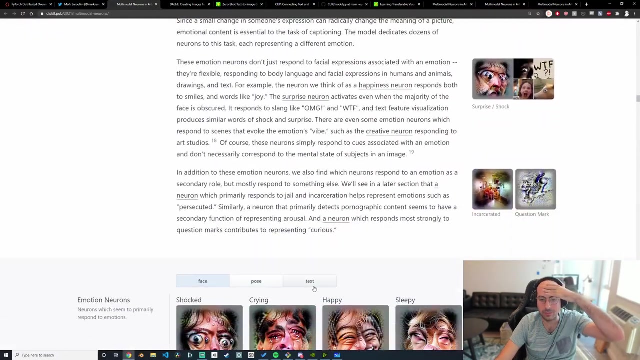 a striking similarity to each other. look very similar. it's almost like the same face. evil one is like intense, actually dragon and stuff like a scale, right incarcerated, figured out like a bar pattern. it's interesting, okay. so i think like basically given this natural language api to the search through concepts. 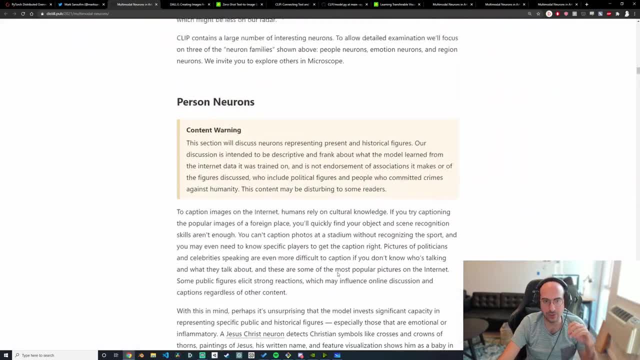 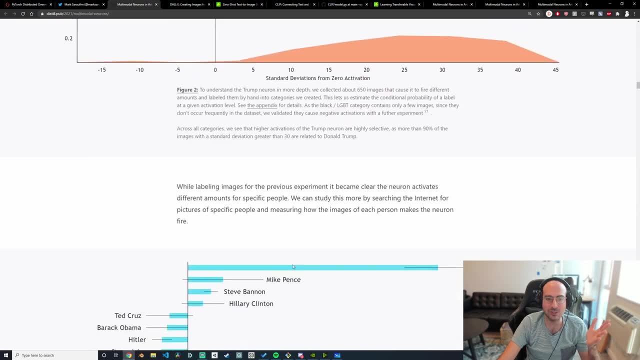 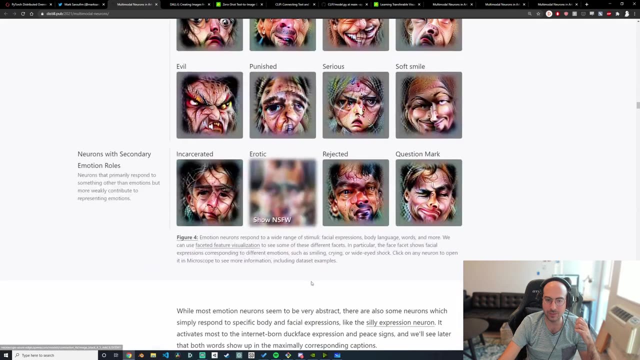 they split it up into first looking at the images and then looking at the images and then looking at people. it looks like trump is by far the most triggering person and uh, probably like in history at this point then with emotion neurons. and then looking: uh like you can get, uh like you. 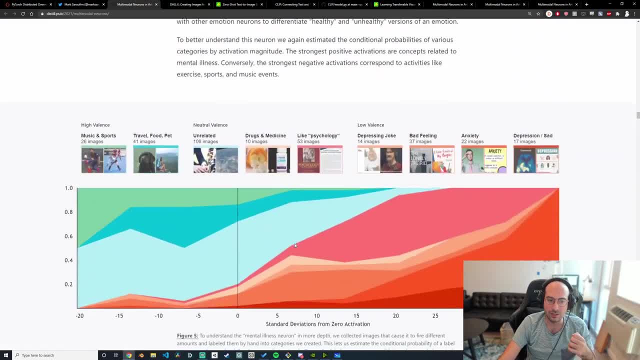 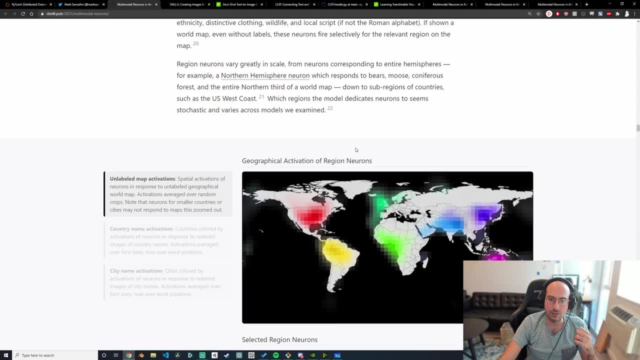 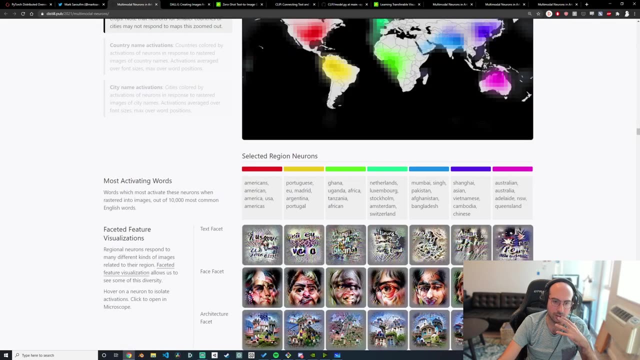 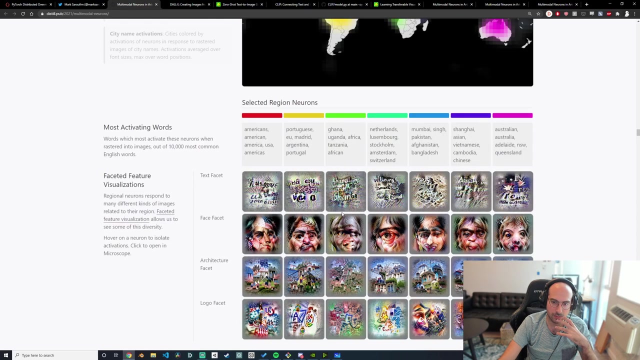 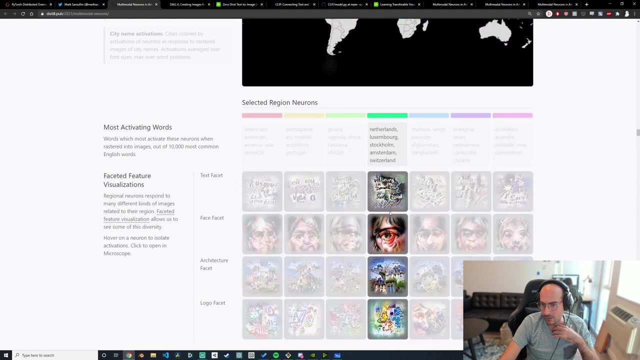 can get relevant activations in this way. um, let's see here. so then we have these region neurons. how does this work exactly? oh, this is a visualization, i think, kind of hard to say what's going on here. i think the america one is pretty funny here with all the usa flags. i think the holland one certainly this feels. 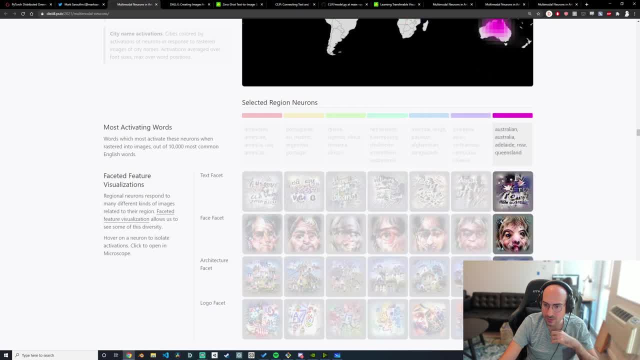 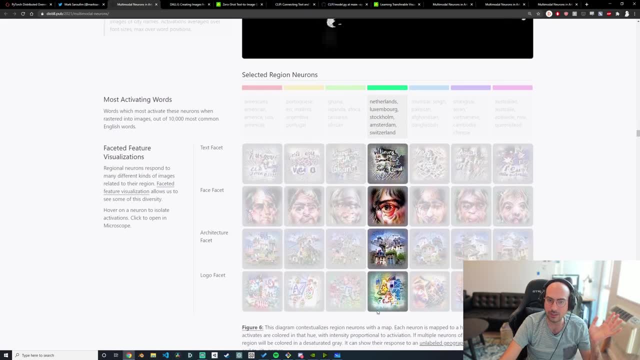 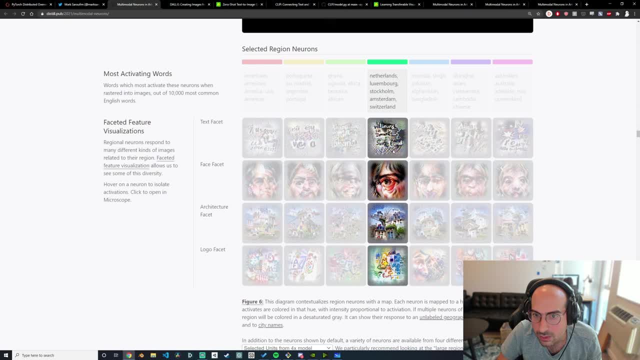 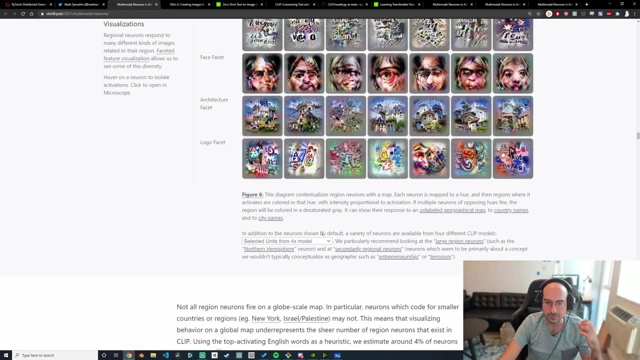 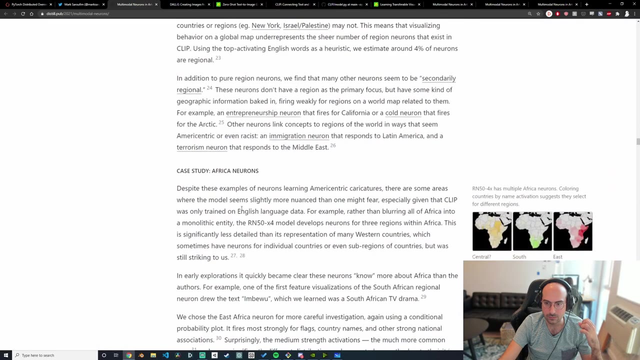 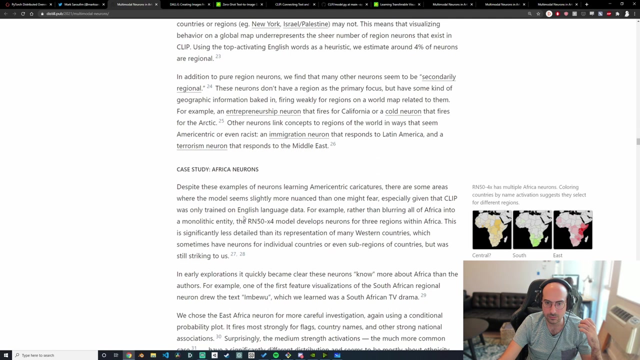 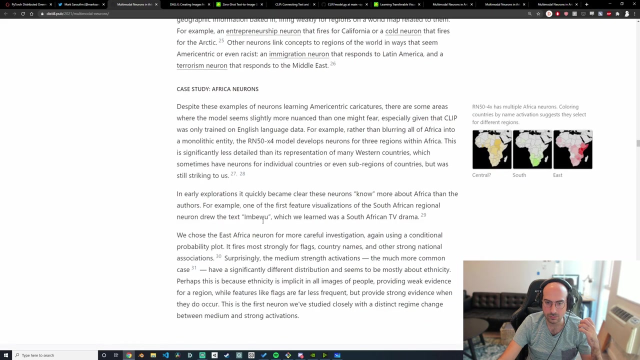 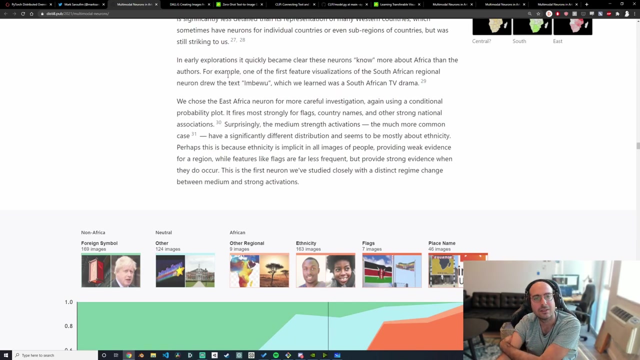 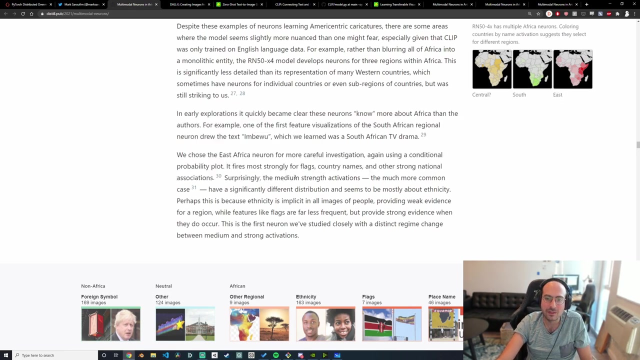 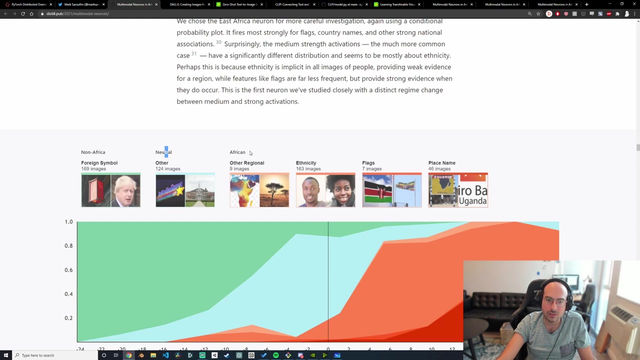 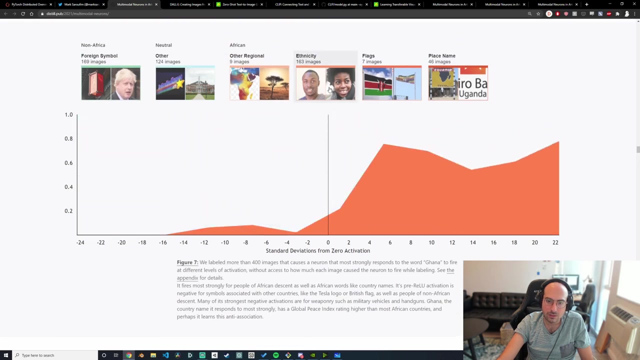 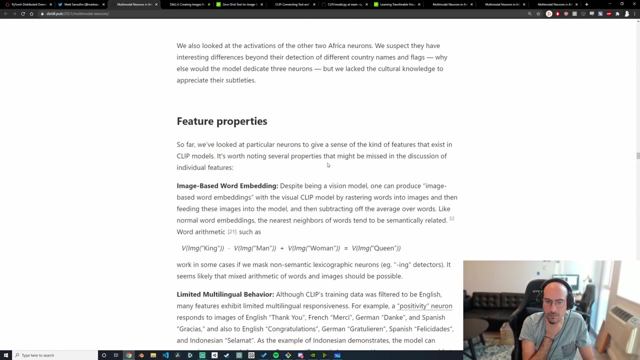 alfonsino la reyna. this is what the Oh interesting And I guess like, yeah, I mean, yeah, it makes sense that the model knows more, but the users don't Interesting This is interesting. So they bring back some of these ideas from the original Word2Vec paper, which is like arithmetic on images. 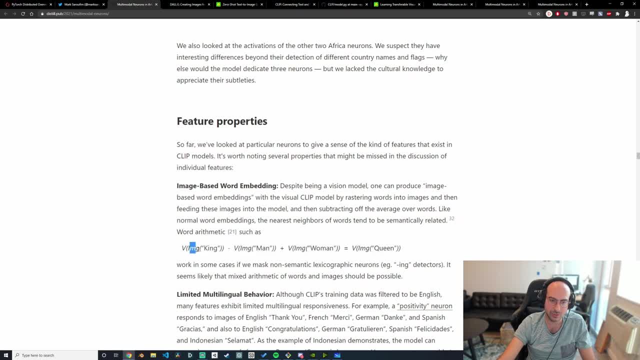 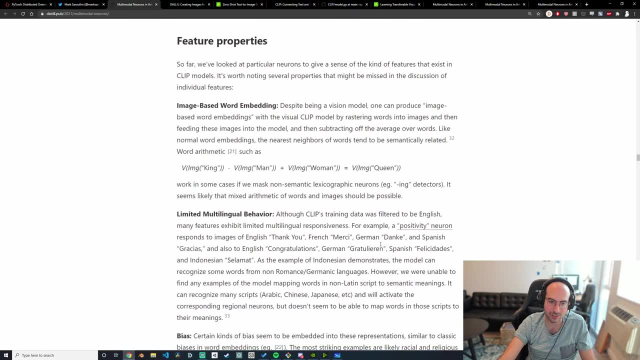 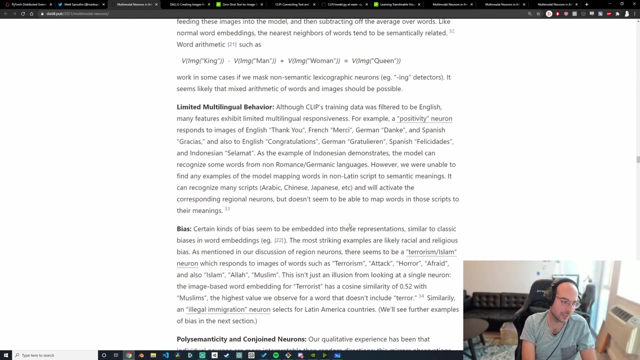 So you can basically do a search like: OK, well, give me an image of a king and then take the encoding of that And this should be like relatively close. This is very interesting, OK. I like this because it's like, instead of just working over text like now, you have this new modality that you can work with in an arithmetic way. 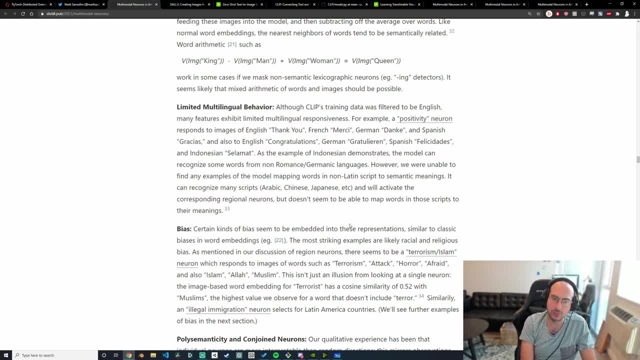 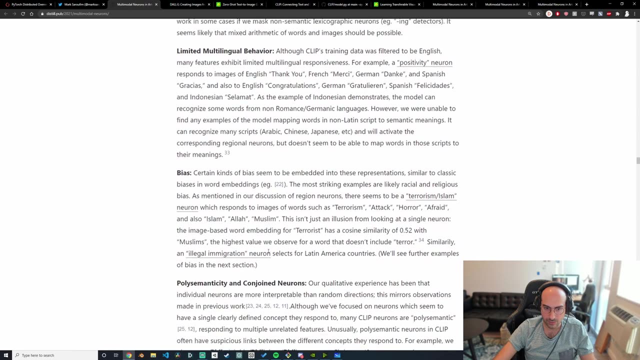 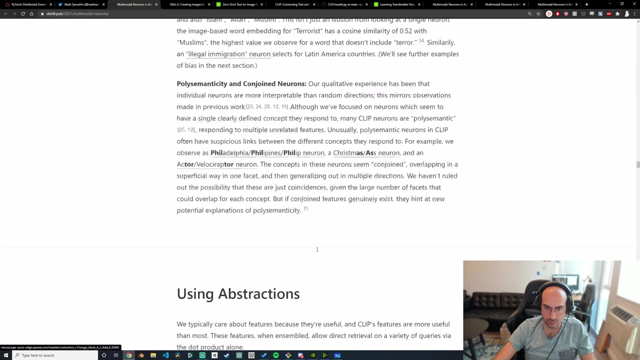 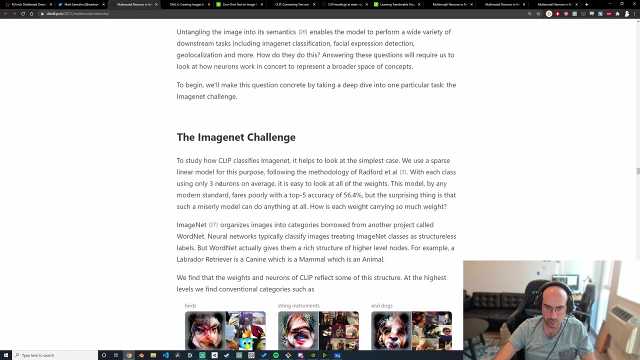 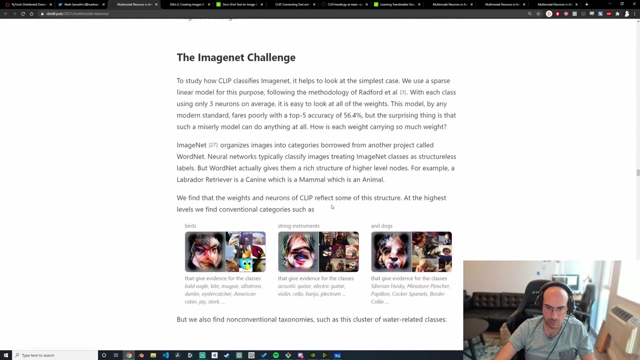 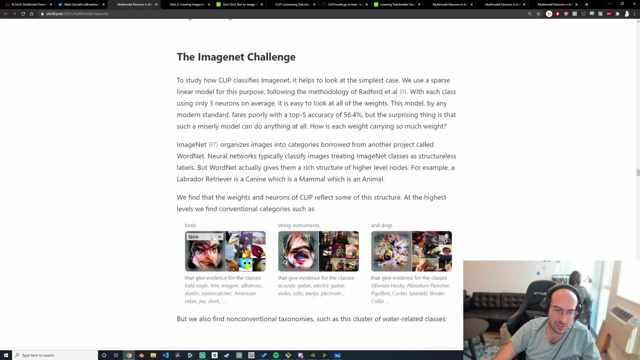 Although I do remember there were lots of criticisms about this word, embedding arithmetic and whether it actually generalizes. I think I saw a lot of work saying it does not. But just something to keep in mind. I'm surprised like the author is going to make anything out of like looking at these images. 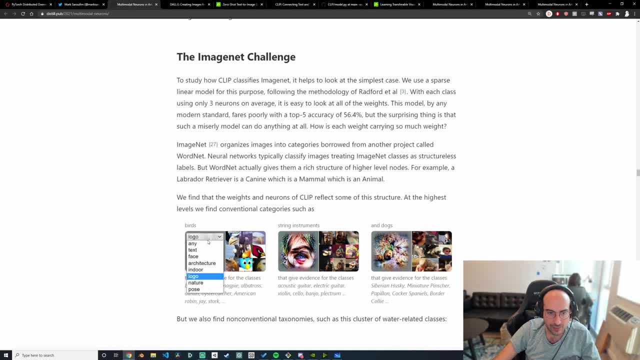 I don't know, I'm just saying eagle though, right, And this kind of looks like a human bird. This is really weird. I don't get the architecture. It's like bird memorabilia. This is very, very bizarre images. 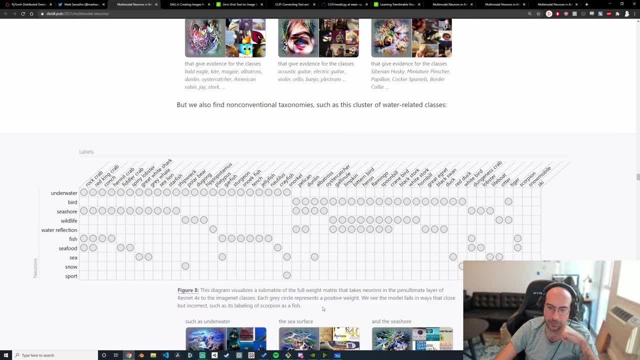 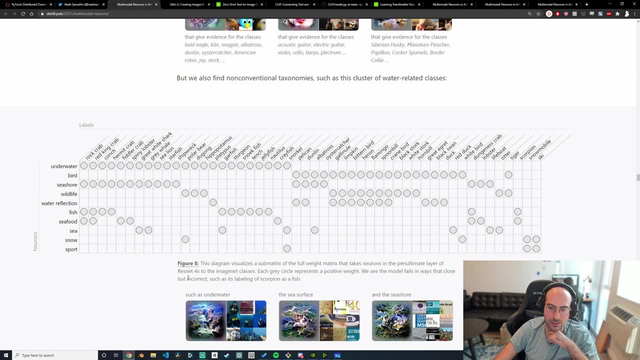 So this is how I can visualize the full weight. This is a matrix that takes neurons in the penultimate layer of resonant force of the image net class and each gray circle represents a positive weight and we see the model fails in ways that close but incorrect, such as this labeling of scorpion as a fish. 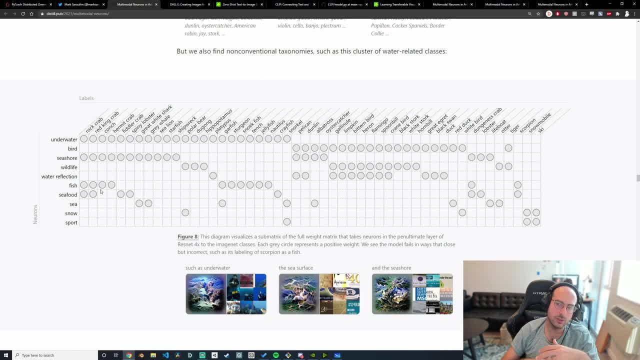 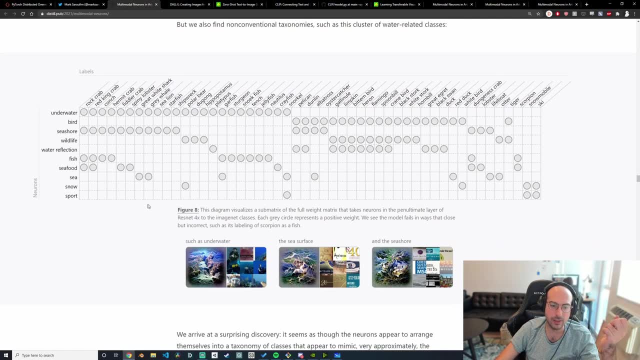 Oh, interesting. So once you recognize certain neurons, you can see on which kinds of images they get classified, and then look at the diff. This looks like it's qualitative, though like I think these neurons would be qualitatively generated, if I'm not mistaken. 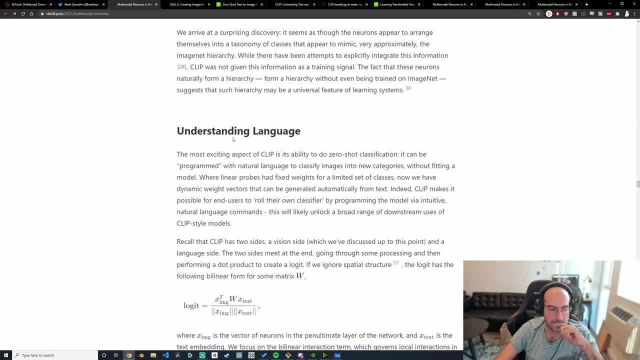 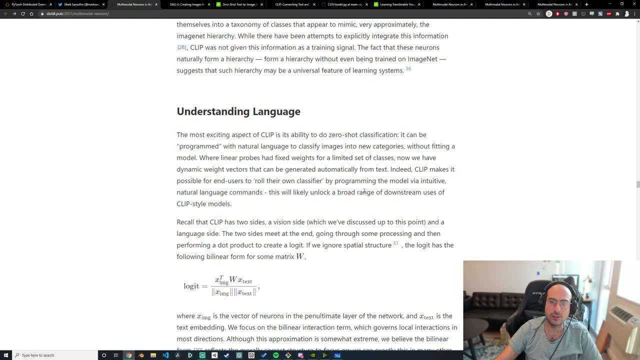 Yeah, I'm almost done, so don't worry about it. All right, So what CLIP also does is it does zero-shot classification. Okay, so we talked about this. So CLIP has two sides, a vision side and a language side, and they meet at the end going through some processing and then performing a dot product to create a logit. if we ignore spatial structure, 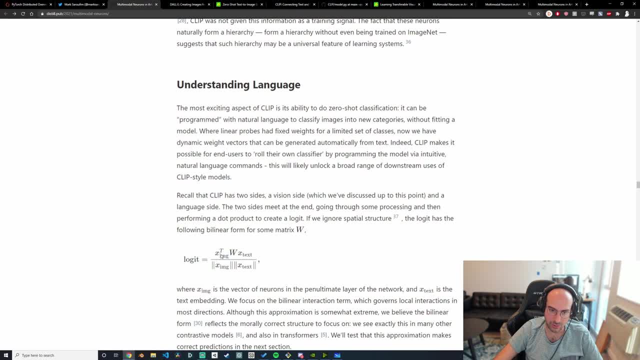 And the logit has this form. So we take the image. Oh yeah, I mean, it's like, yeah, like the image times the weight matrix times the text divided by the norm of the image and the text. It's like that, you know, almost like 1.. 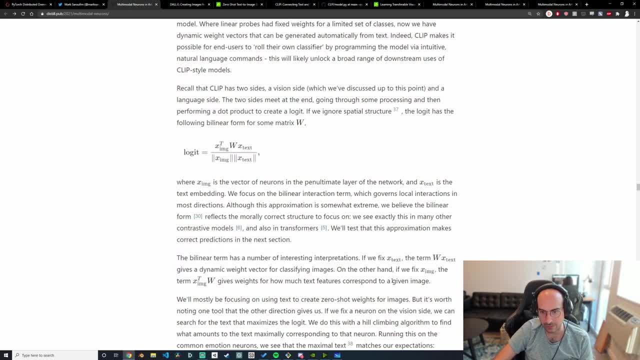 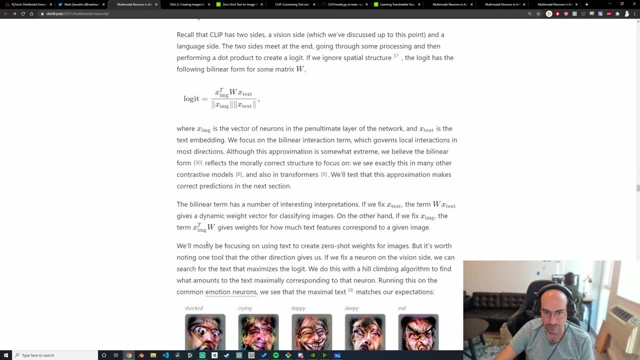 So the bilinear term has a number of interesting interpretations. If we fix one of them, the WXX, the dynamic weight vector for classifying images, Okay, If we fix the neuron on the vision side, we can search for the text that maximizes the logit. if we do this hillclimbing algorithm to find what amounts to the text maximally corresponding to that neuron. 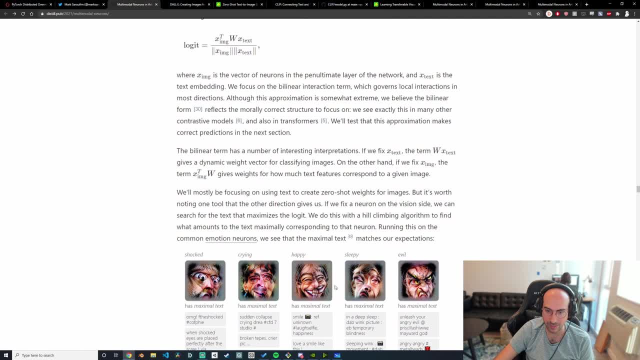 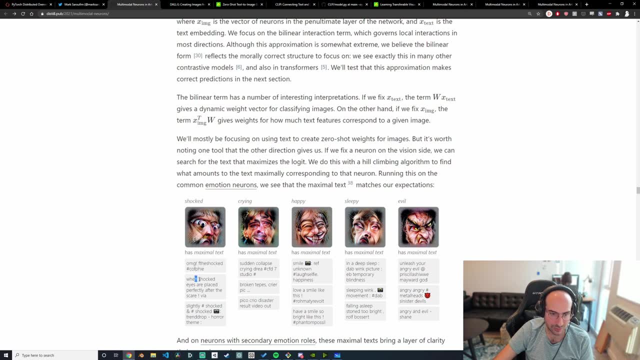 And we can run this on a common in emotion neurons. We can see that the maxual text And we can see that there is a 1. That's what we're trying to do there right- matches up to our expectations. Oh my God, the shocked eyes are perfectly placed. 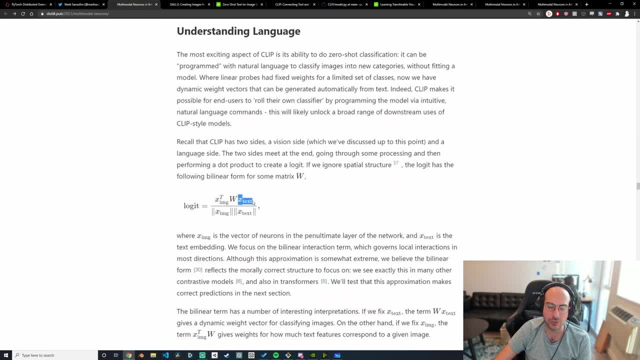 This is interesting actually. So remember, like we're doing a form of search right, Like, given certain concept neurons, we either fix the text or an image and then we can search for the neurons that most highly activate either that text or that image. 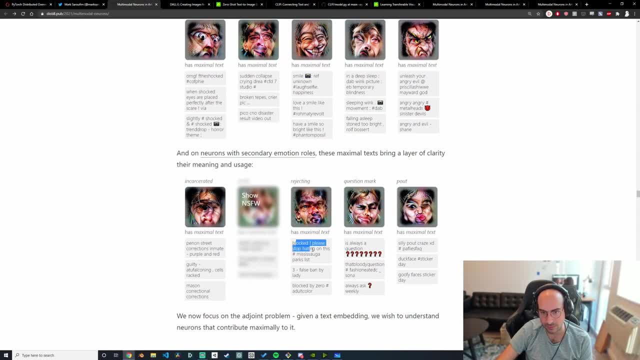 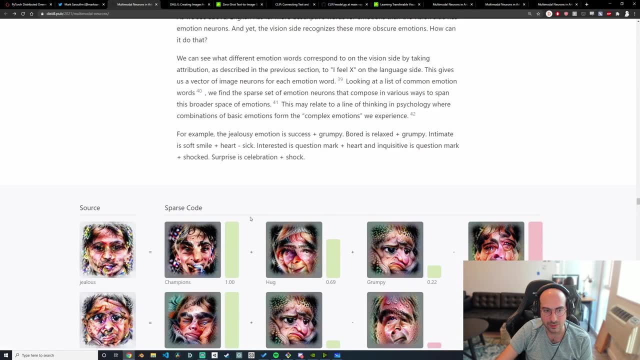 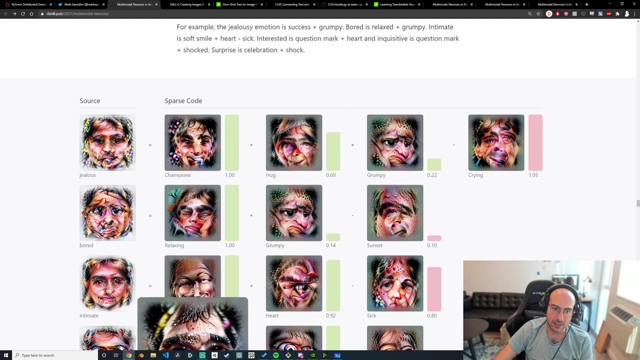 So I think they're gonna be using the same idea. Please stop hating on me. False band, okay. So emotion composition, interesting, So relaxing, plus grumpy. sunset is bored. Oh, that's interesting, Yeah, like the negative version of minus sunset, I see. 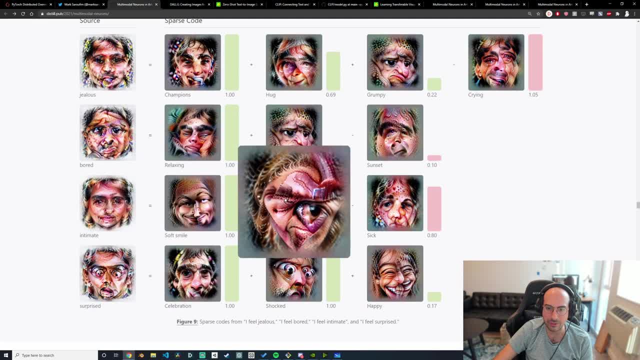 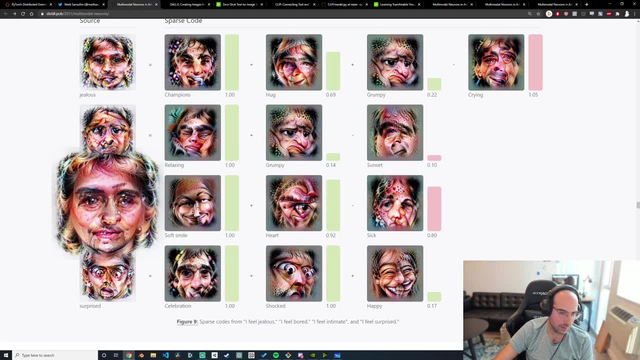 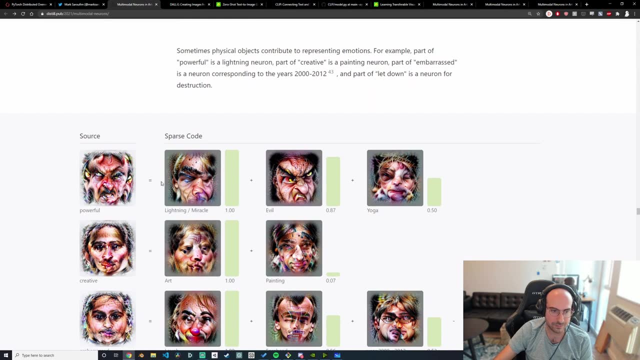 Intimate. if you take a soft smile with a heart and you remove sickness, then you get intimate. Yeah, I don't know, but these don't make too much sense to me. So lightning, miracle and evil plus yoga gives you powerful. 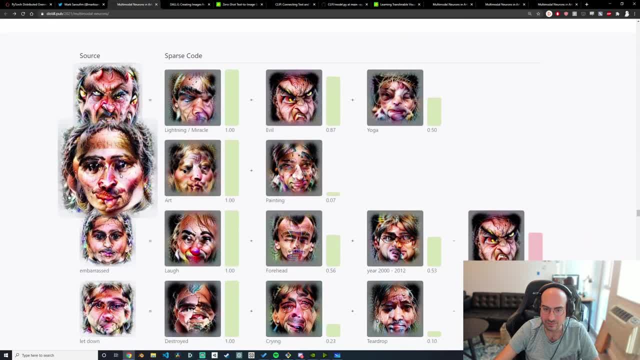 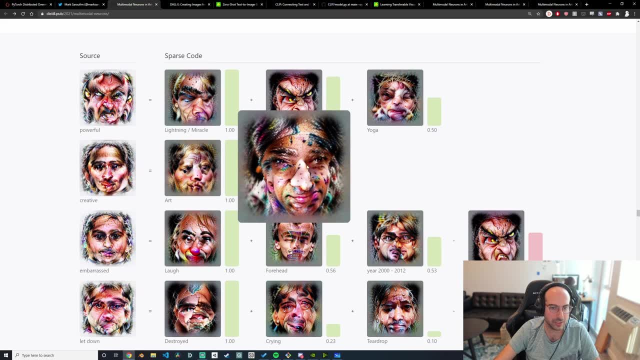 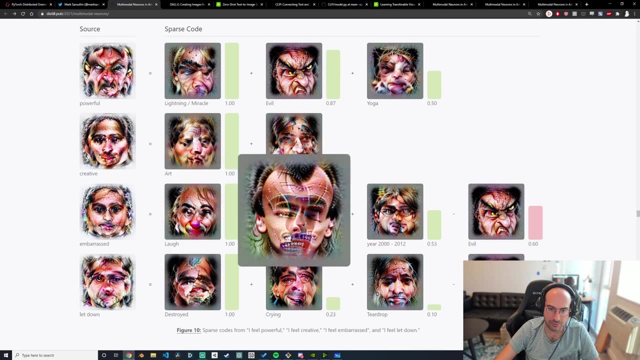 This is a cool image, though Could be a metal cover. So creative is art plus painting. This sounds a bit more reasonable. The painting was very interesting that I figured out. this is paint on a guy's face, So if you take laugh and foreheads- 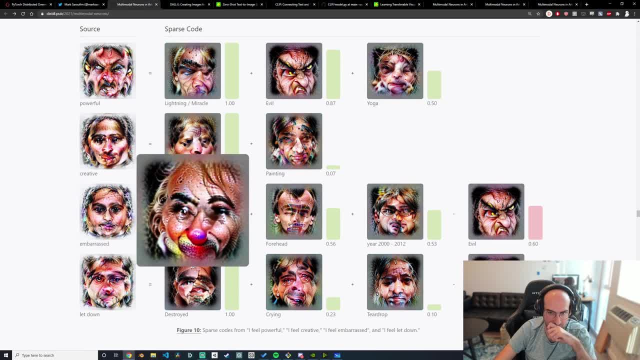 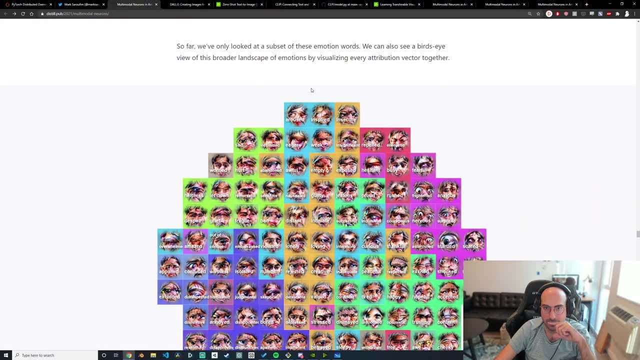 Okay, this guy has a forehead that's showing. Doesn't look like he's laughing. Yeah, I don't know, but Oh, whoa, We can serve up this broader landscape of emotion by looking at like a full vector of it. 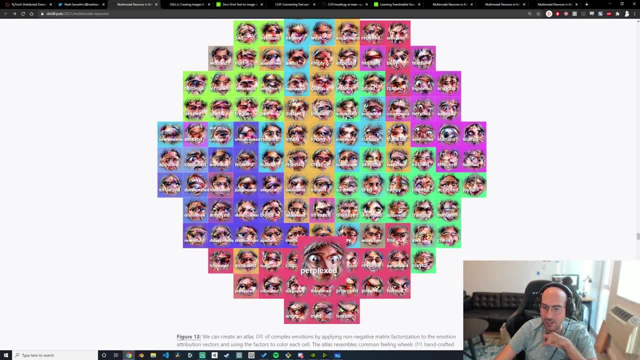 This is kind of nuts actually, Like I can imagine like now for something like a game. this is very interesting because, like you could, you could basically also like have an encoding for some sort of 3D model and then have it be either angry or disapproving. 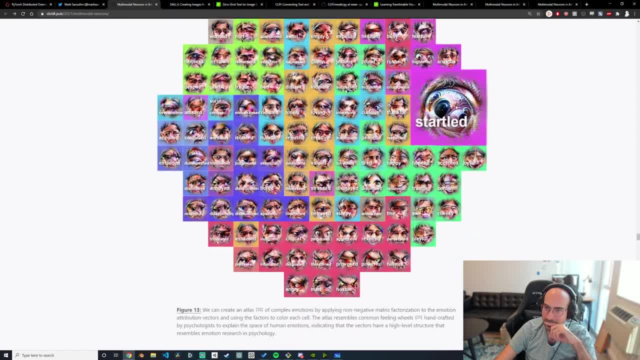 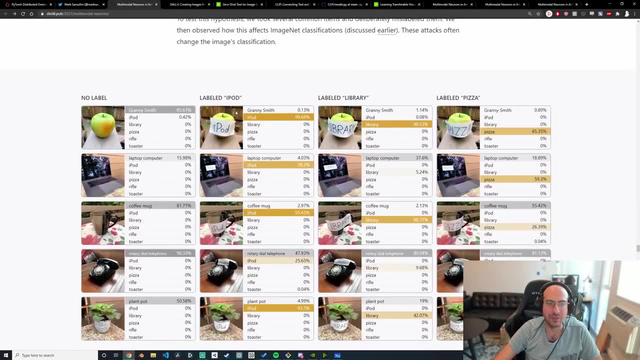 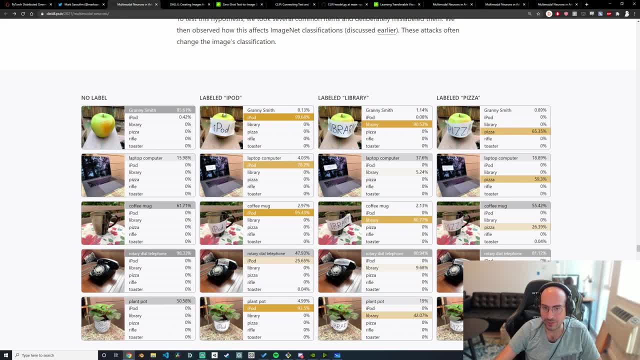 and text be part of the same. you know like both have the representations. like a really simple attack is you just put like a label text that you know this is an iPod and you know all of them say like look, it's an iPod. 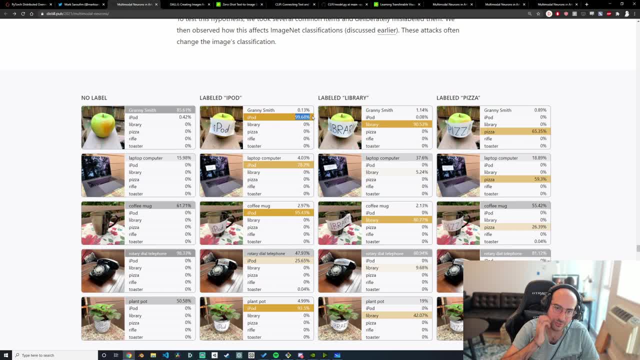 The interesting thing is like, right after that it says it's Granny Smith, but it's just like very confident of this prediction. So it gives you, like I guess, a good way of potentially defeating these attacks, even though, like let's say here: 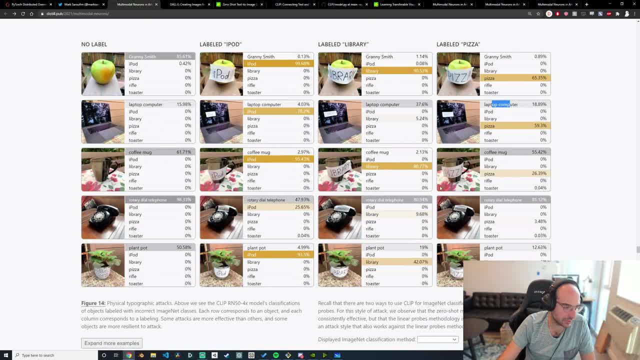 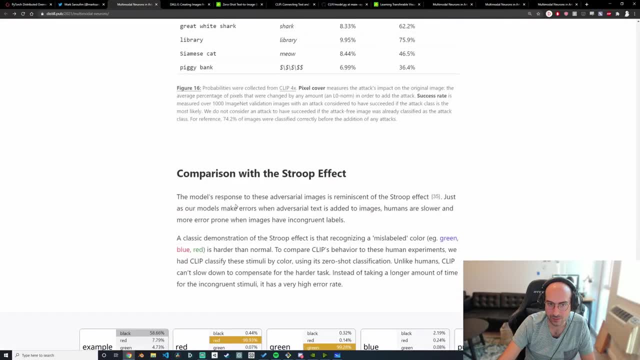 oh yeah, it's saying it's a pizza and then after that it's a laptop computer. So I'm also has a pretty good idea of what the thing is. It just seems to over-prioritize the text. The Stroop effect. 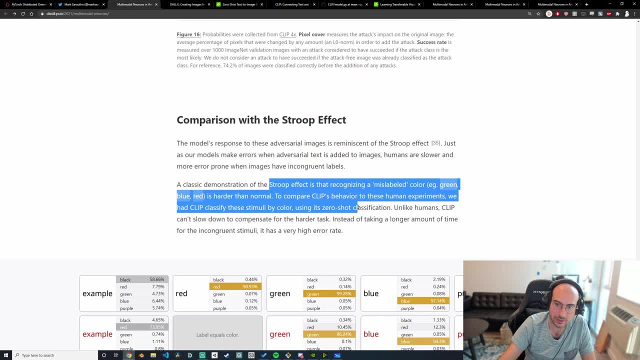 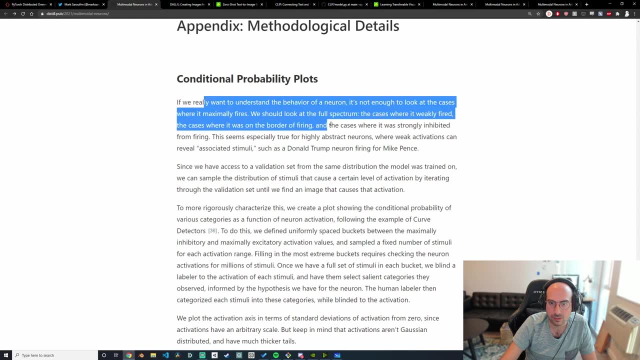 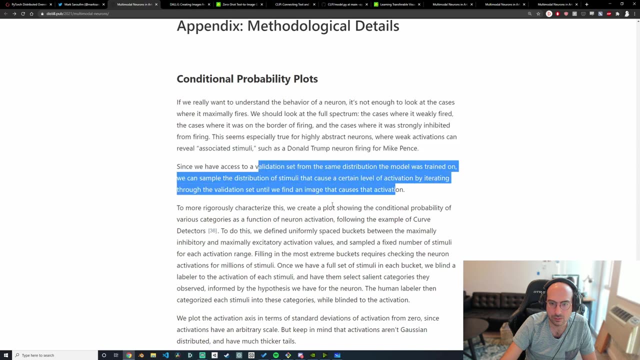 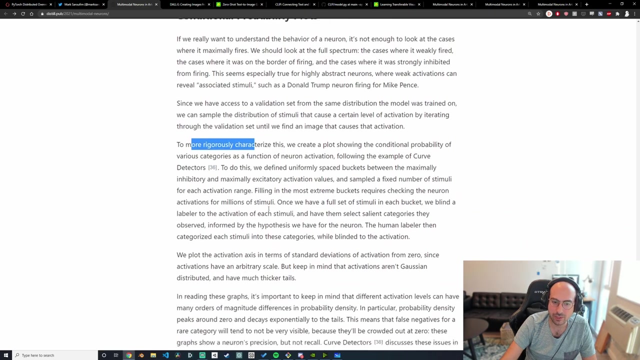 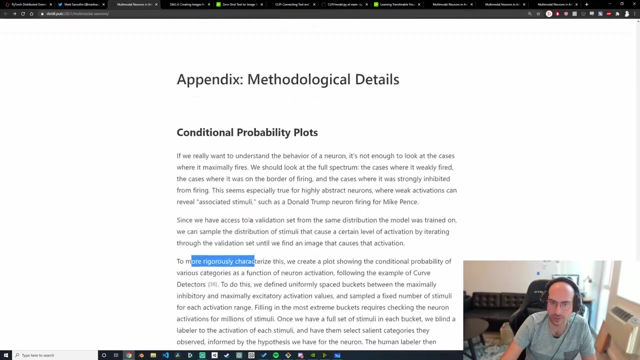 So recognizing a mislabeled color is harder than normal, Okay, Okay. so this is here. they're finally explaining what was up with those activation plots And they explain how this stuff works here. So let's go through this, and I think we'll just do a one final skim. 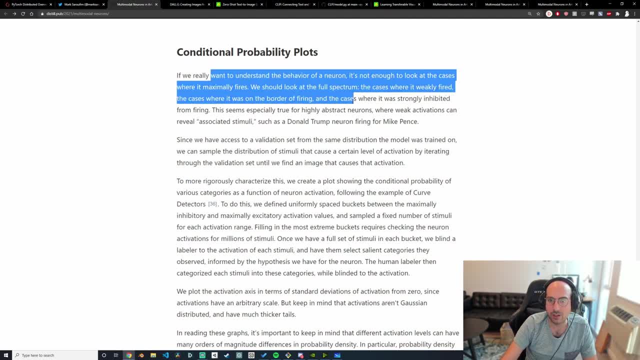 and probably call it So. if you want to understand the behavior of a neuron, it's not enough to look at the cases where it maximally fires. we should look at the full spectrum, The cases where it is weakly fired, where it's on the border of firing. 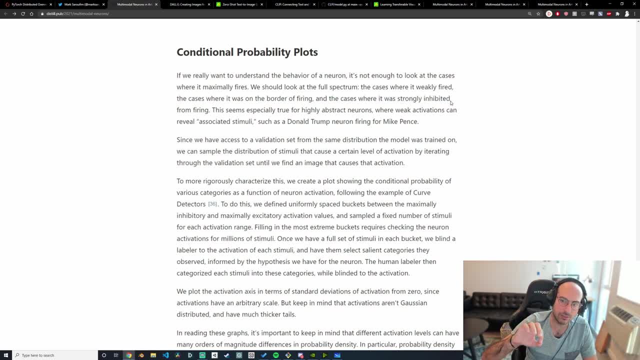 and the cases where it was strongly inhibited. So basically, plot the activation of a single neuron as a function of all the images in the data sets. right, Okay, And so since we have access to a validation set from the same distribution, the model is trained on. 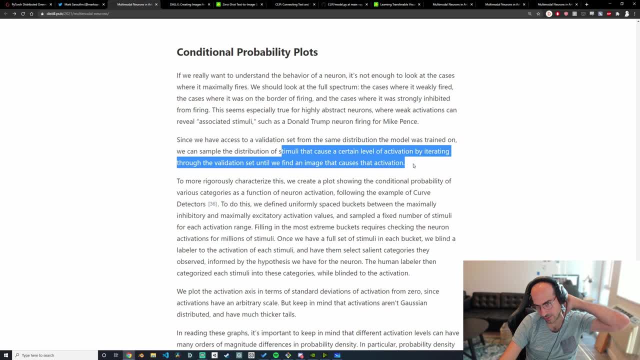 we can sample the distribution of stimuli that causes a certain level of activation By iterating through the validation set that we find an image that causes the activation. Yeah, so this is basically what I was just saying. We define universally spaced buckets to the maximally and minimally inhibitory. 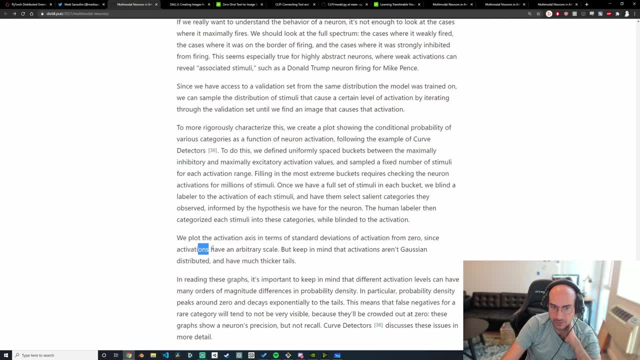 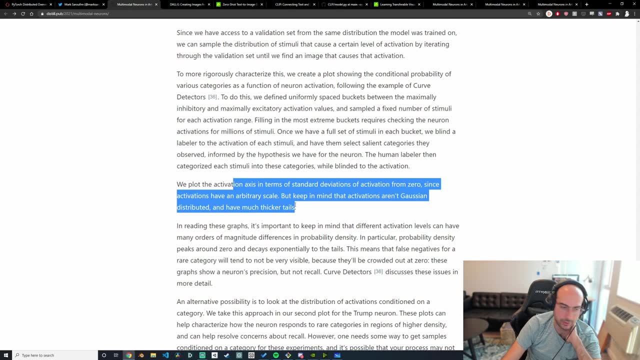 So we plot the activation in terms of standard deviations of activation from zero. Yeah, I think they're also saying: look, these aren't Gaussian distributions because, like I guess, like some, some neurons have power laws. It seems like Trump, the Trump node, for example. 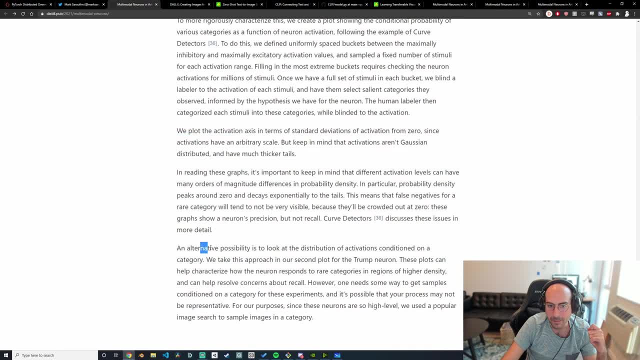 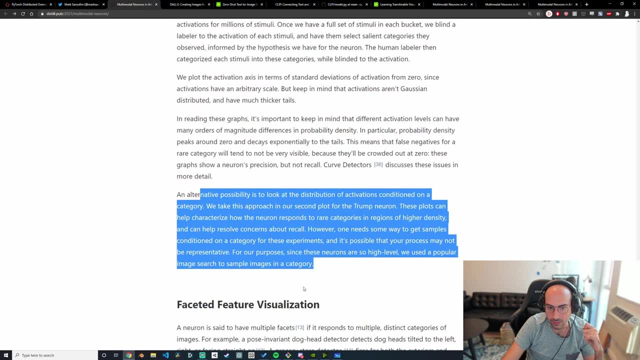 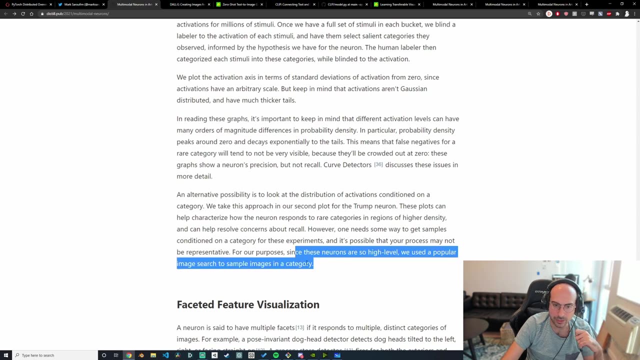 is a highly correlated concept with lots of stuff on the internet. Oh, and it looks like they used an image search tool to sample images in a category. I wonder what that image search tool that they used was. I'd imagine that maybe they use like Google search. 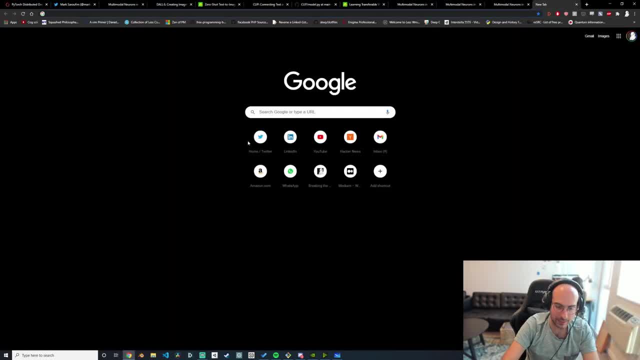 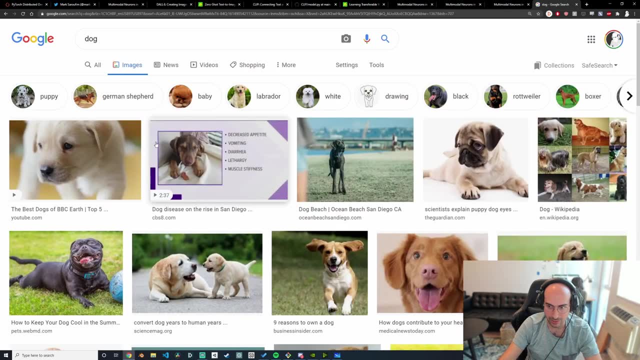 just to come up with the concept Right Like as in. by that I mean like, let's say I say dog like this is. this is a good image search for you know what a dog could look like. 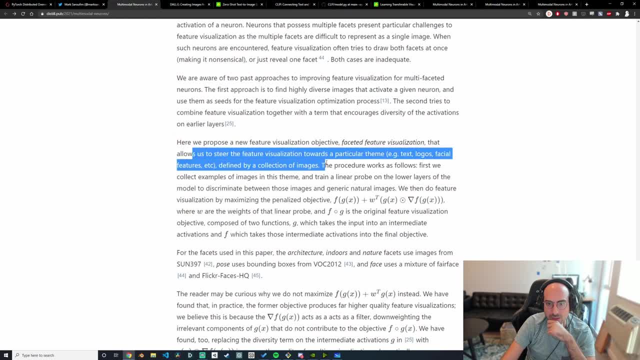 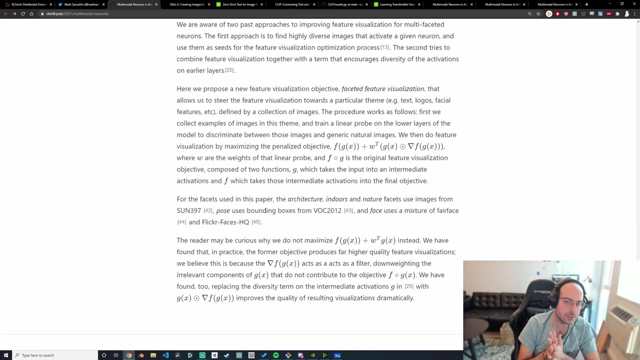 Okay, Facet feature visualization Between a linear probe on the lower layers of the model to discriminate between those images and natural images. Okay, so I think this is where the contrastive part comes in, From the facets and doors. Oh, interesting. 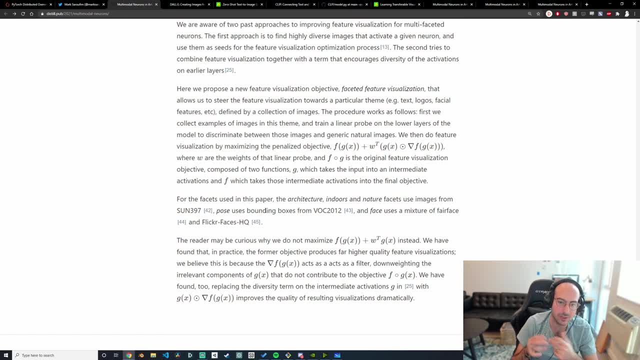 Yes, so it literally looks like they used like existing data sets for like: okay, these are rooms, So that's how they can. why do we not maximize this thing instead? I mean, that's sort of a different concept, Like, for example: 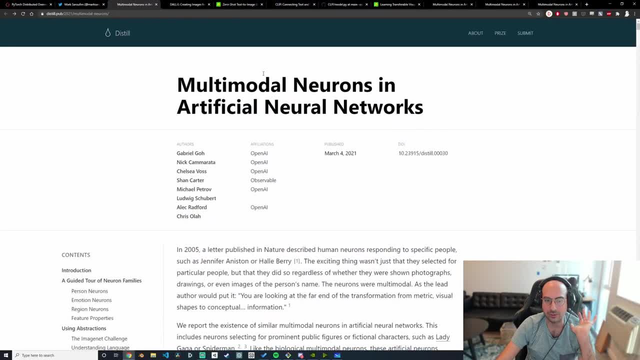 I think that's what it must be. I don't know if this is a bit more complicated or something. I'm just kidding, I'm just you know, I don't know. I think it would probably be if it was a multi-modal model. 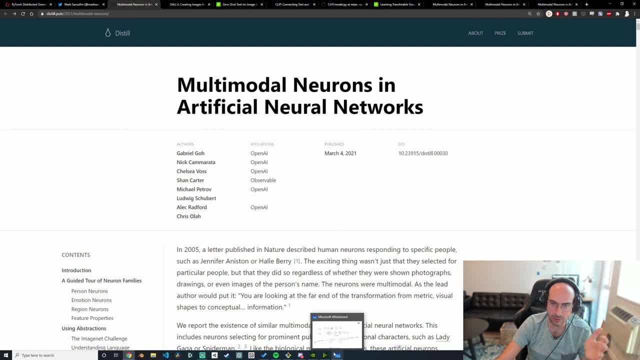 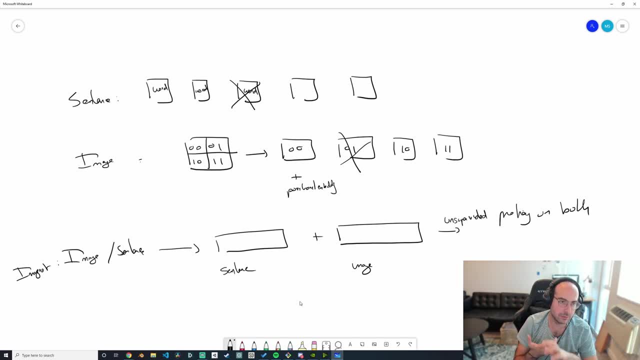 I don't know why it doesn't have all these different dimensions. Yeah, I don't know, I don't know. Yeah, Yeah, Yeahildcom, the fact that we can combine the main idea of BERT for both sentences and images. 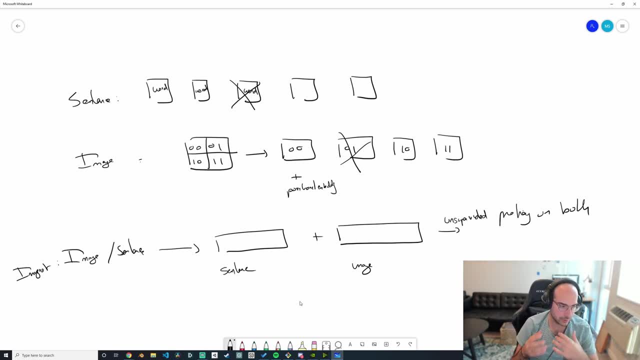 and create like encodings for them, And once we have encodings for each, we can combine them and then we can use this as a pre-training step and then use this to solve some sort of like end level task, If you're doing this on with clip, for example. 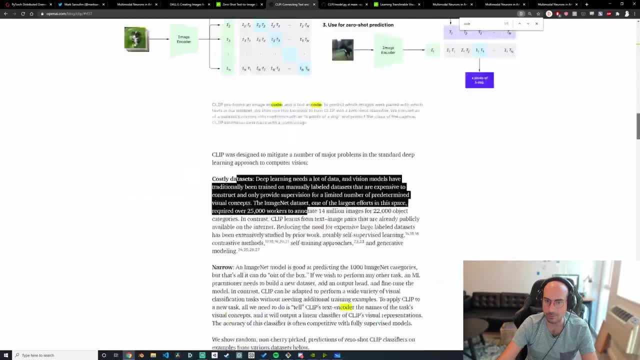 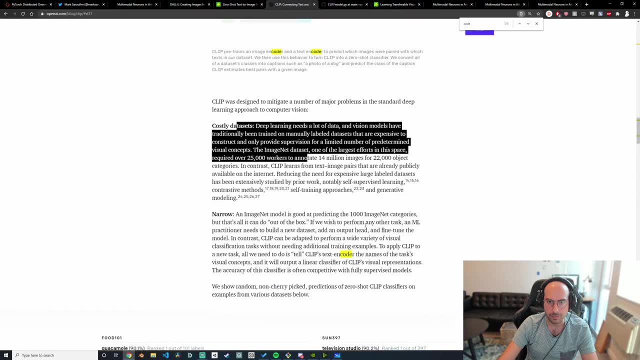 it tends to be pretty good. It seems to outperform ImageNet at a fraction of the flops, like actually more efficient to train than ResNet, which is very surprising. but just something to keep in mind, And specifically with DALI as well. 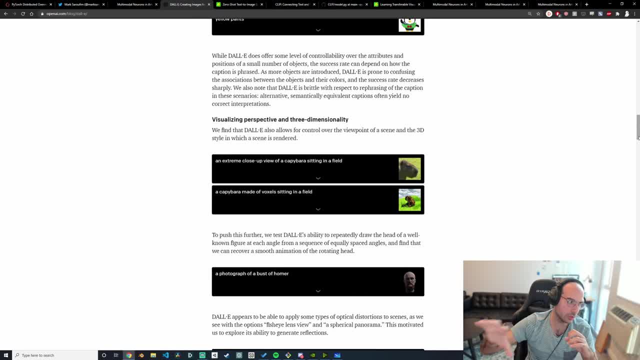 given that you can. generally in any sort of neural network, you can change the last layer, like whether you want this to be a classification or regression or a generative task. you just plop on something in the end and you can solve different tasks. 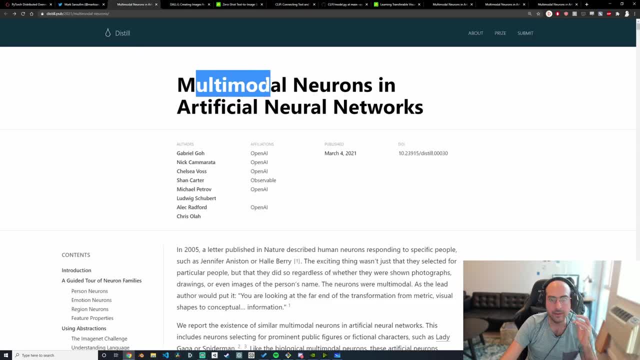 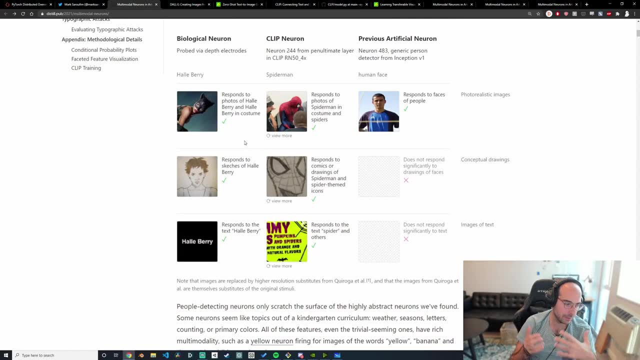 And specifically when trying to understand, like: why do these things work really well? this multimodal neuron works? realize, like: recognizes that some neurons respond to concepts and that clip may be doing well because it is learning to recognize these concepts And to specifically prove it. 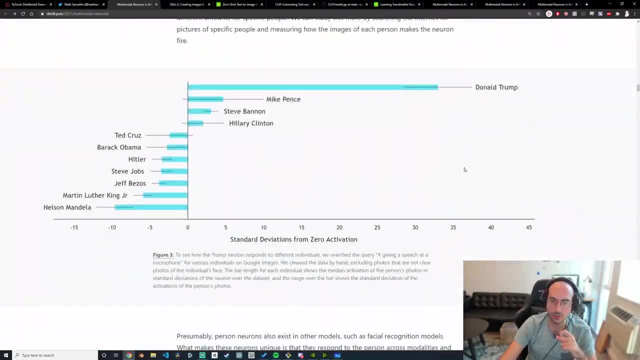 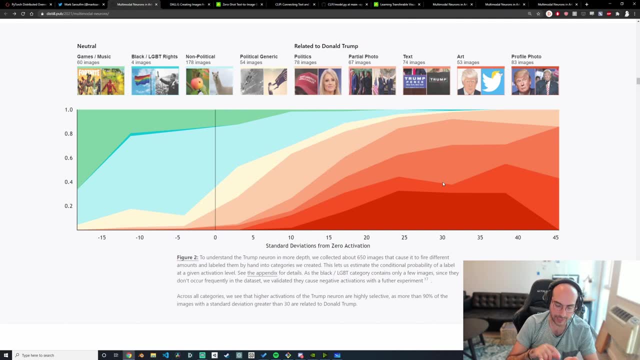 what they do is that they plot. they essentially use these distribution plots. where is it here? Where they look at the conditional distribution of an activation of a specific neuron with respect to all of the images related to that concept in a dataset. So you do this plot. 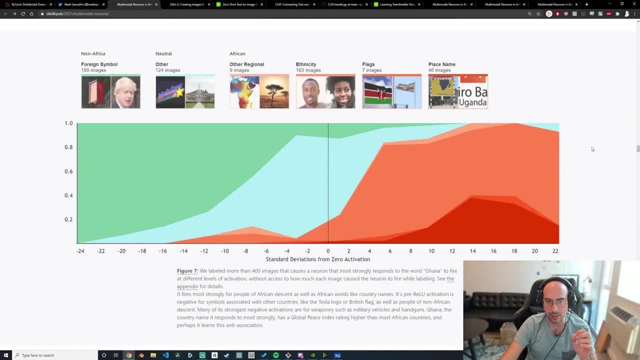 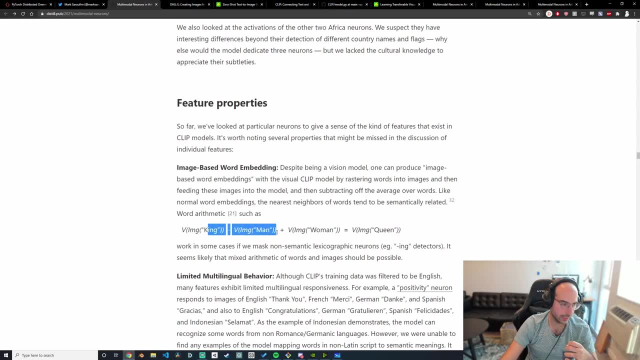 and then you can get a pretty good idea of what's going on. So after you do this plot, you can come in here and there's a bunch of other stuff. you can study One instead of just looking at traditional word: embedding arithmetic. 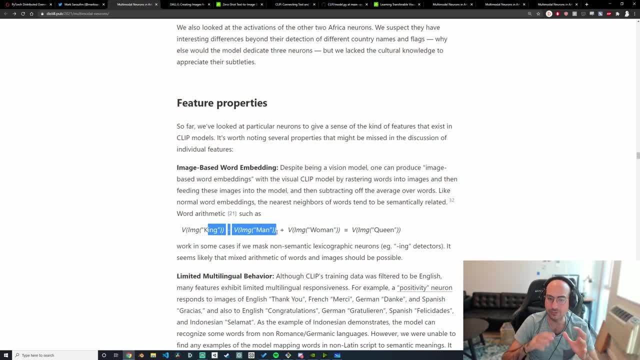 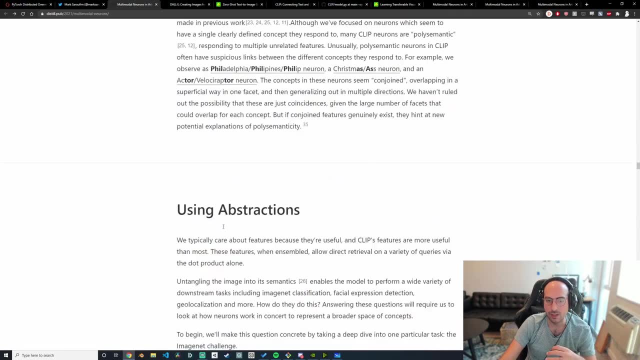 you can also look at image embeddings to have concepts of images, right? So let's say an image of a king, and then you can do this arithmetic here. What else I thought was really interesting is this part right here, which is that in clip. 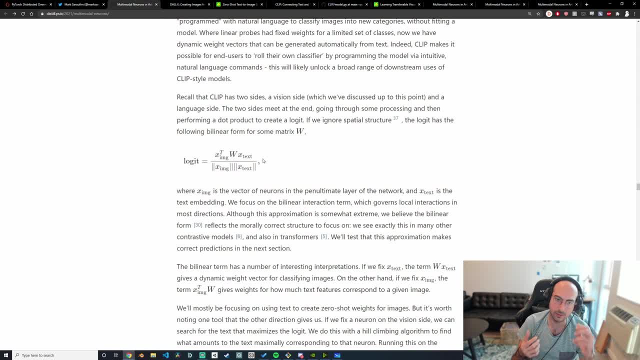 there's sort of two sides, right. So when you're actually making a prediction, at the very end you have your weight, so like the weights of your model, but you also have like an embedding for your image and your embedding for your text. 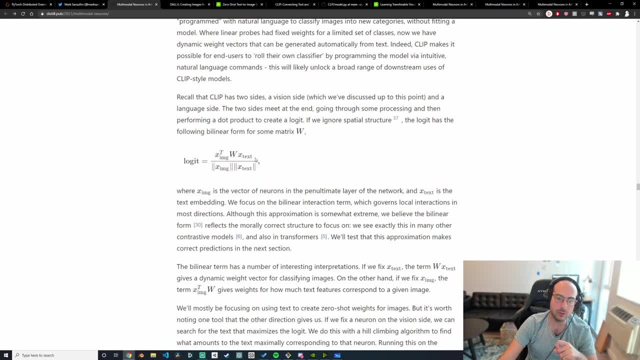 If you fix either one of them, what you can then do is you can find what maximally activates either the image or the text, And so this becomes like a good way to do a form of image search. So yeah, I think this was the end. 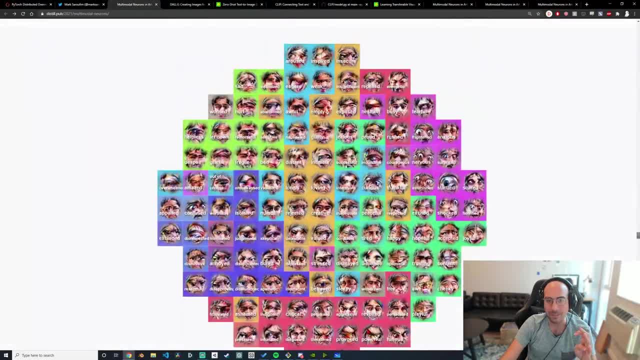 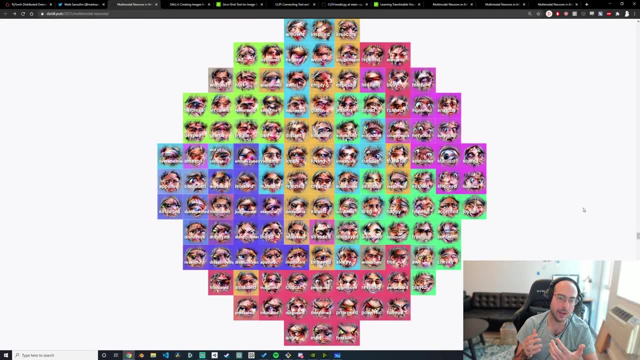 And this part I don't know like I didn't fully understand this part, but this part I actually really, I actually really thought was very interesting, Like the fact that we can create like a spectrum of emotions and then maybe even combine this. 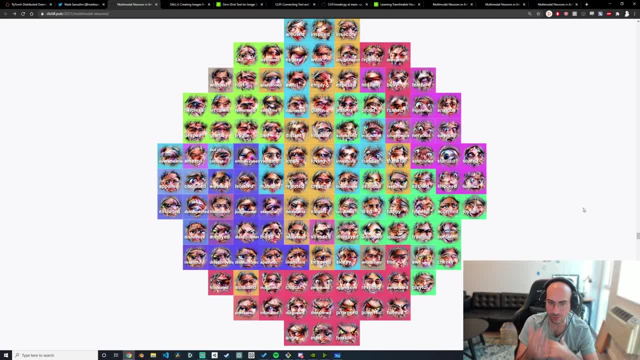 with some stuff in 3D modeling and that way generate emotions for different people in a almost like an unsupervised way. right Cause this was: you don't need labeled data to say like: I want you to look like this, or it's probably simpler ways of doing it.